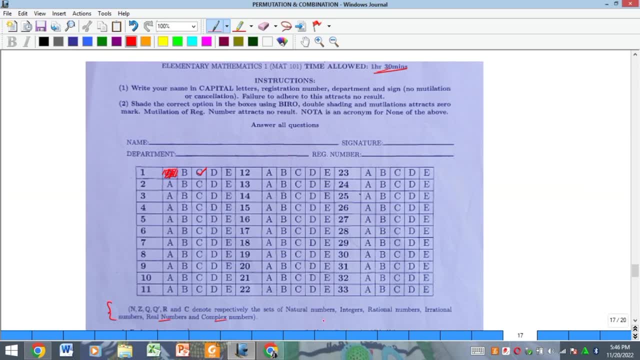 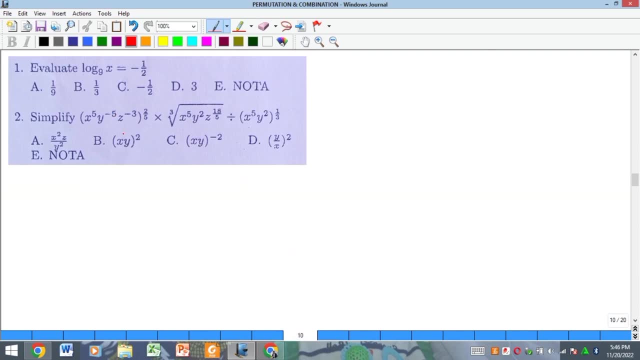 that Okay, so we begin with the first, the beginning part of the exam, which is the number 1.. The number 1 here is from logarithm and it says that we should evaluate log 9,- sorry, log x- base 9 equal to minus half. So what do we do? We simply solve this following the definition. 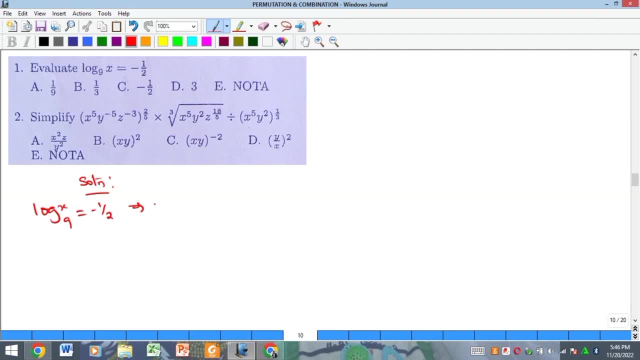 of logarithm And that definition says that that if I raise the base by half, then I will have the base of a logarithm equal to the value of the logarithm, that it is equal to the number. This is the number, this is the base and this is the value. So that means 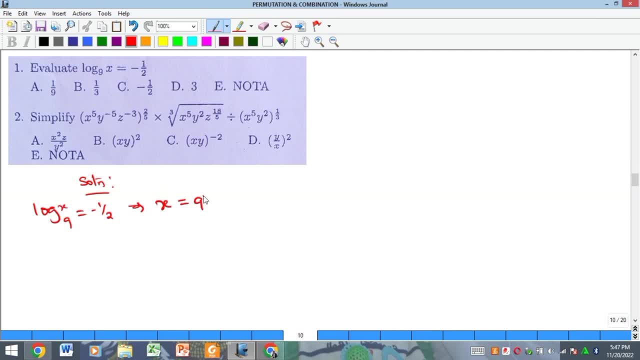 my x is equal to 9 raised to the power of minus half, And of course this is the same thing as by indices. This is going to give me 1 all over 9 raised to the power of half, which is equal to 1 all over. of course, power half means square root of 9. And that is equal. 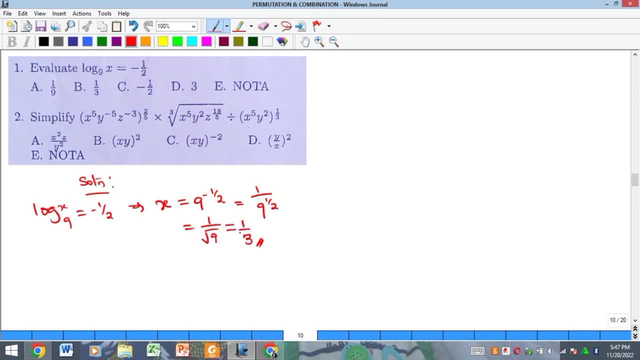 to 1 all over 3.. And you can see here now that our solution for number 1 is B. Okay, so quickly we go to example 2.. Number 2 says that we should simplify this, So I'm going to quickly start the simplification. You recall that when everything in brackets is raised, 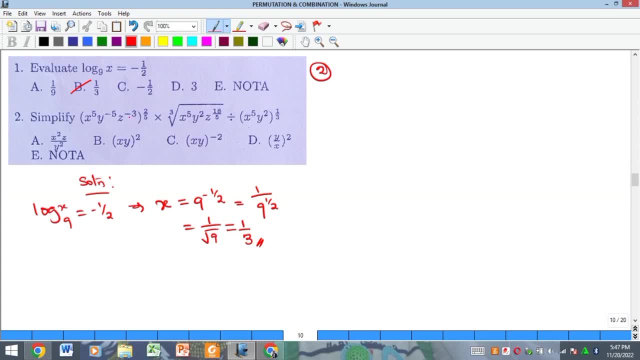 to this power. that means this power is going to multiply all the powers of each of the terms inside the bracket. So if 2 over 5 multiplies 5, of course we will multiply this power by the power of 5.. 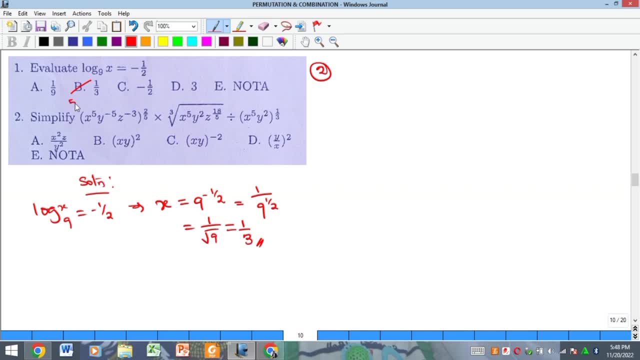 Okay, So we should have the power of 5 x 2 of x. This is the power of x, the power of x squared course. what will happen is that 5 will cancel 5, so you only have 2 left, so the x there is going to. 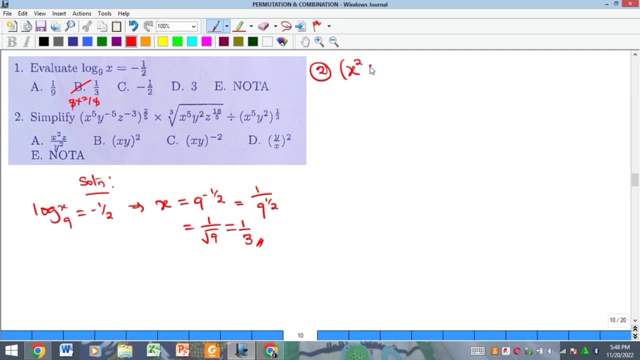 be power 2 and then the y is going to be the 5 here will cancel the 5, and so you have minus 2 left and then you have z. the z power is minus 3. multiplied by this, that will give you minus 6 all. 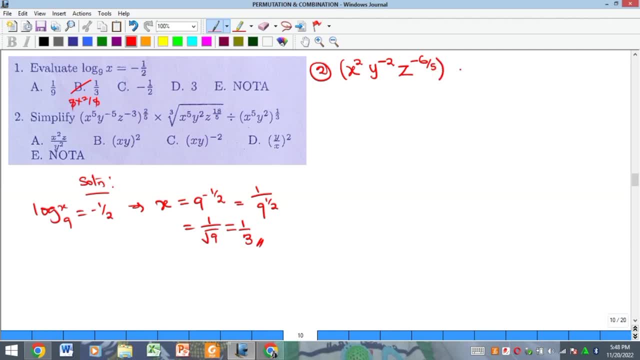 over 5. okay then, this is times. now remember that root means power of a fraction. that means this is the same thing as x raised to the power of 5, multiplied by y raised to the power of 2, z raised to the power of 18, all over 5. and then now cube. root here means 1, all raised to the power of 1. 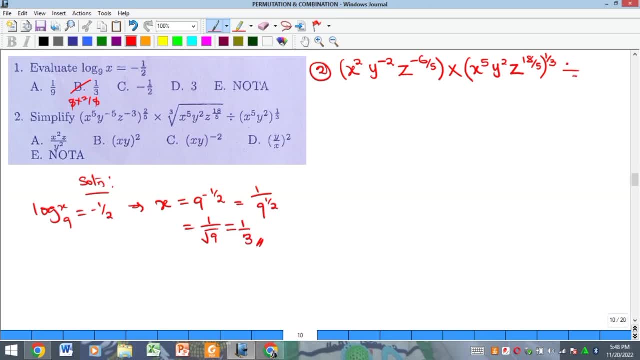 over 3 and this is divided by. we can also open this bracket, and when we do that, we will have x to the power of 5, all over 3. that's 1 over 3 multiplying 5, and then we now have 5 raised to the power of 2 over 3. sorry, y raised to the power of 2 over 3. 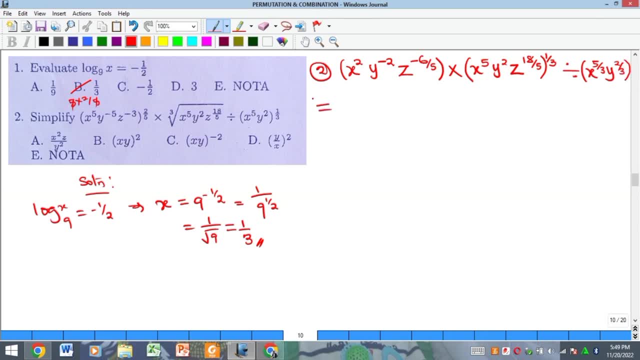 and this is going to give us, of course, this is the same thing, so we'll just simplify this a little bit, you know. so we are going to have x to the power of 2, y to the power of minus 2, z to the power of minus 6 over 5, and this is multiplied by. if this now comes into the bracket, 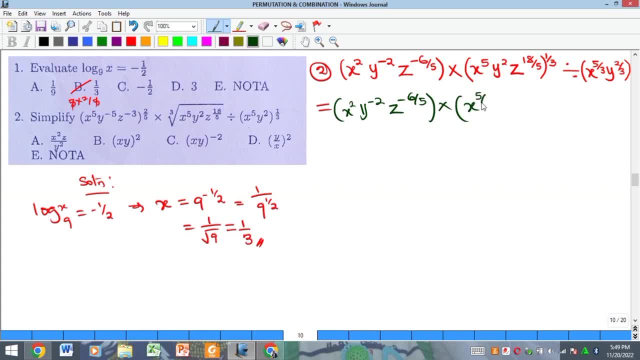 you will have x raised to the power of 5 over 3 times 2 raised to the power of 2 over 3 times z raised to the power of. if this 1 over 3 multiplies, this, d3 will cancel this 18, so you will have 6. 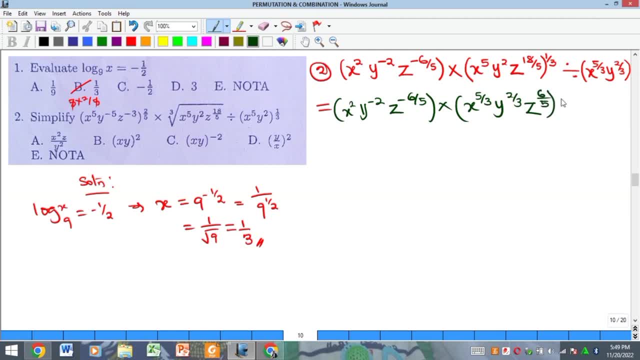 over 5 left there, and this is divided by x, raised to the power of 5 over 3, multiplied by 2 over 3. okay, so i am going to apply the law of indices here now, which says that multiplication of the same base is the same thing as summation of the powers and then division. 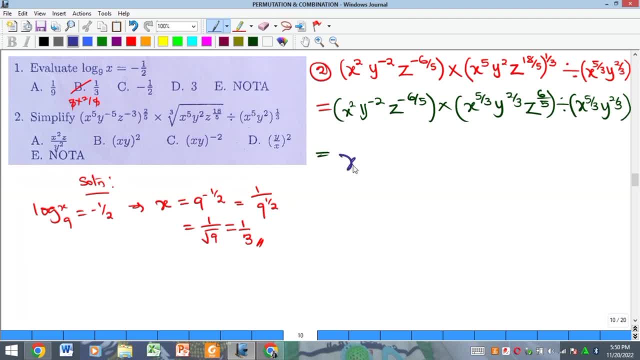 is subtraction. so i'm going to pick x now and then the powers of x. i'm going to add for multiplication and then subtract for division. so i'm going to have 2 plus the power here is 5 over 3, and then the power here is also 5 over 3, but in this case it will be subtraction, since what i 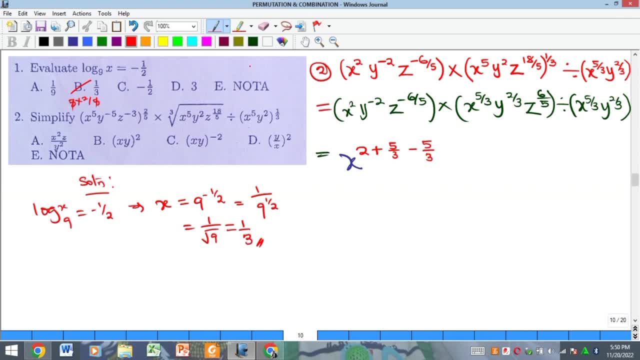 have. there is division and that will be times y to the power of. the power in the first bracket is minus 2 plus the power in the second bracket is 2 over 3 minus the power in the third bracket is 2 over 3. and then i have finally z to the power of in the first bracket, it is equal to. 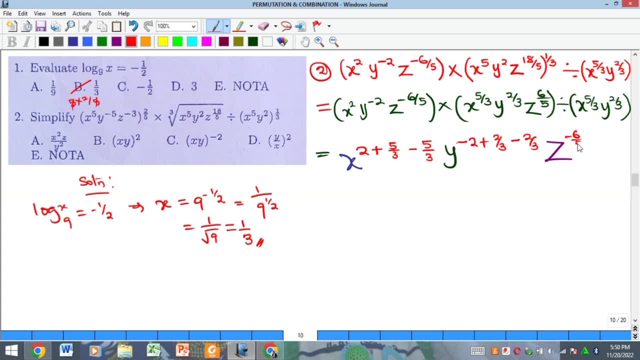 minus 6 over 5, and that is plus. in the second bracket is positive 6 over 5, and so this is going to now give us that, of course, this will take away this and this will take away this, so you just have x squared, y raised to the power of minus 2. this will also take away this, so you just have z raised. 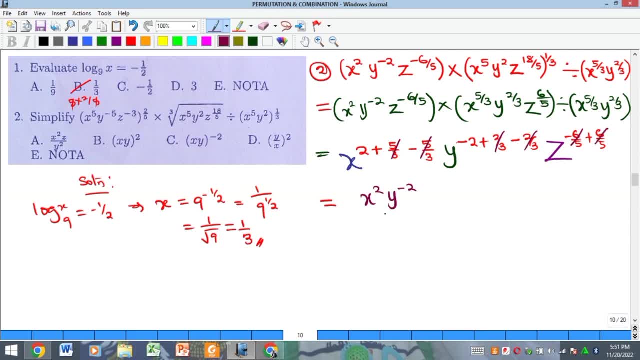 to power 0, which is actually equal to 1. so this is our solution, which we can also write as x squared over y squared by indices, this will become 1 all over y squared, and we can quickly write this as x all over y all squared. and, of course, if you check in the option, there is no option there. this is what. 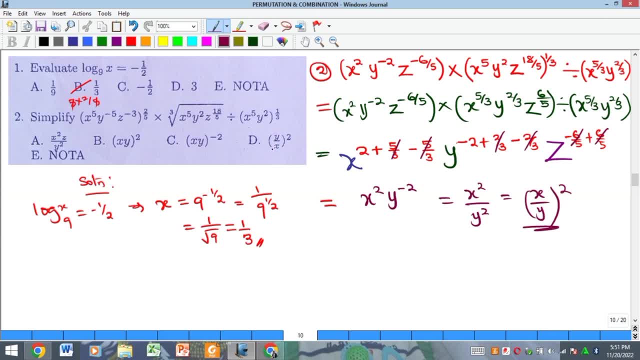 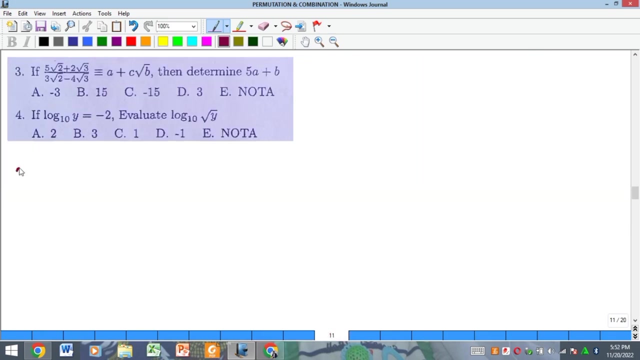 wanted to look like it, but please note, it is wrong to choose nota- nota means sorry- is wrong to choose a solution that is close to what you are supposed to have. so when it is not in the option, please always take your e, which is: nota is none of the above. okay, so we go to the next one here. example three: we have, uh, sorry question. 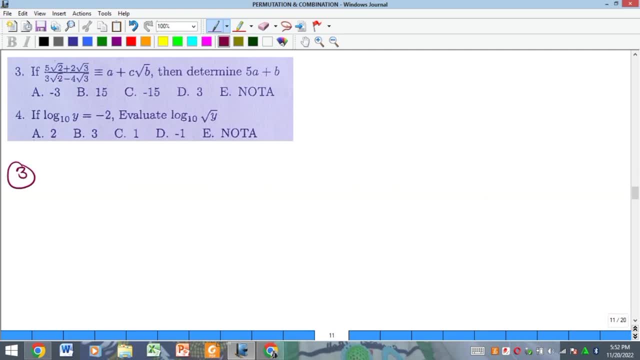 three. we have that. we should put this in this form and then evaluate this, and so to do that, i am going to rationalize the sort. this is from sort, so i have 3 root 2 minus 4 root 3, so i'm going to multiply by the conjugate of the. 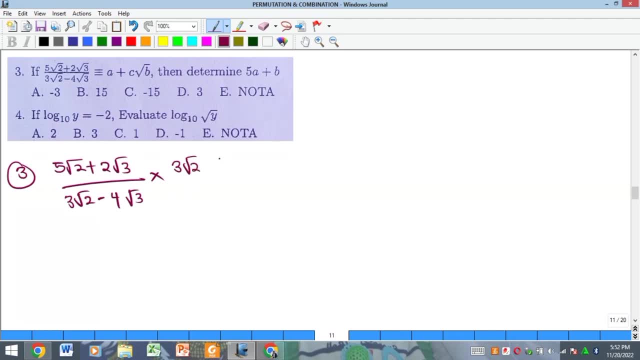 denominator, which is just to change this to plus, and this will give me plus root 3, all over 3 root 2, minus sorry. plus 4 root 3. okay, so when you do this multiplication you are going to have, of course, this will multiply these two and this will do the same. so 5 root 2 times 3 root 2 will give us 15. 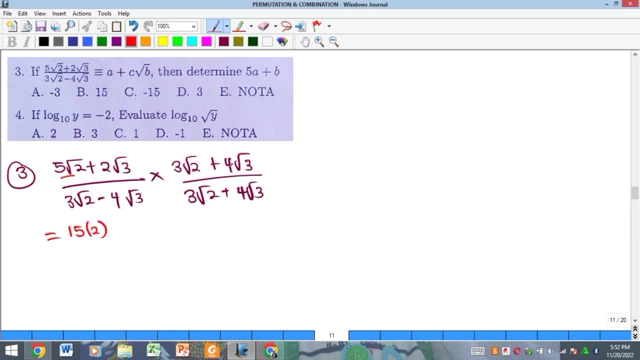 times 2.. 5 root 2 times this will give us 20 root 6, and we are done with that. so we go to this other one: 2 root 3 times 3. root 2 will give us 6 root 6, and then, this times, this will now give us 8 times 3. 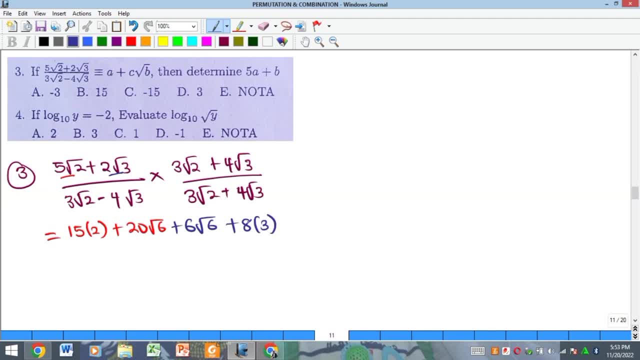 excuse me, your name is hello. hello name is, loss with your name is. so this is all over, of course, recall how to do this. the denominator, since they are conjugate. just use this and multiply this and that's going to give us 9 times 2, and then. 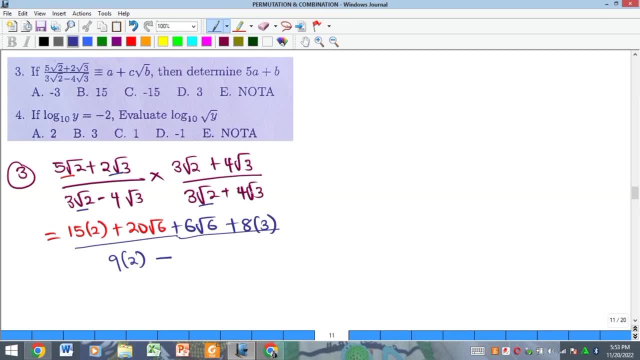 minus. then just use this and multiply this, which is 16 multiplied by 3, and of course this is going to give us, um, this is 30 plus 18, which is 48, and then this is 20 plus 6, which is 26 root 6. 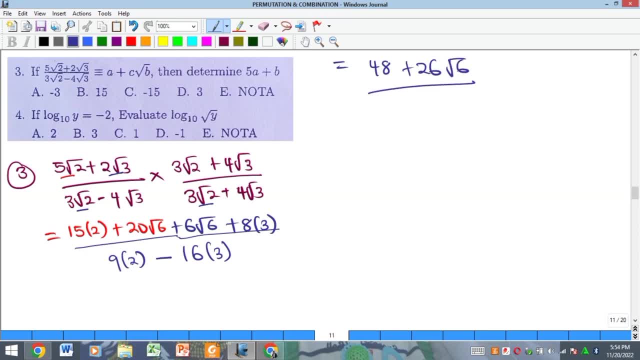 all over this is 18 minus 48, and that's going to give us minus 30. so, of course, if you split this, we are going to have minus 40 all over 30, and that is minus 26 over 30. 30 roots 6, and so they asked us. we have put it in this form, so this is our a, the whole of this. 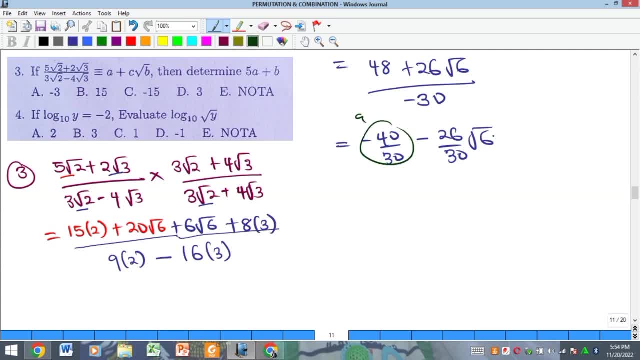 is our a and then our c. sorry, our b is what is under the root, which is 6, and they're asking us to find 5 a plus b, meaning we should multiply our a by 5, which is minus 40 over 30, and then we should. 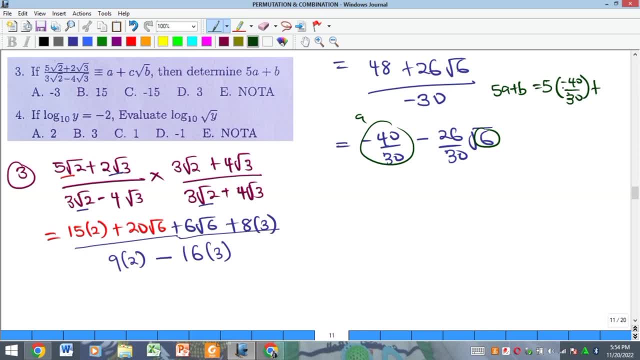 add b to it and our b is 6. so if this multiplies this, of course this will cancel, to give you 5. sorry, this is 48, this is 48, okay, and of course, if this cancels this, we are going to have 6 here. 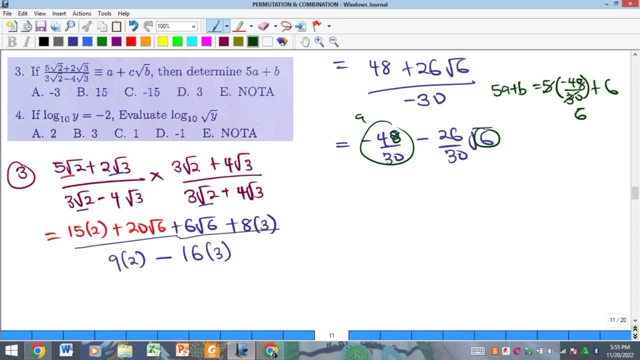 so, and this place is 48, 6, we divide 48 to give us minus 8 plus 6, and this is equal to negative 3, which is option b. so for a number 4 here, what are we? the same definition. so we have log y, base 10 to be equal. 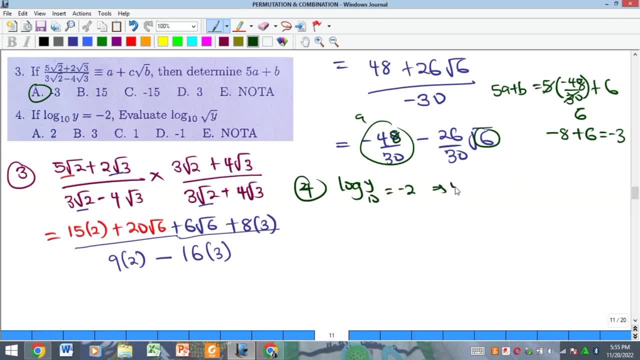 to negative 2. this means that y alone is equal to 10 raised to the power of minus 2. and then they asked us to evaluate this, just substitute into that. so i'm going to substitute my y now, and so i have square root of 10 raised to the power of minus 2, base 10 and of course square root is the. 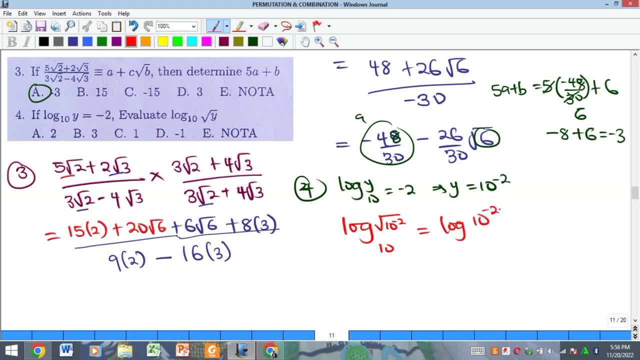 same thing as power half, so i'll have this times half. so this will take away this and this is base 10. so this will give me log 10 raised to the power, minus 1 base 10. of course this one will come to the back to give, sorry, minus 1, to give me minus 1 log 10, base 10, which is equal to 1, and then 1. 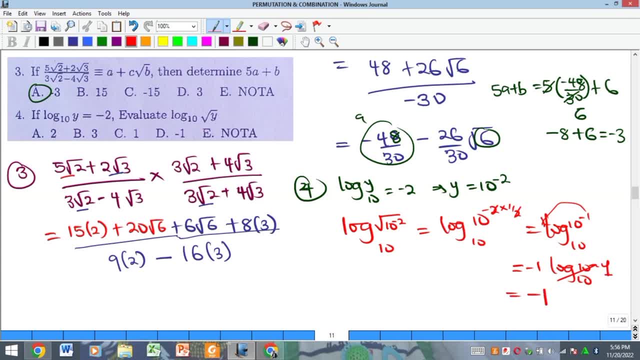 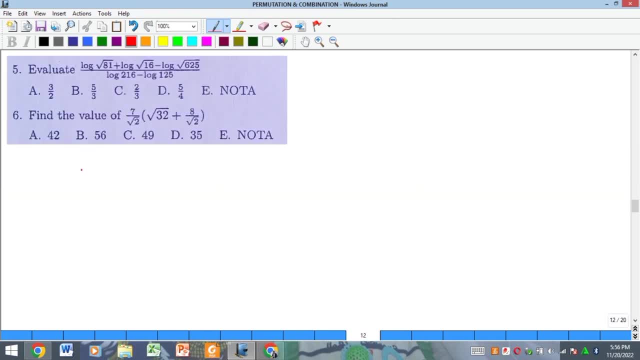 times minus 1 is equal to minus 1, and so your d is the correct option for number 4. so number 5 here asks us to quickly evaluate this. and so what do you do now? of course, we know that log root of 81 is 9 plus and root of 16 is 4 minus. root of 6 to 5 is also a perfect square root, and 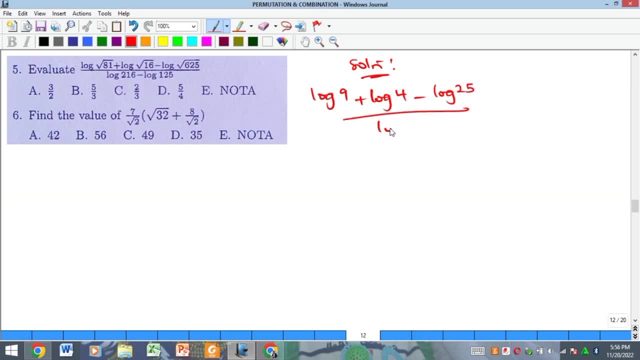 and this is divided by. remember that here we have the 2 1 6 can actually become 2 1, 6. all over 1 2. 5, because subtraction in logarithm changes to division. so this is that i'm going to give up. we will do the same thing up here for 9 times. 4, because addition changes to multiplication. 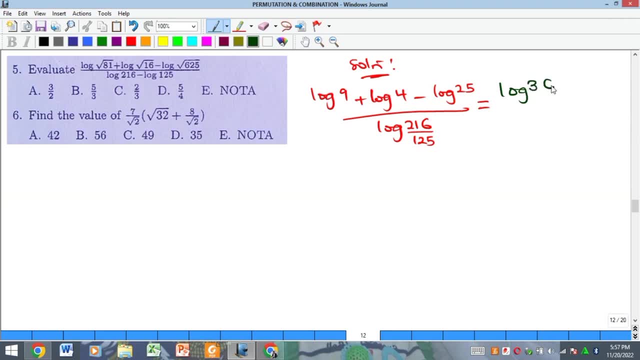 so we'll have 36 all over 25 here, and then everything is all over this: 2 1 6 over 1, 2 5. and now what do i do from here? i can see that i can actually. all of these are perfect squares. 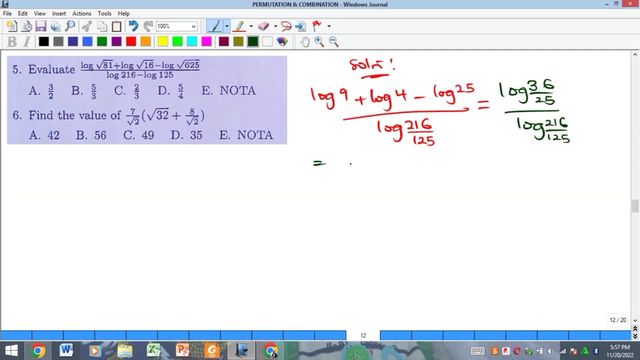 why these are perfect squares? because i can actually do this and i can actually do this, so this can actually give me log 6 squared all over. let me do it this way: log 6 over 5 all squared. of course, if you open this bracket, you will get back your 36 over 25. 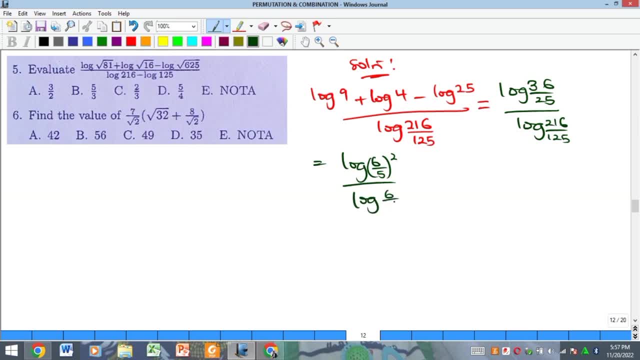 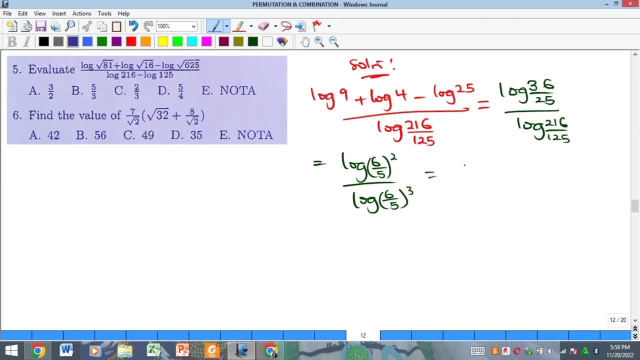 bring the 2 to the back, bring the 3 to the back. so you have 2 log 6 over 5, all over 3 log 6 over 5. so here you have the same value. so i can quickly take away 6 this logarithm. so my answer is 2 all. 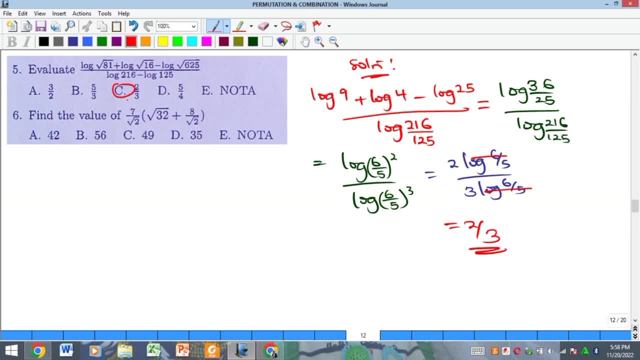 over 3, and that is option c. so we quickly go to number 6 here. number 6 says that we should evaluate this, so the first thing to do is to open this bracket. if you do that, you will have 7 over root 2. multiply each of the terms in the bracket so we'll have 7 root 32 all over root 2. 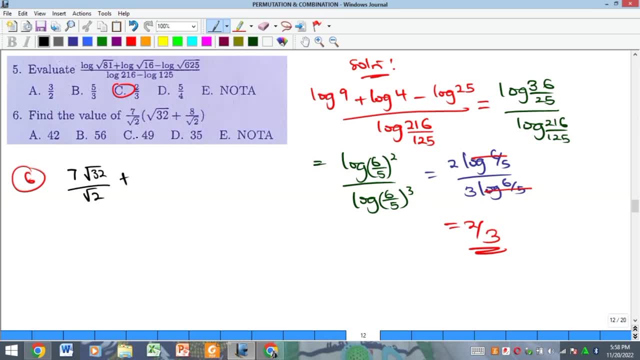 and that is plus 7 times 8 here will give us 56 all over root 2 times root 2 is 2. so of course by rule of sword you know that root a all over root b is the same thing as root a over b. so i'm 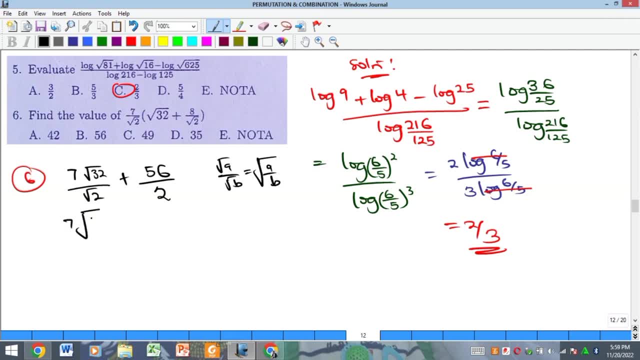 going to open a bracket now, i'm sorry. one root and i'm going to have 32 over 2 and that is plus 56 over 2 is 28. so remember this is multiplication, not a seventh root. so i have this and then 32 over this is 16. so and root 16 is. 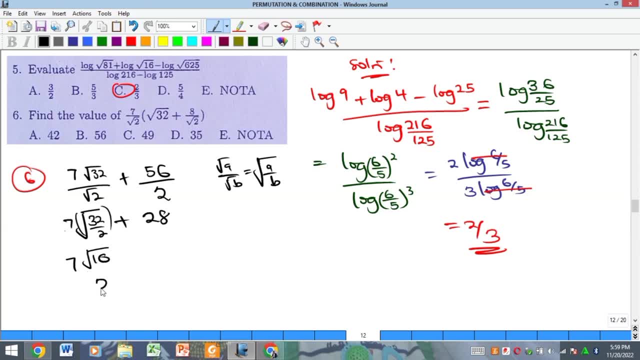 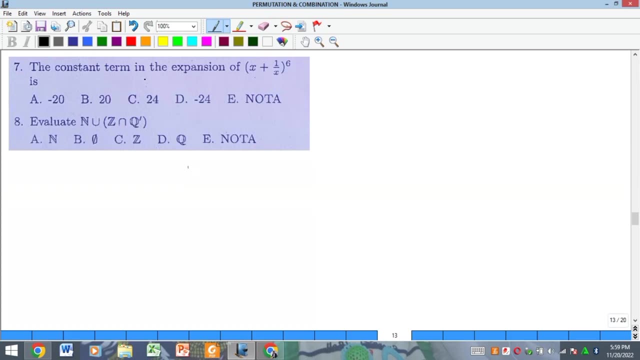 actually 4 times 7 is 28 plus 28, which will give me 56. so remember what i said: you just have to be as fast as possible. so we go to the next one. number 7 says this is from binomial theorem. it says that we should define the 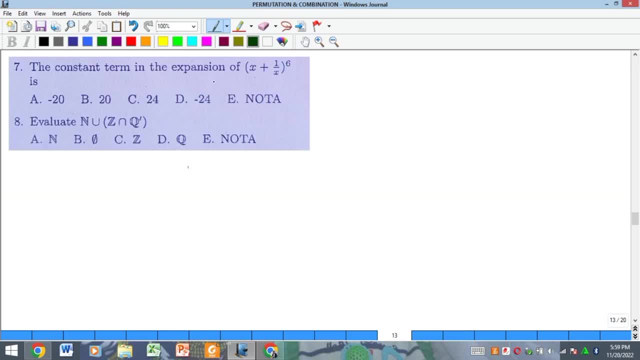 constant term in this expansion. so that means you should expand this and you remember how we do expansion. we either use combination approach or the pascal's triangle. and if we use the pascal's triangle it helps us to get the coefficients. so of course it starts for the power 6, the coefficients. 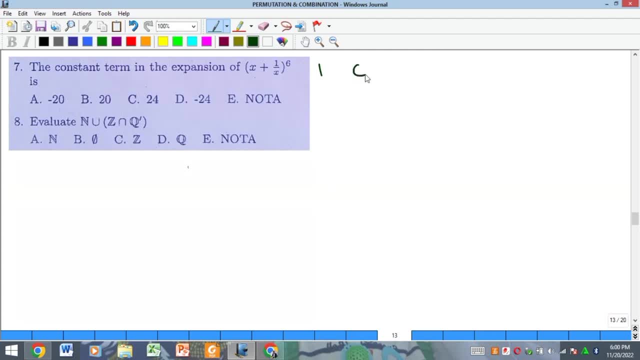 are going to be 5, 6- because of our time, no need showing all of that- 5, 6, 15, sorry. and then we have 20, then 15 again, and then you have 6 again, and then you have 1, and so for each of these coefficients you are not going to. 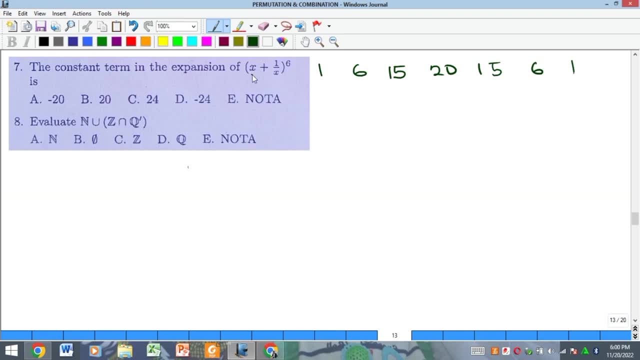 be multiplying each of the term. if you multiply the first term, you sorry, if you bring the first term, you raise it to the highest power. multiply by the second term, raise to the least power, which is zero, and then you keep reducing by one, increasing the second one by one. so that means the first one here is going to be x, raised to power 6. 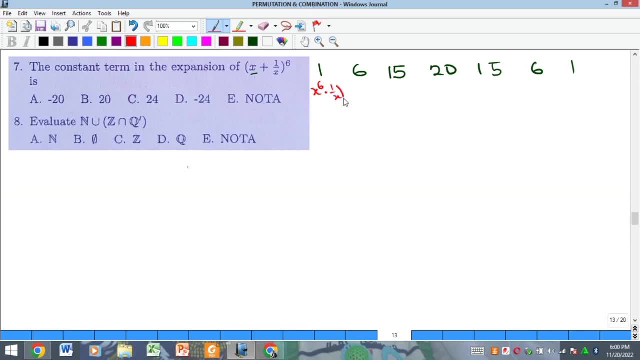 multiplied by 1, all over x raised to the power of 0, which is actually 1. then you will add- remember that the coefficient is 1, which is this. then the next one will be 6 times x raised to the power of 5, then multiplied by 1 over x raised to the power of 1.. now, there is no need to do all of these. 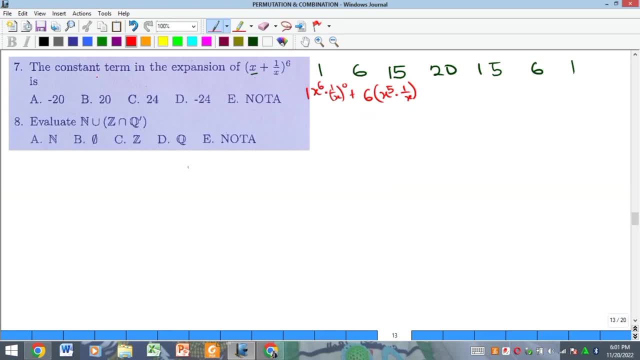 because they just asked us for the constant term, meaning where there will be no x at all, and they for remember that in this expansion you expected to ensure that the sum of the powers you have here must be six. this is six plus zero, which is six five plus. the power here is one which is: 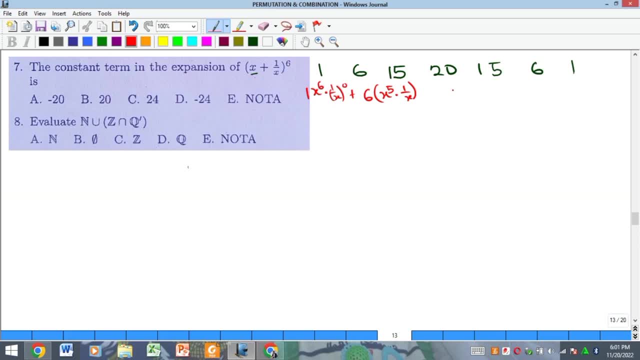 also six. the next one will be four plus two. so which of the two sums that will give us six is able to give us something that can cancel the x? and that is the one for here, and what is it going to be remember? this one is for d, so the next one will be four, two. 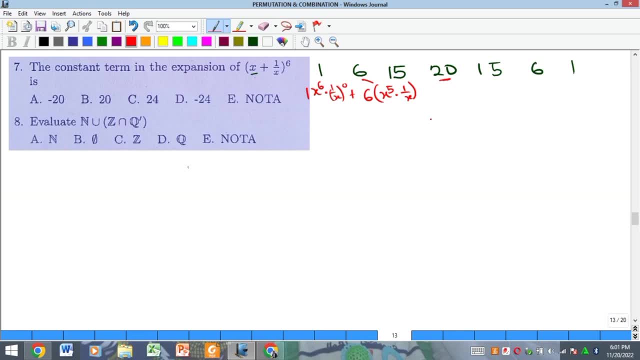 and so the next one is going to be 20 multiplied x will be power 3 multiplied by 1, all over x to the power of 3 also. so the sum of this will give you 6. so the rest is not going to give you. 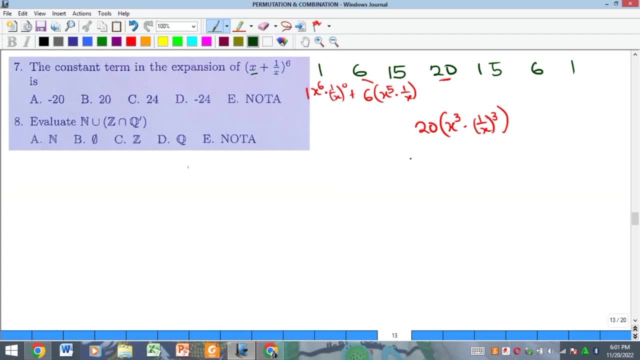 something that will cancel. and how do i mean? if i expand this by indices, i'm going to have s cube times. 1 cube is 1 all over s cube is also s cube. so what happens here is that s cube will cancel s cube. so it is only on the expansion here that that will happen. if you get here, it will become. 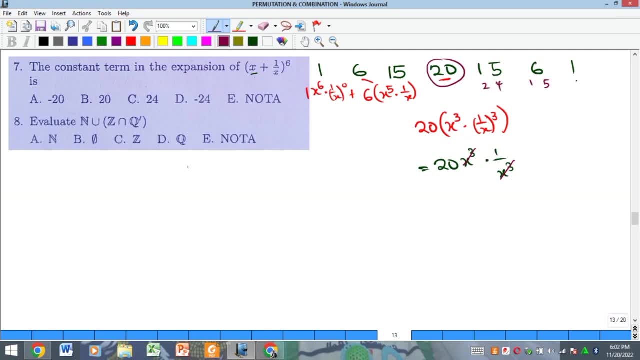 2, 4, this will become 1, 5, this will become 0, 6, so there is no how it can cancel any other place except at this point, and so that means, if i now expand this, finally i have 20. therefore the coefficient is actually 20, which is b. then we go to number 8. here number 8 is actually from types. 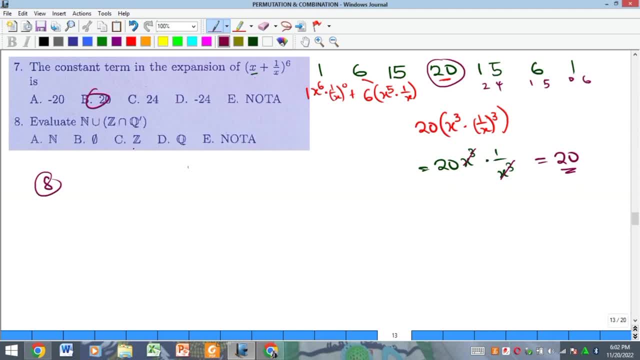 of numbers joined with set theory, and so we know this as natural numbers, integers, and then and then we have this as irrational numbers. so what is the? of course we take the bracket first, so we have the natural numbers: union, union. what is the intersection of z and q? remember, z is contained inside q, that's. 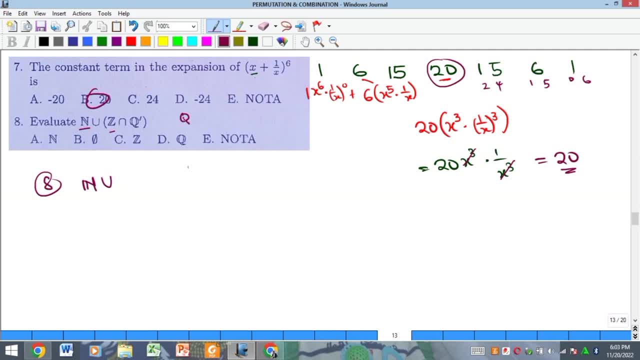 rational numbers that z, q and q prime are completely empty, and so what that means is that the anything that is contained under z cannot be inside q prime, and so their intersection would definitely be an empty set. okay, so when you now take the union of n and the empty set, you will. 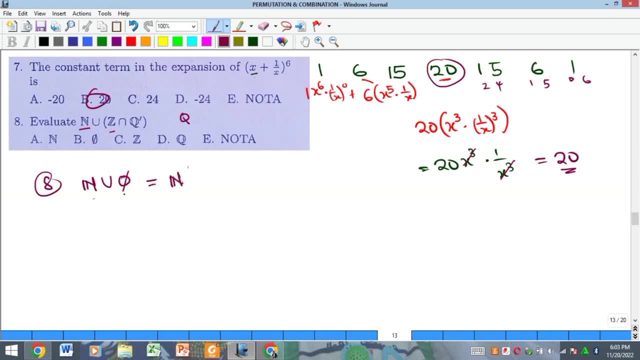 get n remember that how to handle this is that if a set is greater than another and is containing it, then their union will be the greater set. that if a set is smaller than the other and is inside, for example, if a is inside b, then if i 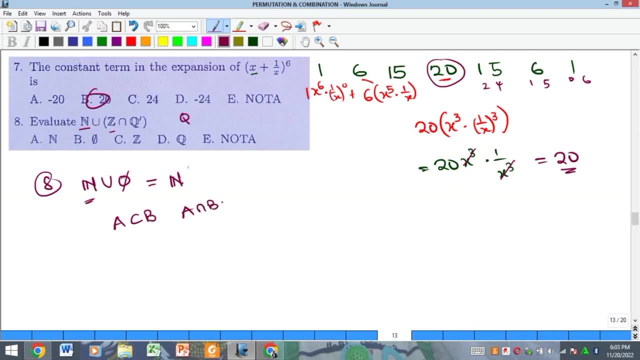 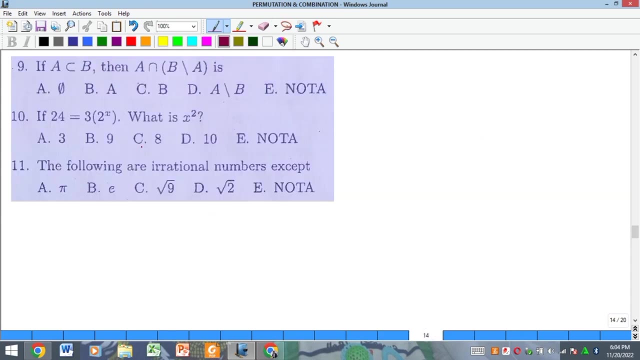 take a, intersection b, i am going to get the smaller set, which is a. if i take the union, i am going to get the bigger set, which is b. all right, and that's how we got our n here, which is option a. so we go to number the next number, which is nine. so the same thing we are going to apply here for number. 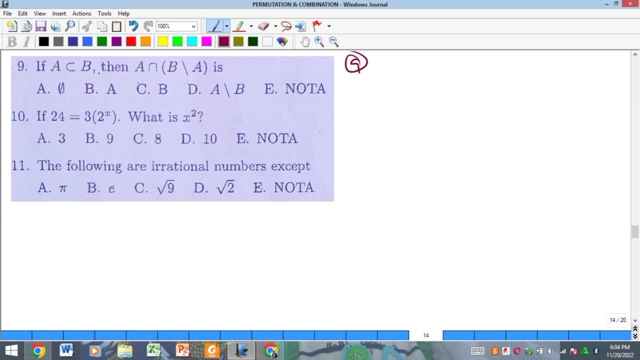 nine here. a is contained in b. so what is this intersection? remember that a slash does backslash a, sorry, b backslash. a means b without a. that means the set of elements in b that are not in a, meaning that the elements of a will not be here at all. so when you take the intersection of a, 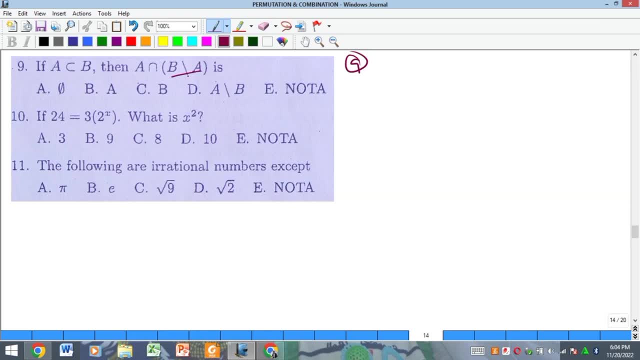 and intersection of a and something that does not contain a at all. the intersection is definitely going to be the empty set, because they don't have anything in common, because all elements here are going to be empty, and so they are going to be empty, and so they are going to be empty. 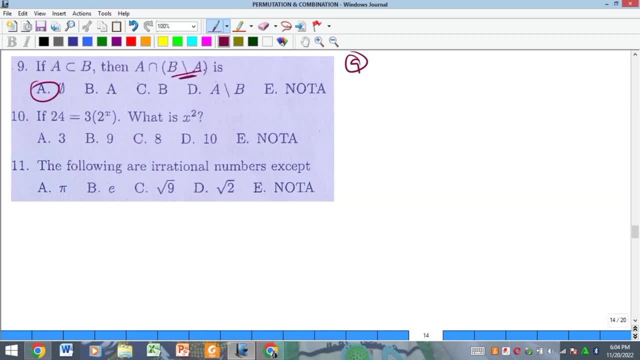 here are only found in b, they are not found in a, and so we go to number 10 quickly. so here, what do we do? we divide both sides by three. if you divide here by three, you get eight, so that you can clear this three here, and then you divide that side, you'll get two raised to power x. so by indices. 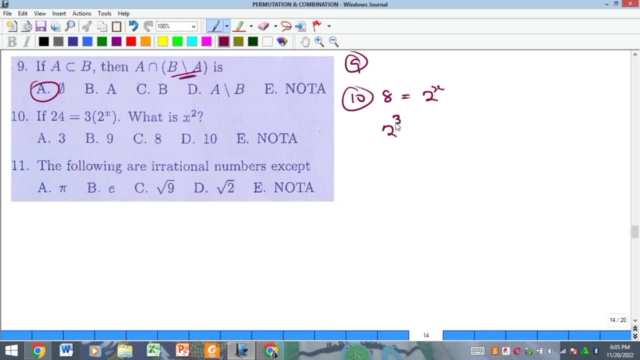 i'll, i'll take two of them to the same base, and then, uh, therefore, my x becomes equal to what three? and so they say we should find x squared, which is three squared, and that is 9. and then number 11 says the following are irrational numbers except: so this is: 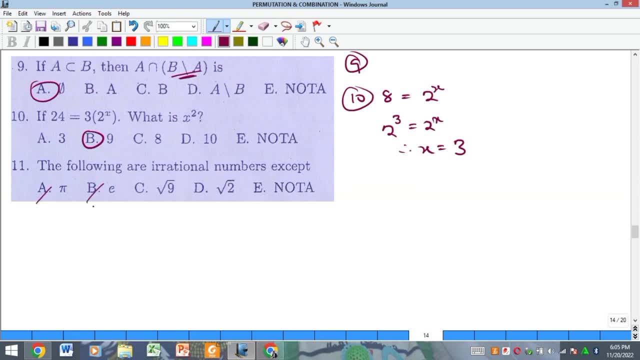 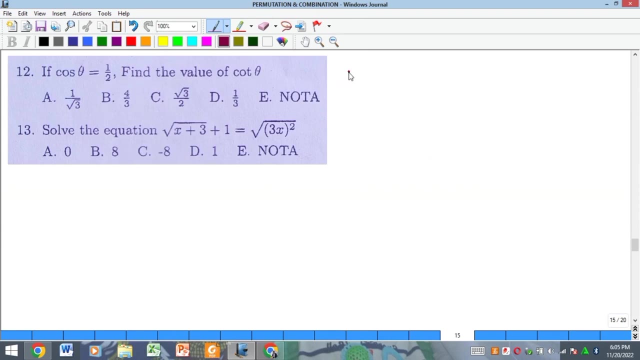 a an irrational number. this is an irrational number. now, the square root of nine is three, and three is not an irrational number, so c is the correct answer here. number 12: the question says that cos theta is equal to half. what does that mean? if cos theta is equal to half, it means that. 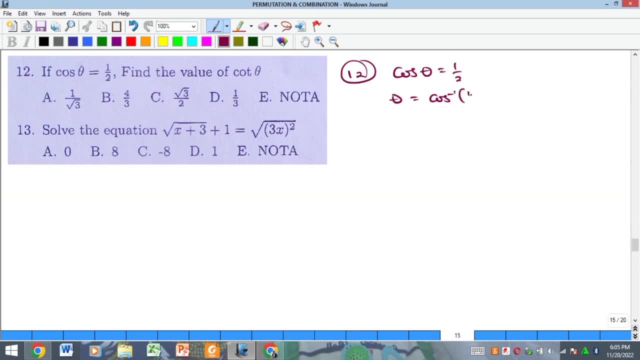 t is equal to half, and that means that t is zero. and so we have: t is equal to half, and that is is cos inverse of half, and cos inverse of half is 60 degrees. and so they say we should find the value of cot. but we know that cot is one all over tangent, so let's quickly get our tangent. 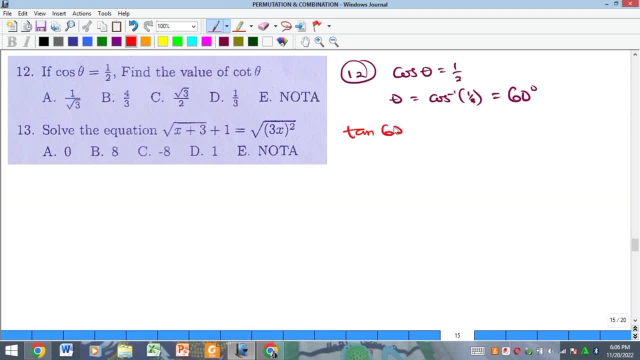 what is the value of tan 60? tan 60 is actually root 3, and so that means that cot 60, which is the theta, is then going to be one all over the root of 3, and that's our solution, which is a. so we go to a number, 13. 13 says that we should solve this, and what are you going to do? first, 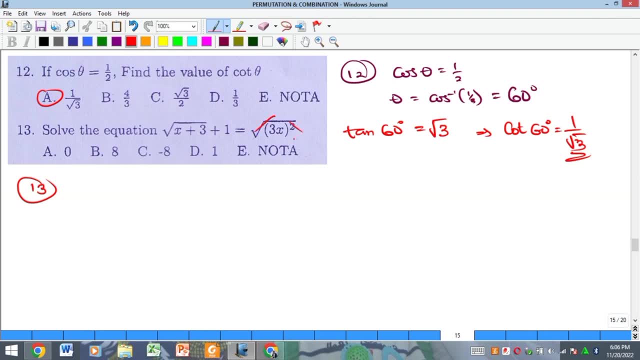 of all see here that we can actually remove this. the square can remove the square roots, and so here we just have only the square of this plus 3 plus 1, equal to 3x. so i can take this to the other side. so the the 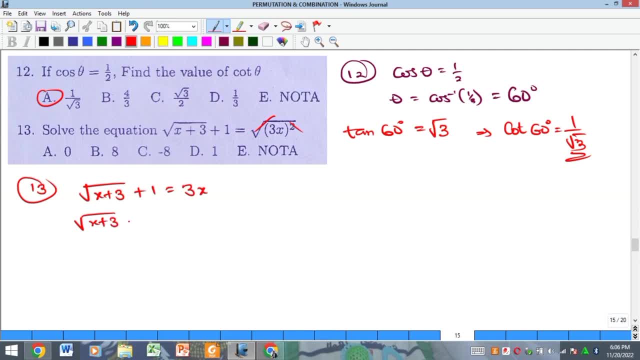 the just have the square root of x plus 3, equal to 3x minus 1. now let the square root go to this side, then it becomes a square, and so i'll just take the square of both sides. so if i take the square of both sides, i am going to have. this will go, so i'll just have x plus 3 and that's equal to the. 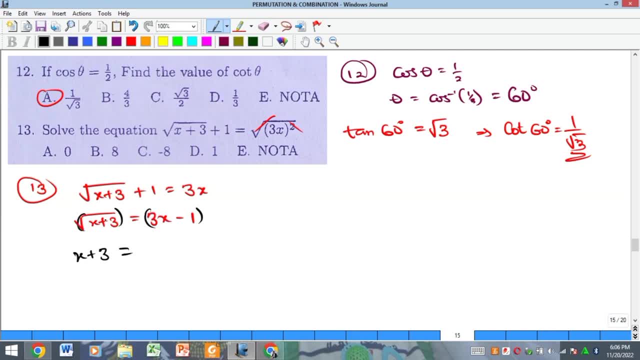 square of this side. let me quickly put it this way: so the square of this is going to be 9x squared minus 6x plus 1, so collect like terms. let everything here go this way. so i'll have 9x squared s coming here will become minus x, and that will give me minus 7x 3 coming here will. 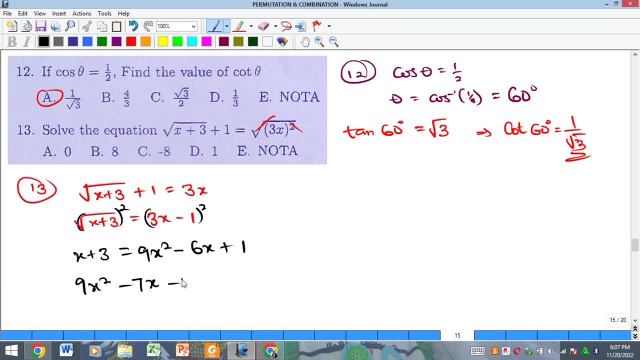 become minus 3. 1 minus 3 is minus 2. everything is equal to 0. and to solve this, if you go to my previous video, just the video before this, you are going to see that to solve, or, sorry, under how to factorize? so i cannot. 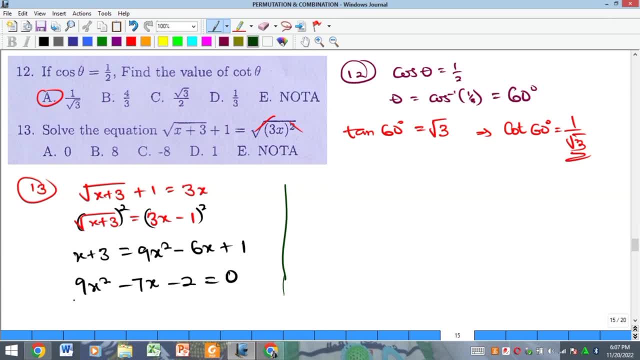 you can see that to solve or sorry under how to factorize. you can see that to solve or sorry under how to factorize this. if you multiply 9 and minus 2, you this: if you multiply 9 and minus 2, you have minus 18. so what are the two factors of minus 18? that? 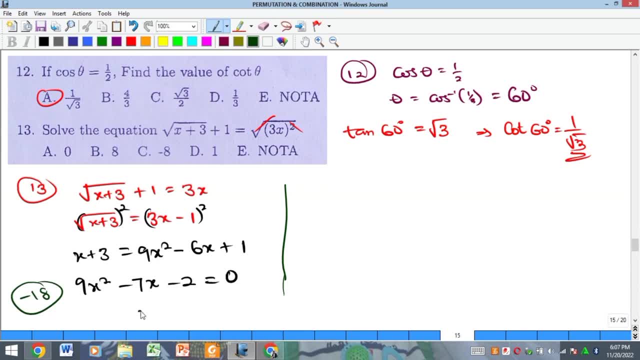 have minus 18. so what are the two factors of minus 18? that will sum to minus 7 and that is minus 9, will sum to minus 7 and that is minus 9 and positive 2.. so i will just come here open my 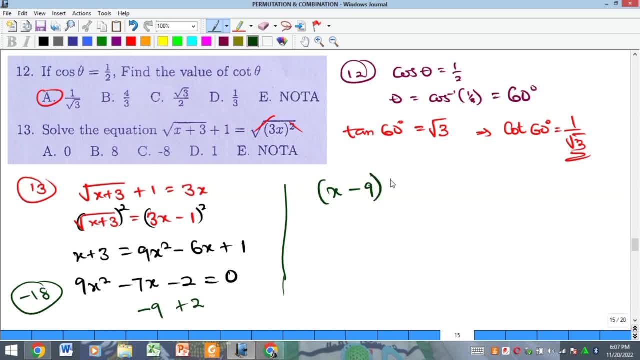 and positive 2.. so i will just come here, open my bracket, put minus 9 open. another one, put positive bracket, put minus 9 open. another one put positive 2 and that is equal to 0, but the coefficient here 2 and that is equal to 0, but the coefficient here is not one. so we pick that coefficient, use it to. 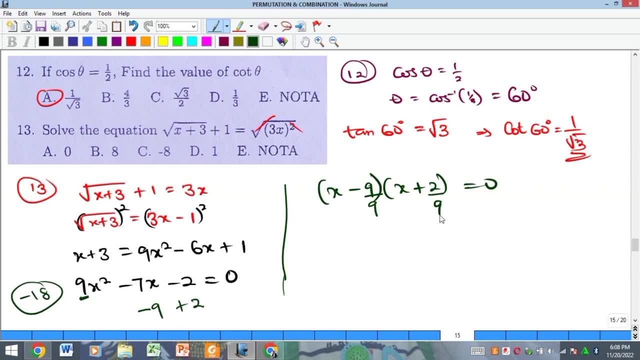 is not one. so we pick that coefficient, use it to divide this number. use it to divide this, so this divide this number. use it to divide this, so this will go away. you have x minus one will go away. you have x minus one is zero or x is equal to minus two over. 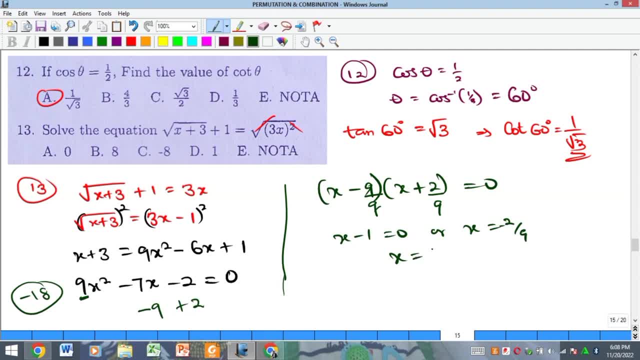 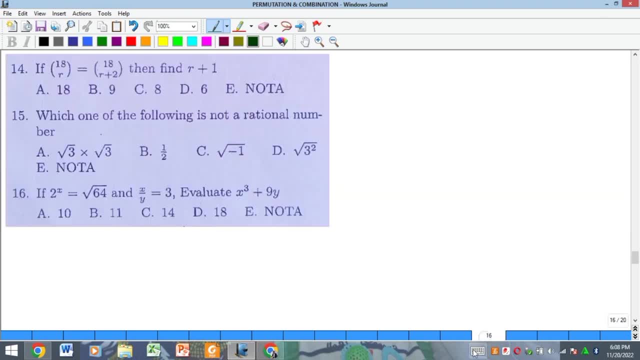 is zero or x is equal to minus two over nine. so if you solve this side, you have x is positive nine. so if you solve this side, you have x is positive one and there is positive one here, one and there is positive one here, and that is our solution. so for the next one, number 14, here, 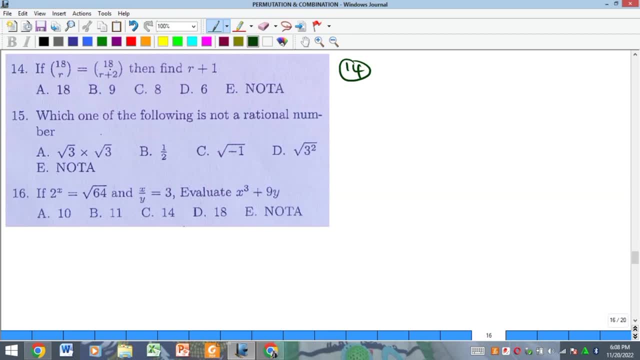 and that is our solution. so for the next one, number 14, here we have that if this is equal to this, and we have that if this is equal to this. and what's the meaning of this? this thing actually means? what's the meaning of this? this thing actually means combination. this is another way to write. 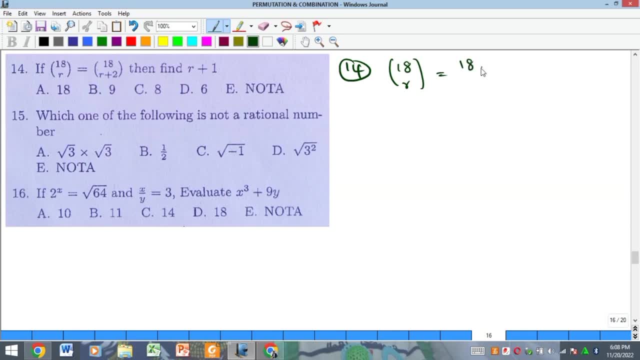 combination. this is another way to write combination. that's a thin combination r combination. that's a thin combination r combination. that's a thin combination r. okay, so this is 18 combination r, but however. okay. so this is 18 combination r, but however. okay, so this is 18 combination r, but however, that's not where i am interested in going. but 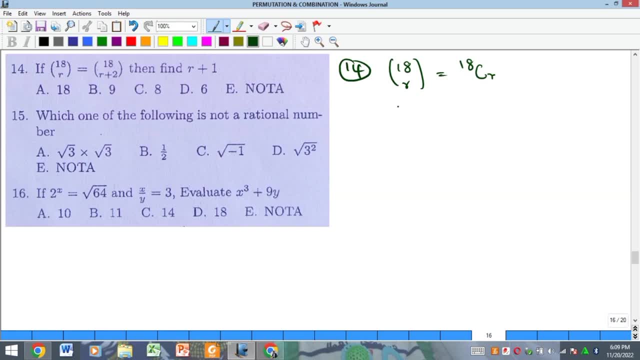 that's not where i am interested in going. but that's not where i am interested in going. but we can use that. so that means the other one. we can use that. so that means the other one. we can use that. so that means the other one is a thin combination, r plus two. now there is a law. 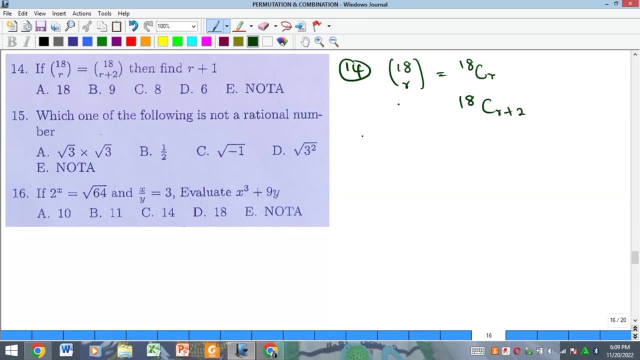 is a thin combination: r plus two. now there is a law is a thin combination: r plus two. now there is a law which we call the complement, which we call the complement, which we call the complement rule under combination and permutation rule, under combination and permutation rule, under combination and permutation, especially combination, which says that if 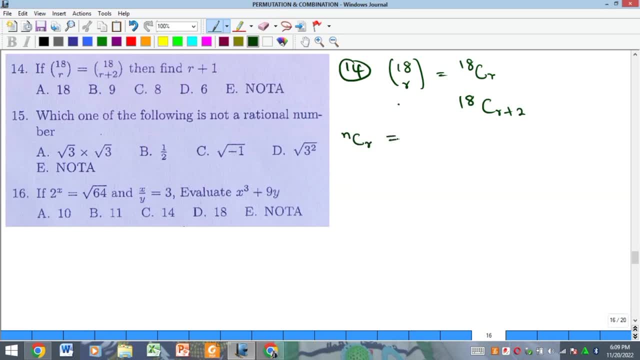 especially combination which says that if, especially combination which says that if n, n, n cr is equal to n, cr is equal to n, cr is equal to n c. let's say r plus one. let me use this as c. let's say r plus one. let me use this as: 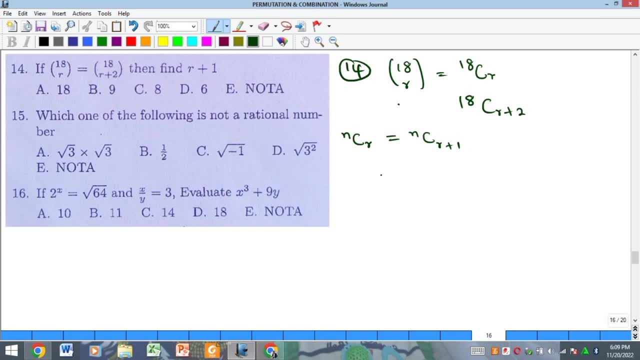 c, let's say r plus one. let me use this as an example. what it means is that n is an example. what it means is that n is an example. what it means is that n is equal to the sum of these two, which is i equal to the sum of these two, which is i. 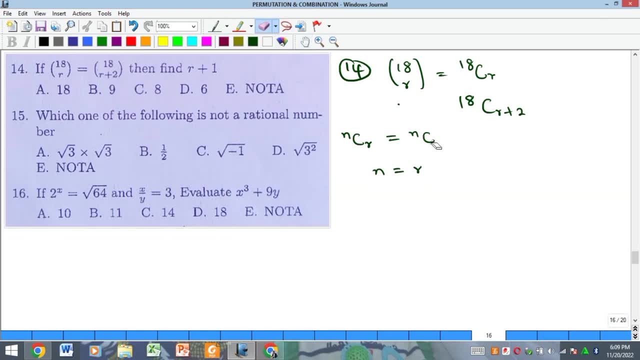 equal to the sum of these two, which is: i should have just used another another, should have just used another another, should have just used another. another letter here, maybe letter here, maybe letter here, maybe k. so it means that n is equal to r plus k. so it means that n is equal to r plus. 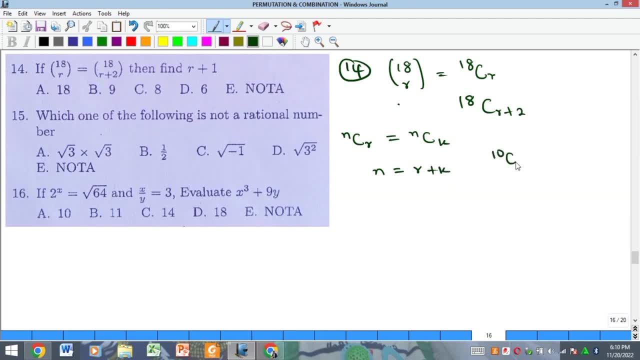 k. so it means that n is equal to r plus k. so if you have 10 combination, 3 is k. so if you have 10 combination 3 is k. so if you have 10 combination, 3 is equal to 10 combination 7. the sum below: 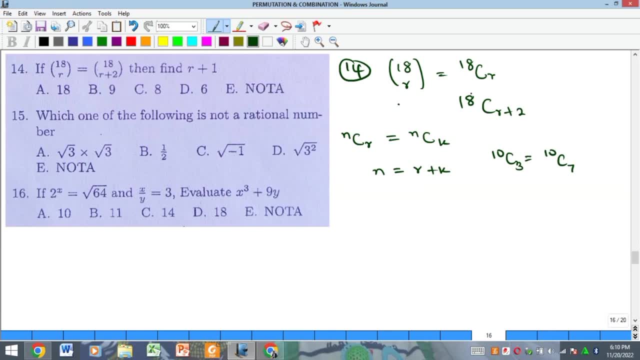 equal to 10 combination 7. the sum below equal to 10 combination 7. the sum below must be equal to your n. so if we use must be equal to your n. so if we use must be equal to your n. so if we use that rule here, what it means is that 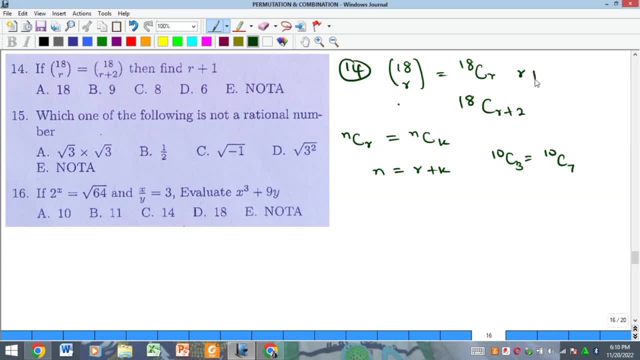 that rule here. what it means is that that rule here. what it means is that our r, if we sum this to r plus r plus our r, if we sum this to r plus r plus our r, if we sum this to r plus r plus 2, it must be equal to the n, which is 18. 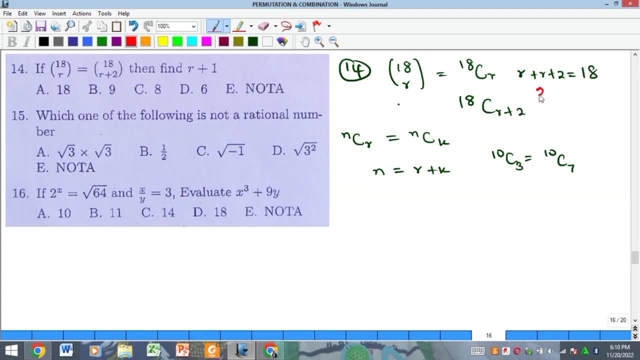 2 it must be equal to the n, which is 18. 2 it must be equal to the n, which is 18. and then, solving from there, this is going, and then solving from there, this is going, and then solving from there, this is going to give us 2r. 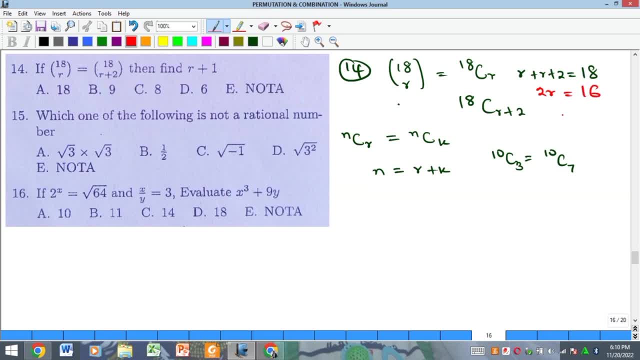 to give us 2r. to give us 2r is equal to 18 minus 2, which is 16, is equal to 18 minus 2, which is 16, is equal to 18 minus 2, which is 16. therefore, our r is 8 number, the. 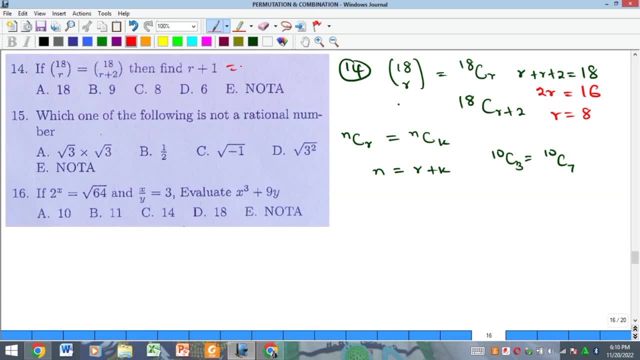 therefore our r is 8 number. the, therefore our r is 8 number. the question says we should find r plus 1. question says we should find r plus 1. question says we should find r plus 1, which is equal to 9, and that's option b. 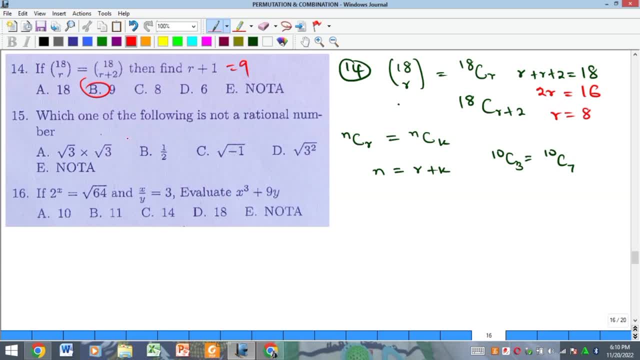 which is equal to 9, and that's option b, which is equal to 9, and that's option b. now this one says which one of the: now, this one says which one of the. now, this one says which one of the following following: following is not a rational number and, of course, 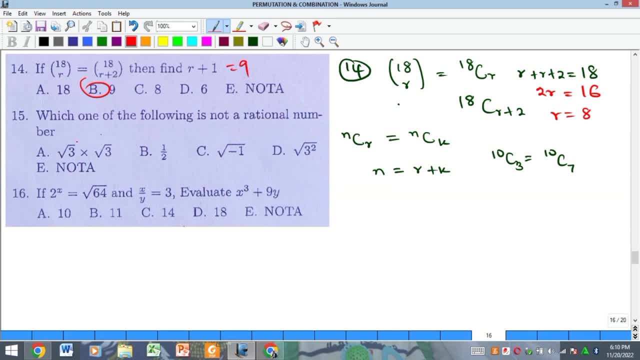 is not a rational number and of course is not a rational number. and of course, this, this, this, multiply this is going to give you three. multiply this is going to give you three. multiply this is going to give you three is a rational number. this is already a. 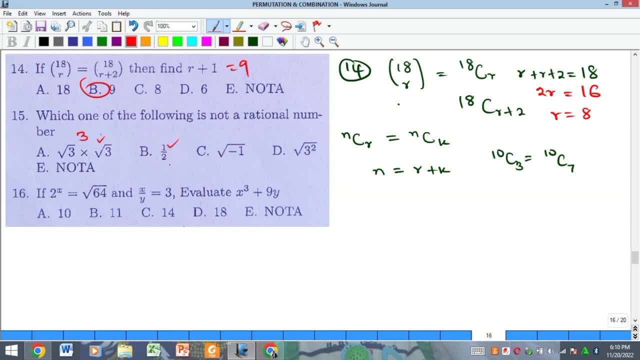 is a rational number. this is already. a is a rational number. this is already a rational number. that's a fraction of rational number. that's a fraction of rational number. that's a fraction of integers. now, this is definitely not a integers. now, this is definitely not a. 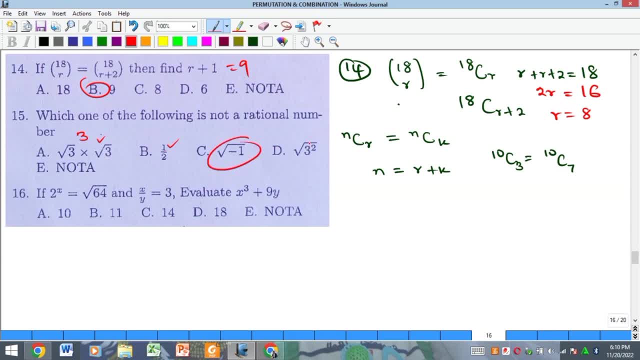 integers. now, this is definitely not a rational number. now, of course, this is rational number. now, of course, this is rational number. now, of course, this is going to cancel the square root. you also going to cancel the square root. you also going to cancel the square root. you also have three. so this is also rational. so 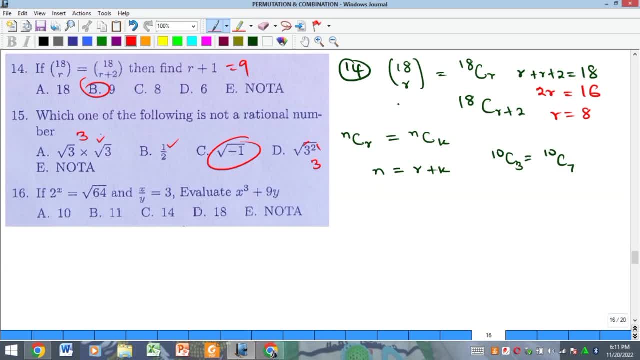 have three, so this is also rational. so have three, so this is also rational. so the answer, the answer, the answer is c. finally, for this, we have the number is c. finally, for this, we have the number is c. finally, for this, we have the number 16. 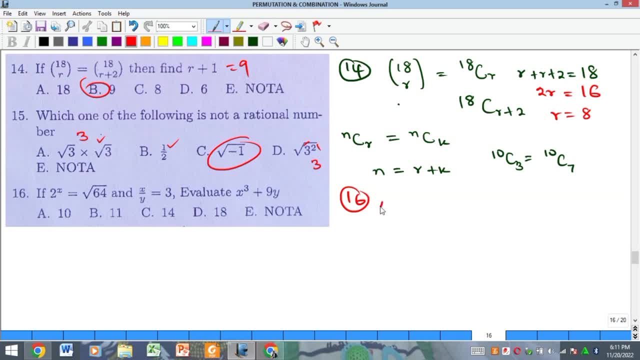 16. 16, which says that two raised to power of x. which says that two raised to power of x. which says that two raised to power of x is equal to root of 64 and root of 64 is: is equal to root of 64 and root of 64 is: 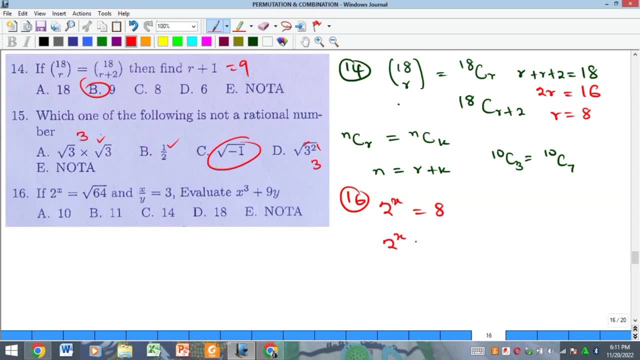 is equal to root of 64, and root of 64 is equal to eight. so that means, if i take equal to eight, so that means if i take equal to eight, so that means, if i take this by indices, i'll have two. this by indices, i'll have two. 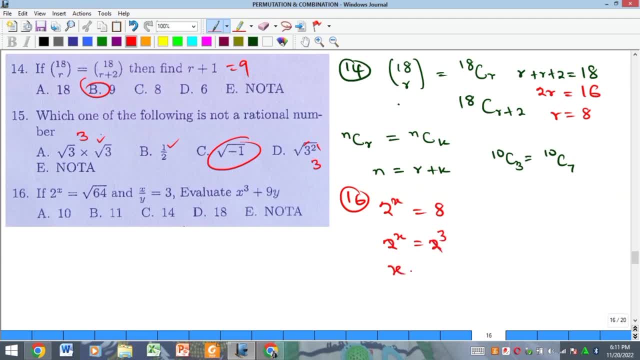 this by indices. i'll have two raised to power of three. if i remove the raised to power of three, if i remove the raised to power of three, if i remove the equal basis, x is equal to three. equal basis x is equal to three. equal basis x is equal to three. and then they said this other equation: 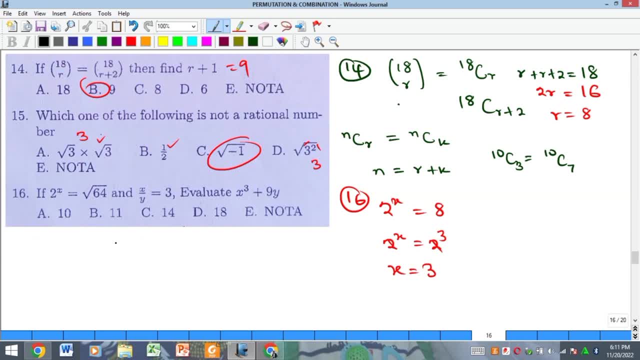 and then they said this other equation, and then they said this other equation holds. what that means is that, since my x holds, what that means is that, since my x holds, what that means is that, since my x is three, i can have three over y. is is three, i can have three over y is. 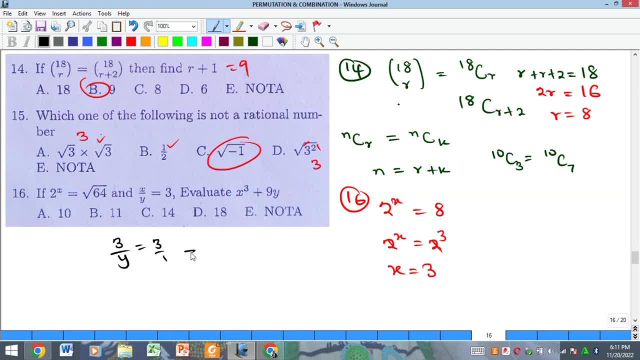 is three. i can have three over. y is equal to three over one cross multiply equal to three over one cross multiply equal to three over one cross multiply. you have that three y is equal to three. you have that three y is equal to three. you have that three y is equal to three. therefore, y is equal to three over three. 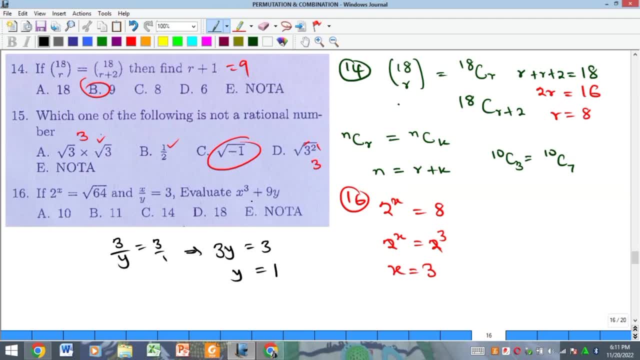 therefore, y is equal to three over three. therefore, y is equal to three over three, which is one which is one which is one. so then, to evaluate this, just substitute. so then, to evaluate this, just substitute. so then, to evaluate this, just substitute your x, your x, your x and your y. so, if i put my x as three, 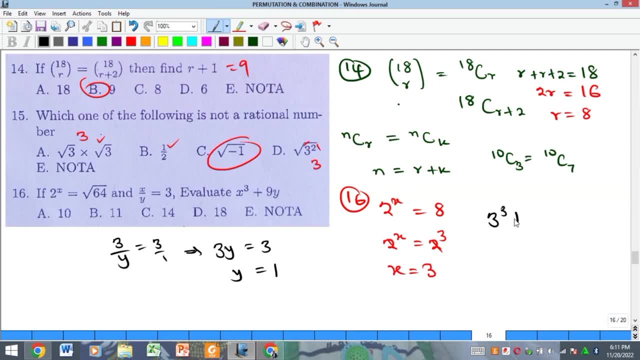 and your y. so if i put my x as three and your y, so if i put my x as three, then three raised to power three plus then three raised to power. three plus then three raised to power three plus nine times one, and that's going to give. 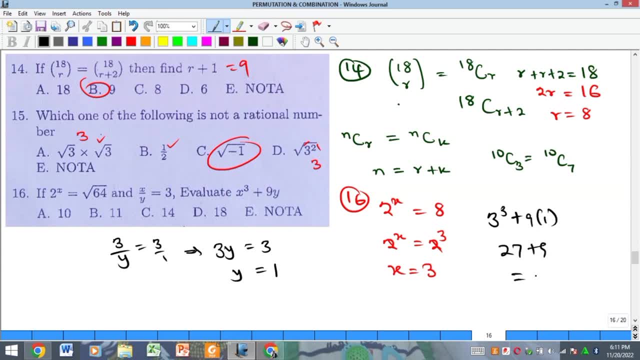 nine times one, and that's going to give nine times one, and that's going to give me 27 plus me, 27 plus me, 27 plus nine, which is equal to 36, and that is the nine which is equal to 36, and that is the. 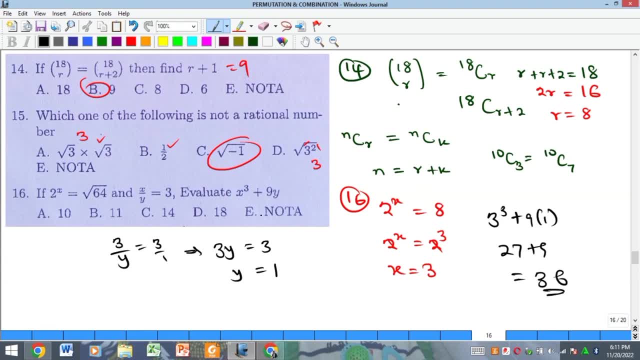 nine, which is equal to 36, and that is the solution. so of course you can see the solution. so of course you can see the solution. so of course you can see the answer is not here, answer is not here, answer is not here. so the none of the above becomes our. 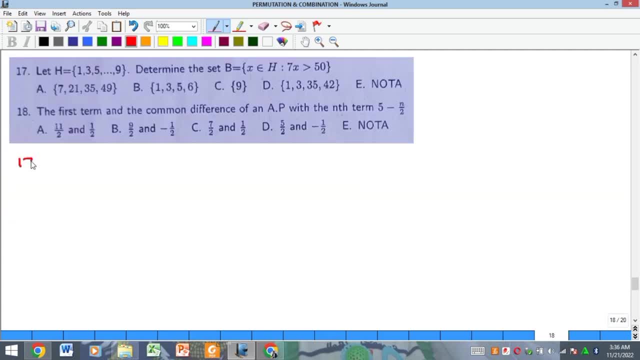 so the none of the above becomes our. so the none of the above becomes our solution, solution, solution. so for number 17, now. so for number 17. now, so for number 17. now we are asked to determine what set b. we are asked to determine what set b. 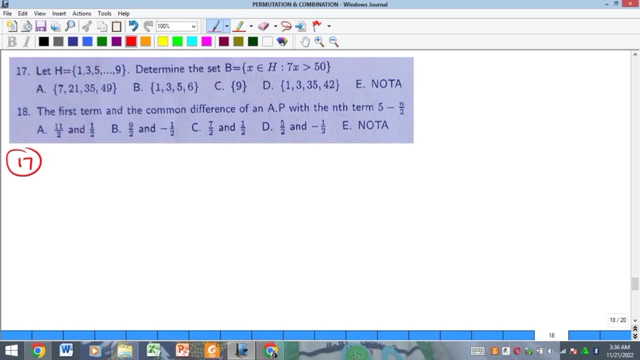 we are asked to determine what set b and what is the first thing that the and what is the first thing that the and what is the first thing that the elements of set b, elements of set b, elements of set b must be from set h must be from set h. 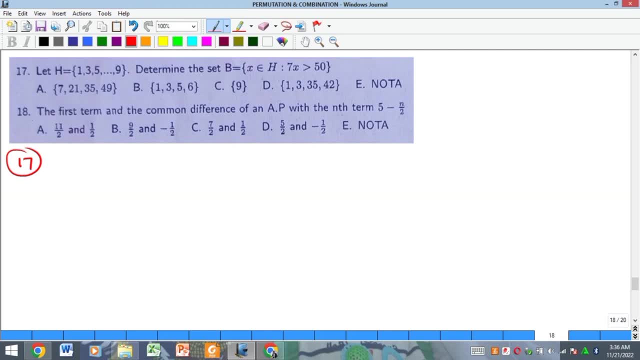 must be from set h and such that this happens so for that to, and such that this happens so for that to, and such that this happens, so for that to be what and meanwhile, what is our set h? be what, and meanwhile, what is our set h? be what, and meanwhile, what is our set h? this is our set h. 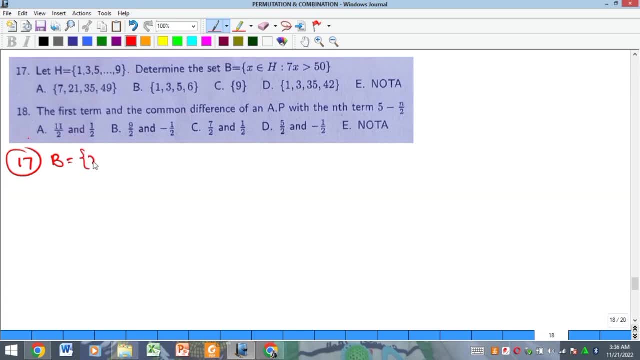 this is our set h. this is our set h. so b is such that. so b is such that. so b is such that x is in h. so all of this h, x is in h. so all of this h, x is in h. so all of this h such that. 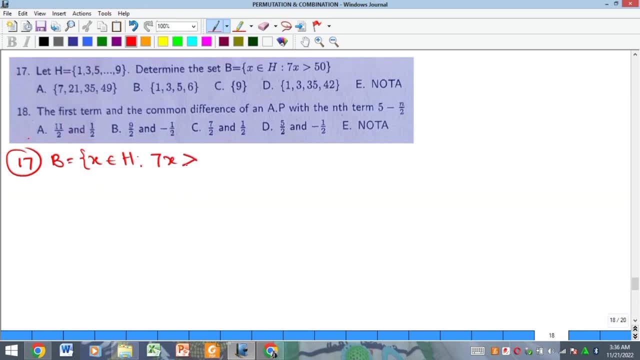 such that, such that any x you pick must be when you any x you pick must be when you any x you pick must be when you multiply by seven must be greater than multiply by seven must be greater than multiply by seven must be greater than fifty. so all we need to do is to solve. 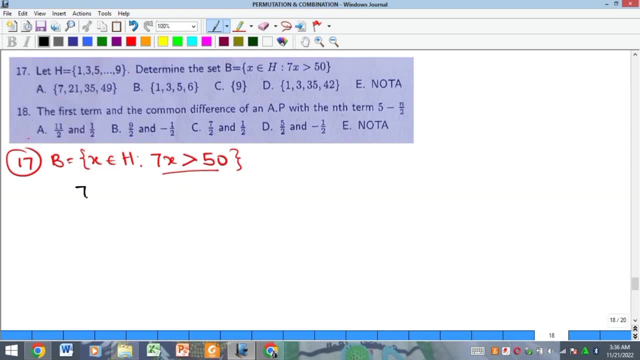 fifty. so all we need to do is to solve fifty. so all we need to do is to solve this inequality, this inequality, this inequality, and we divide both sides by seven, and we divide both sides by seven, and we divide both sides by seven. if you divide both sides by seven, we'll. 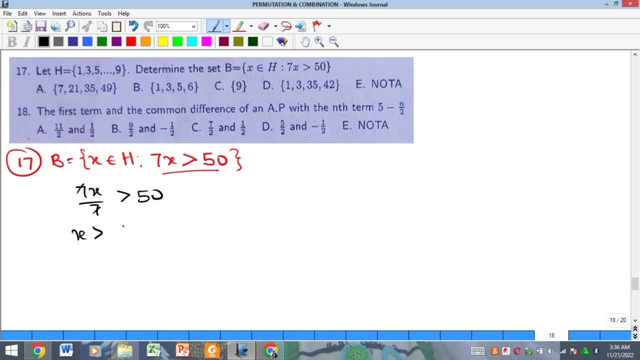 if you divide both sides by seven, we'll. if you divide both sides by seven, we'll have that our x have that. our x have that. our x must be greater than seven over, must be greater than seven over, must be greater than seven over fifty over seven, which is seven whole. 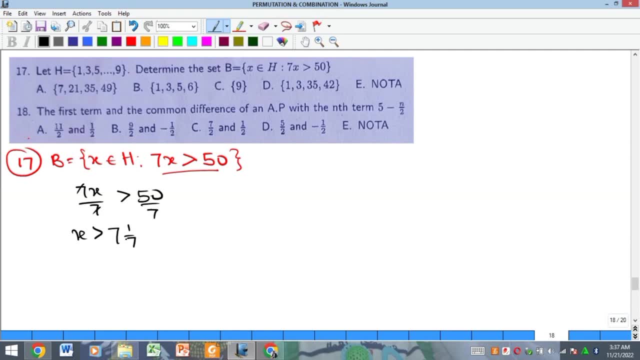 fifty over seven, which is seven whole. fifty over seven, which is seven whole, number one over seven. so something number one over seven, so something number one over seven, so something greater than seven, eight, nine and all of greater than seven, eight, nine and all of greater than seven, eight, nine and all of that. okay, so we come back to h to check. 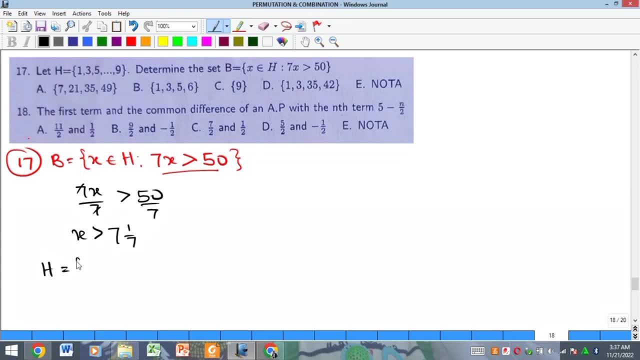 that okay. so we come back to h to check that. okay. so we come back to h to check. meanwhile, what is our h? meanwhile, what is our h? meanwhile, what is our h? our h is actually a set of our h is actually a set of our h is actually a set of odd numbers. we have one, three. 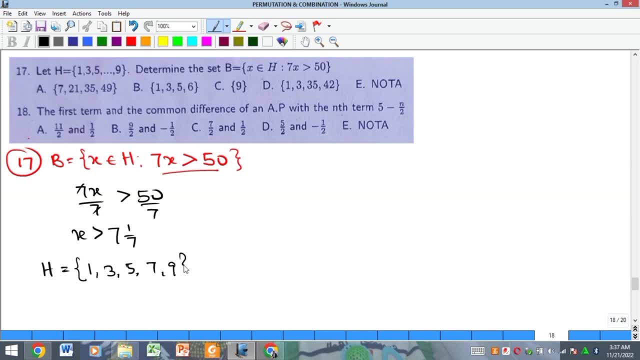 odd numbers. we have one, three odd numbers. we have one, three, five, then seven and nine. so among all five, then seven and nine, so among all five, then seven and nine. so among all of these, the only one that satisfies this, of these, the only one that satisfies this. 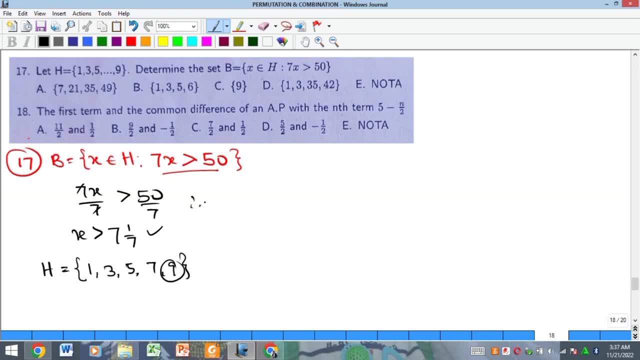 of these, the only one that satisfies this condition is: what condition is? what condition is what? nine, therefore, our set b is a singleton. nine, therefore, our set b is a singleton. nine, therefore, our set b is a singleton set containing only nine, so c. set containing only nine, so c. 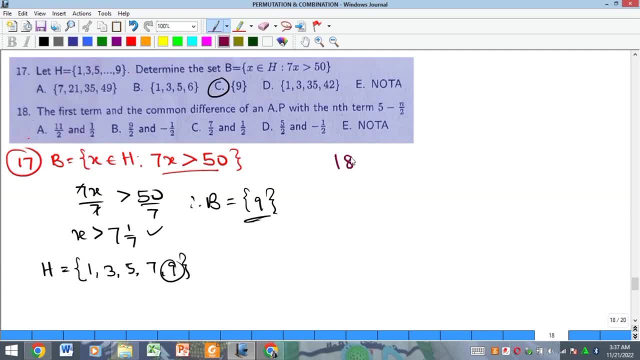 set containing only nine. so c is the correct answer here, so we go to. is the correct answer here, so we go to. is the correct answer here. so we go to number 18 here. now. remember that number, number 18 here. now. remember that number, number 18 here. now. remember that number 17 is from set theory, now from 1818 is. 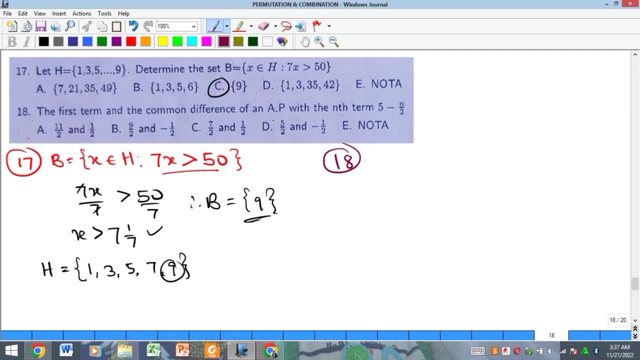 17 is from set theory, now from 1818 is 17 is from set theory, now from 1818, is from, from from sequences and series, particularly sequences and series, particularly sequences and series, particularly arithmetic progression. so we are giving arithmetic progression, so we are giving 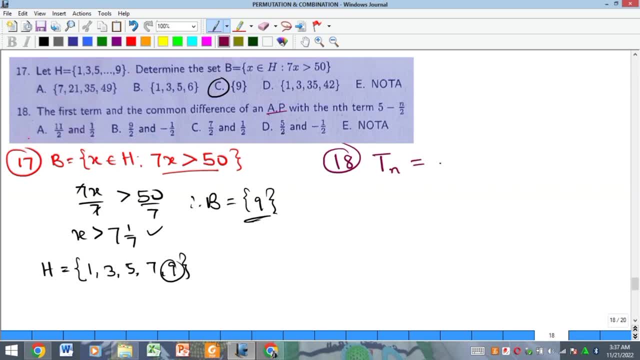 arithmetic progression. so we are giving a, an expression for the t a, an expression for the t a, an expression for the t n stem, and the set is equal to 5 n stem, and the set is equal to 5 n stem, and the set is equal to 5 minus n over 2. so the meaning is that: 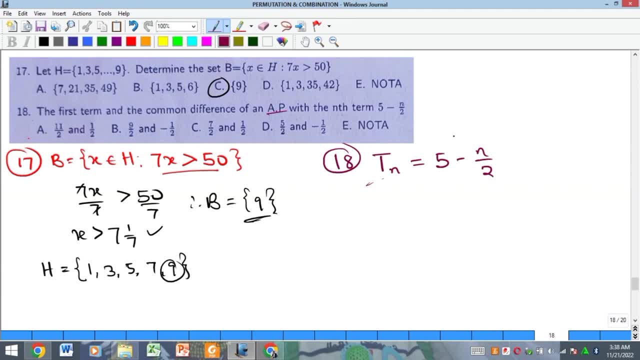 minus n over 2. so the meaning is that minus n over 2. so the meaning is that whatever t you want to find, just whatever t you want to find, just whatever t you want to find, just substitute your n, substitute your n, substitute your n. so now they ask us to find t1. that's the 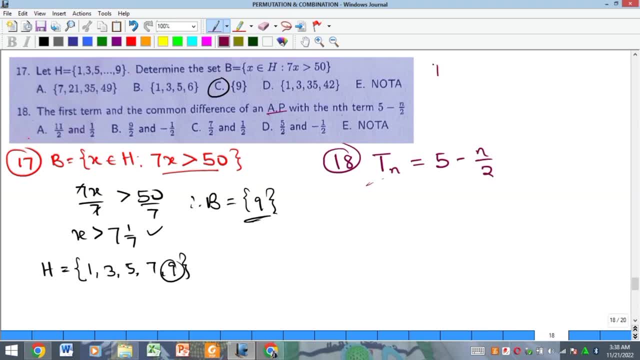 so now they ask us to find t1. that's the. so now they ask us to find t1. that's the first term, first term, first term, and the common difference now t1 here and the common difference now t1 here and the common difference now t1 here means that 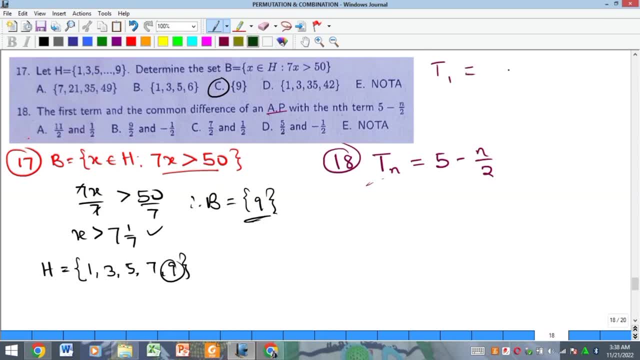 means that? means that anywhere i see n, i should call it one. anywhere i see n, i should call it one. anywhere i see n, i should call it one, and that's going to give me 5 minus, and that's going to give me 5 minus. 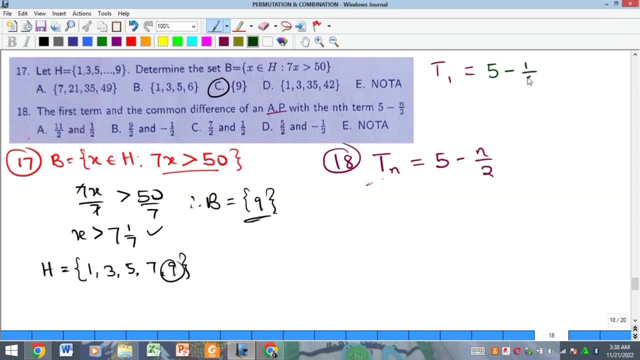 and that's going to give me 5 minus 1, all over 1, all over 1, all over 2, and when you subtract this, you have 4: 2, and when you subtract this, you have 4: 2, and when you subtract this, you have 4 over 5, which is actually the same thing. 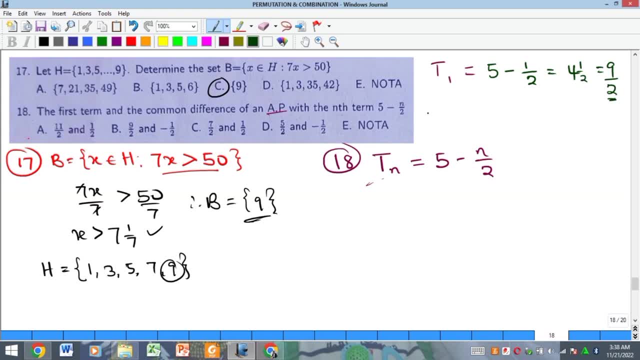 over 5, which is actually the same thing over 5, which is actually the same thing as 9 over 2, as 9 over 2, as 9 over 2. so what about the common difference? so what about the common difference? so what about the common difference? remember that there's a formula that 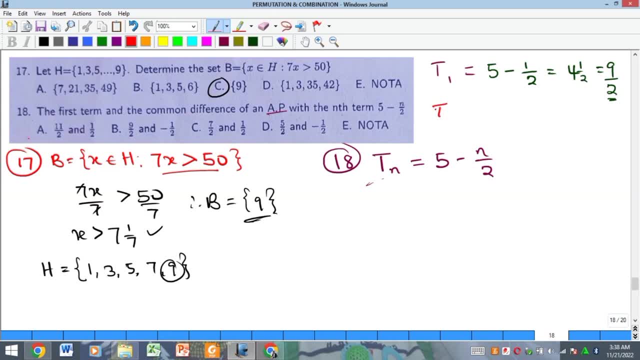 remember that there's a formula that remember that there's a formula that says that common difference says that common difference says that common difference d- sorry, says that common difference d is equal to. says that common difference d is equal to. says that common difference d is equal to c? n minus t, n minus 1. what this means. 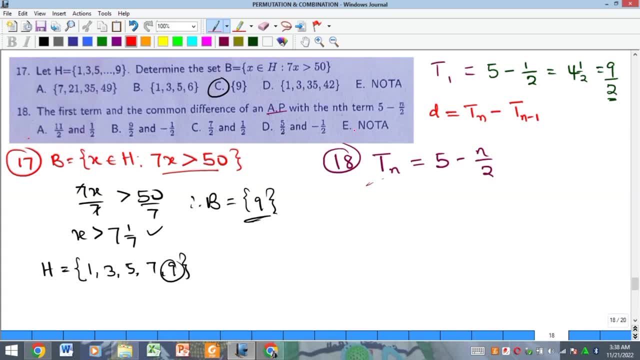 c? n minus t? n minus 1. what this means: c? n minus t? n minus 1. what this means is that if i want to find a common, is that if i want to find a common is that, if i want to find a common difference of an arithmetic progression. 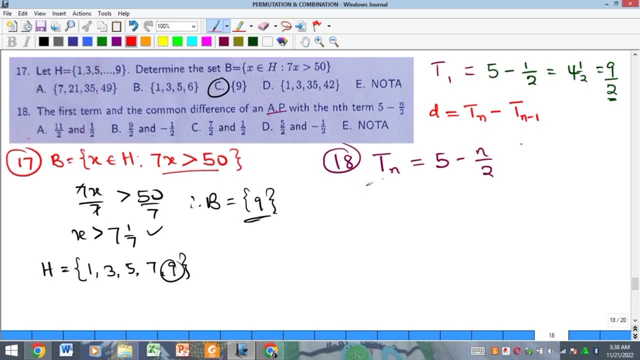 difference of an arithmetic progression. difference of an arithmetic progression. all i need to do is to get a term, and all i need to do is to get a term, and all i need to do is to get a term and subtract the previous term. subtract the previous term. 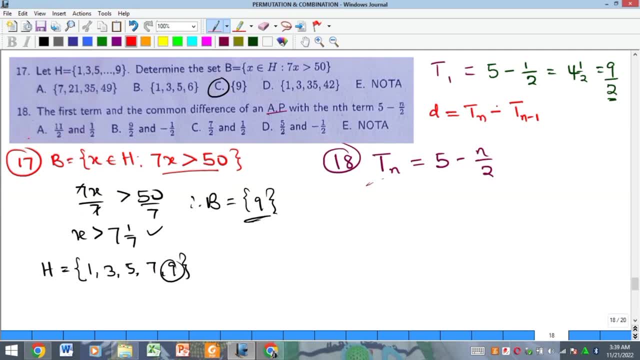 subtract the previous term. so, in this case for me to get this, i so, in this case for me to get this, i so, in this case for me to get this, i will need at least the t2, will need at least the t2, will need at least the t2. so let's get our t2, so our t2 is going. 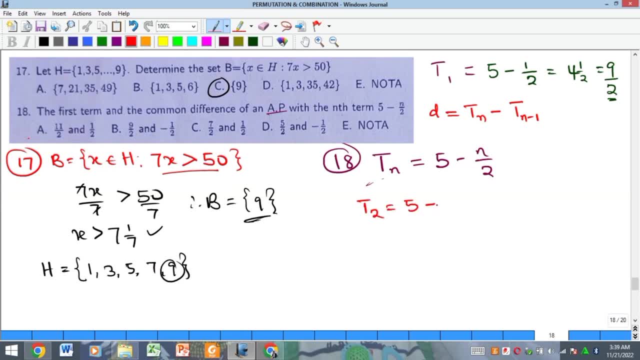 so our t2 is going to be five minus our n now will be two to be five minus our n now will be two to be five minus our n now will be two, all over two, and this is going to give all over two, and this is going to give. 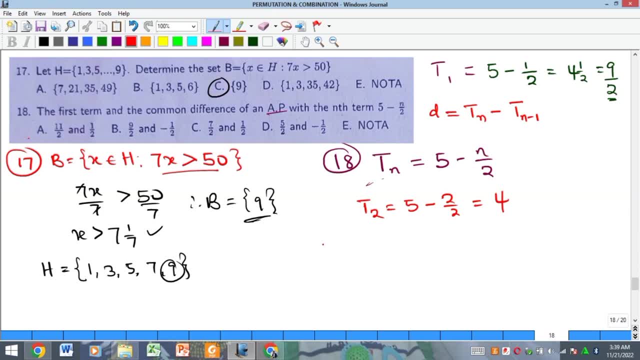 all over two and this is going to give us four. of course two over two is one, us four. of course two over two is one, us four. of course two over two is one. so that now means that our common, so that now means that our common, so that now means that our common difference is going to be equal to 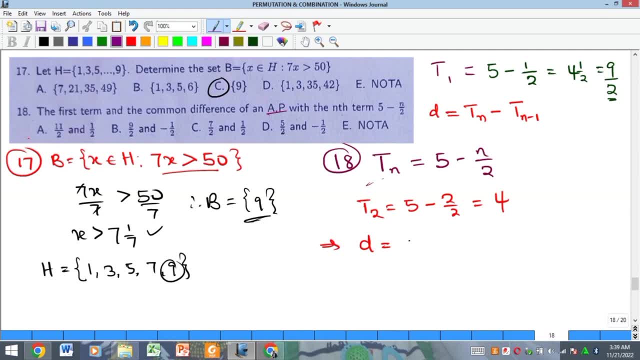 difference is going to be equal to. difference is going to be equal to our d, that is equal to t2. our d, that is equal to t2. our d, that is equal to t2 minus t1. and what is our t2 minus t1 and what is our t2? 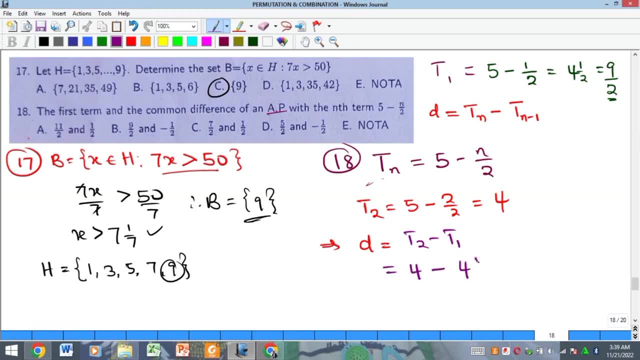 minus t1. and what is our t2 four and our t1 is four and a half four and our t1 is four and a half four and our t1 is four and a half. so if you subtract this, you have minus. so if you subtract this, you have minus. 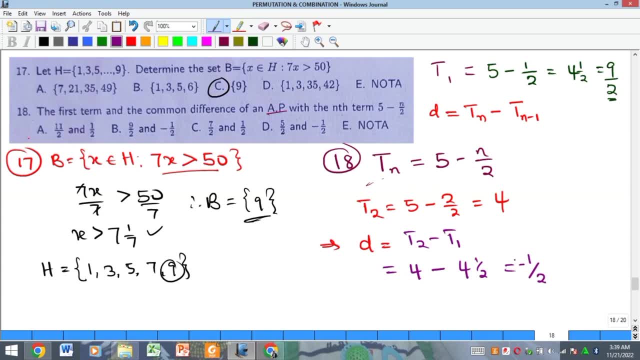 so, if you subtract this, you have minus half left. therefore, what they're asking, half left. therefore, what they're asking, half left. therefore, what they're asking us to get is us to get is us to get is nine over two and nine over two and nine over two and minus half, which is actually option. 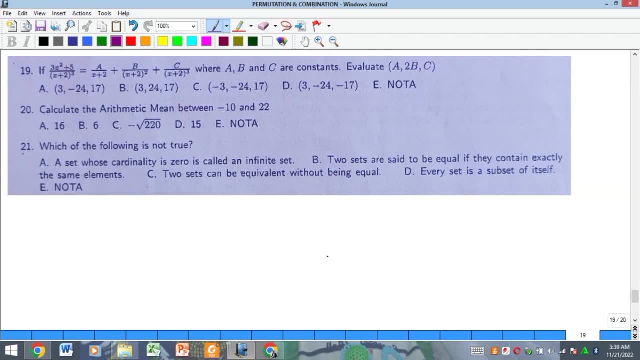 minus half, which is actually option, minus half, which is actually option b. so we move over to the next one number b. so we move over to the next one number b. so we move over to the next one number, 19, 19, 19, which is from partial fractions, and they: 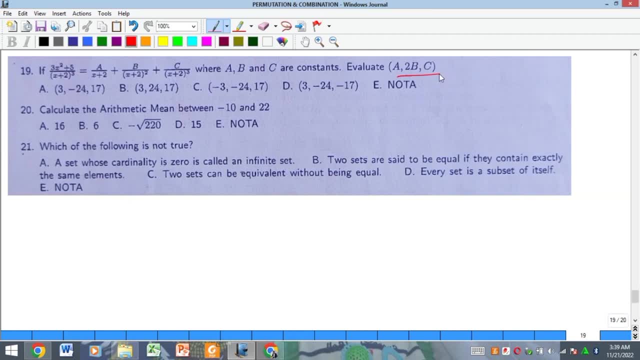 which is from partial fractions, and they which is from partial fractions, and they are only asking us to get this, are only asking us to get this, are only asking us to get this and to evaluate this, we will need a- b, and to evaluate this, we will need a- b. 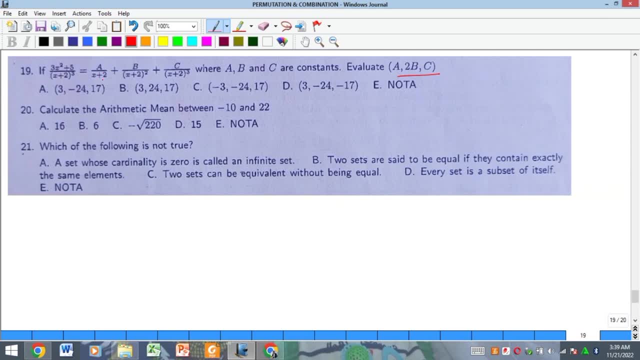 and to evaluate this we will need a, b and c. so all we need to do is to split and c. so all we need to do is to split and c. so all we need to do is to split this into a special fraction, this into a special fraction. 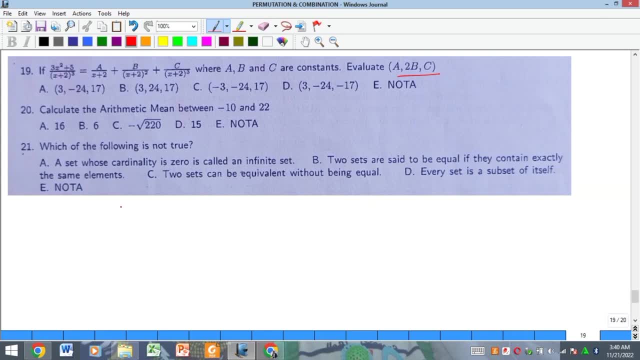 this into a special fraction: get the values of a, b and c and then put: get the values of a, b and c, and then put: get the values of a, b and c and then put it here, it here, it here. so let's start doing that, and so that's. 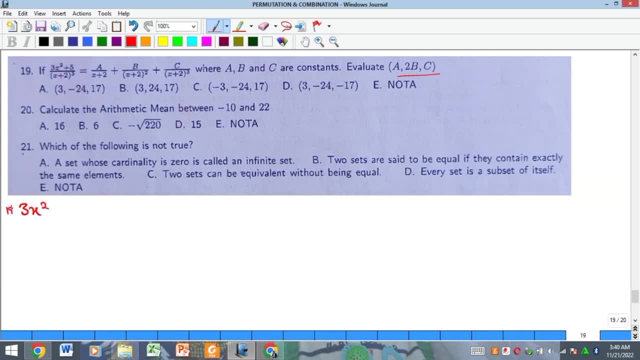 so let's start doing that, and so that's so, let's start doing that, and so that's going to give us 3 going to give us 3, going to give us 3 x squared. that's for 19: 3 x squared all x squared. that's for 19: 3 x squared all. 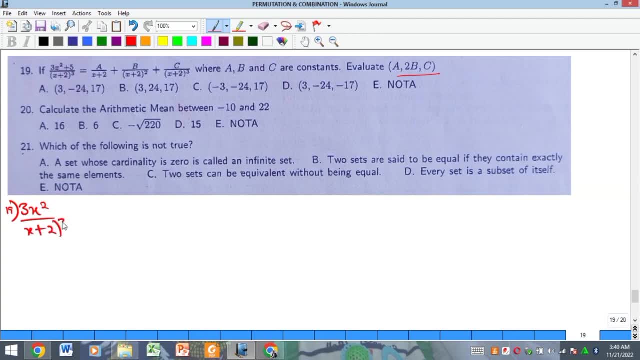 x squared, that's for 19: 3 x squared all over x plus 2, or cubed over x plus 2, or cubed over x plus 2, or cubed is equal to, so i'm going to quickly take. is equal to, so i'm going to quickly take. 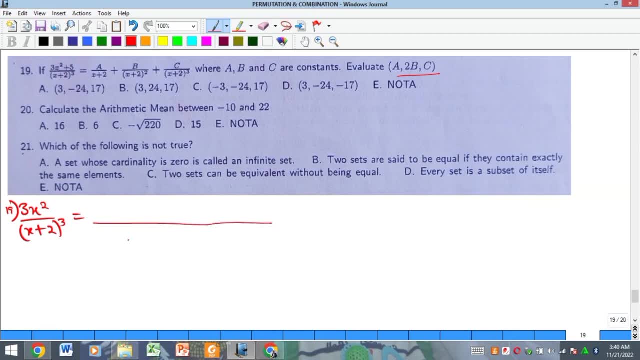 is equal to. so i'm going to quickly take the lcm of the lcm, of the lcm of the right hand side: the lcm is x plus 2. the right hand side, the lcm is x plus 2. the right hand side: the lcm is x plus 2. raise to the power of 3. 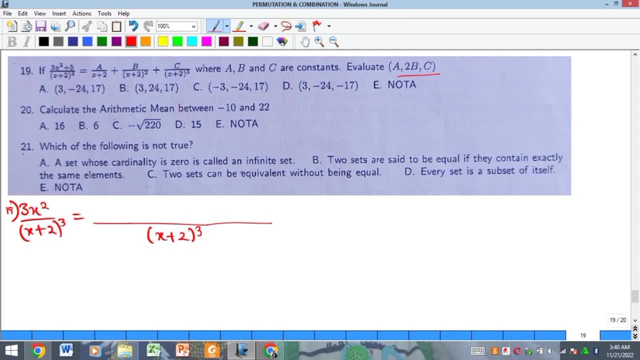 raise to the power of 3, raise to the power of 3, so i'll use this to divide, and then when so, i'll use this to divide, and then when. so i'll use this to divide, and then when it divides, what am i going to get? 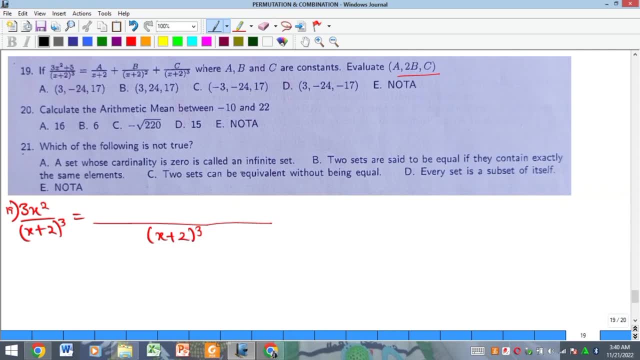 what am i going to get? what am i going to get? i will have x plus 2 squared left. so i will have x plus 2 squared left. so i will have x plus 2 squared left. so you use it to multiply. you use it to multiply. 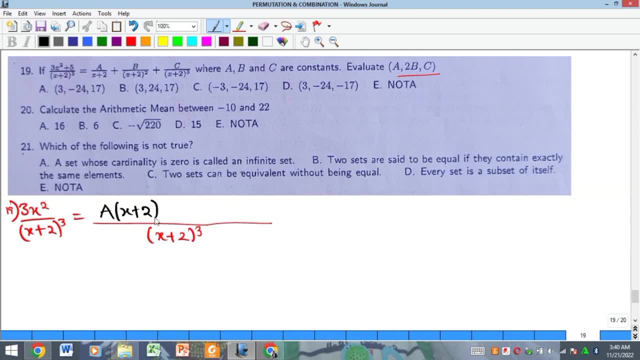 you use it to multiply a. so i will have 8 a times this a. so i will have 8 a times this a. so i will have 8 a times this squared, then plus i will go to b squared, then plus i will go to b. 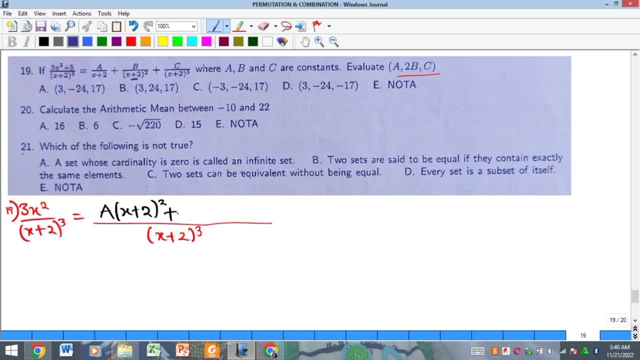 squared, then plus, i will go to b. use the denominator to divide and then use the denominator to divide, and then use the denominator to divide, and then i'll get only x plus 2. use it to. i'll get only x plus 2. use it to. 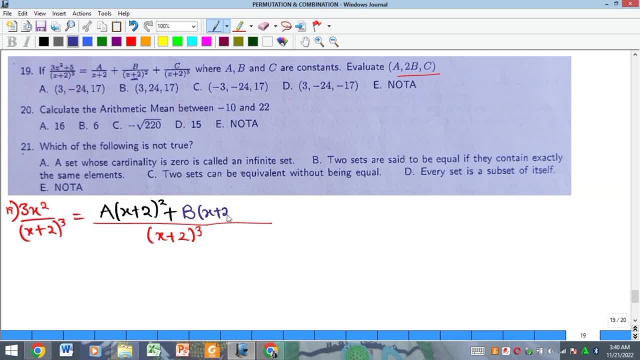 i'll get only x plus 2. use it to multiply b, multiply b, multiply b, and that will give me this, then plus i, and that will give me this, then plus i, and that will give me this, then plus i will go to my c. use this to divide. 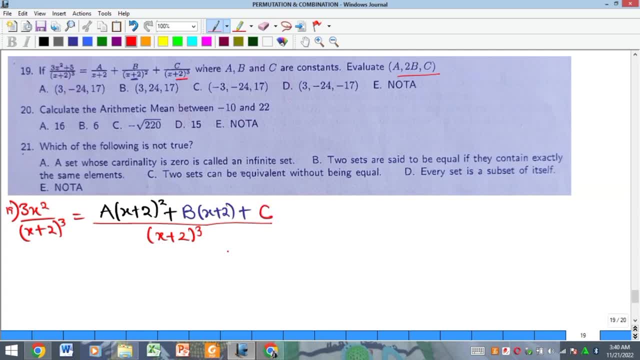 will go to my c. use this to divide. will go to my c. use this to divide, which will give me one, which will give me one, which will give me one one times c is c, and so by one times c is c, and so by one times c is c, and so by normal partial fraction, the denominators. 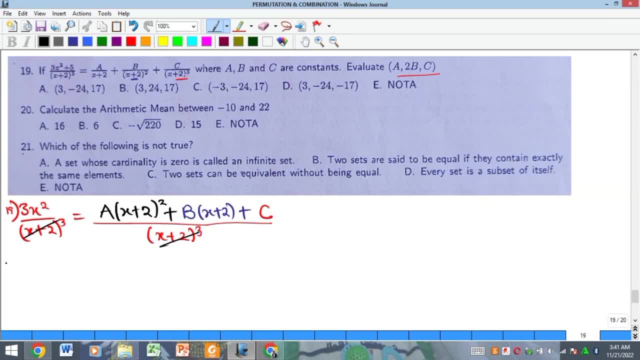 normal partial fraction: the denominators- normal partial fraction: the denominators- will cancel. and then i will get that the will cancel, and then i will get that the will cancel, and then i will get that. the numerators are equivalent. sorry, numerators are equivalent. sorry numerators are equivalent. sorry, this is plus five. so what it means is: 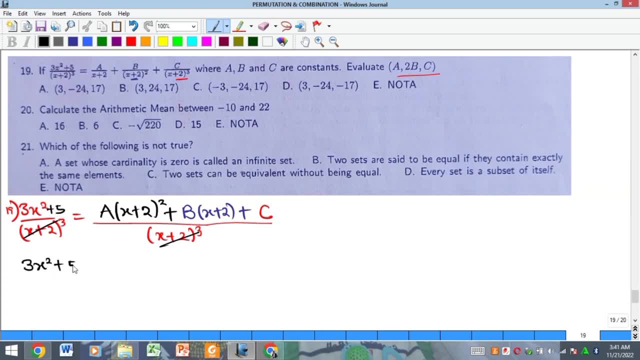 this is plus five. so what it means is: this is plus five. so what it means is that 3x squared plus 5 is equivalent to that. 3x squared plus 5 is equivalent to that. 3x squared plus 5 is equivalent to the numerator with of the right hand. 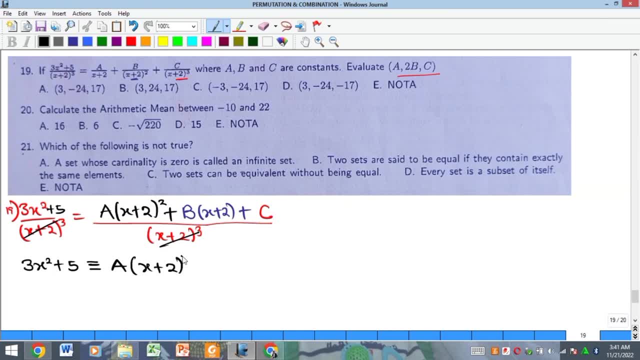 the numerator with of the right hand. the numerator with of the right hand side, which is a into x, squared x plus 2. side, which is a into x, squared x plus 2. side which is a into x squared x plus 2. r squared plus b into x plus. 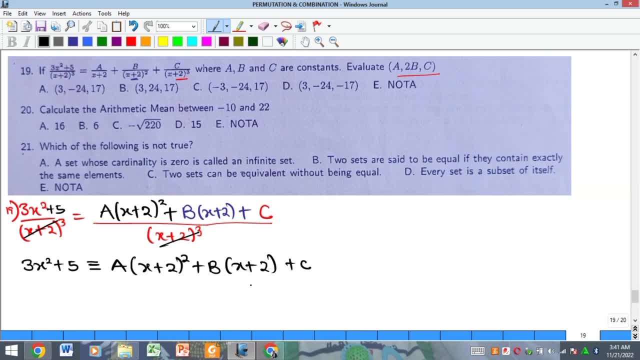 r squared plus b into x plus r. squared plus b into x plus 2, then plus c. so to be able to solve for 2, then plus c. so to be able to solve for 2, then plus c, so to be able to solve for my c. there are two methods i can use. 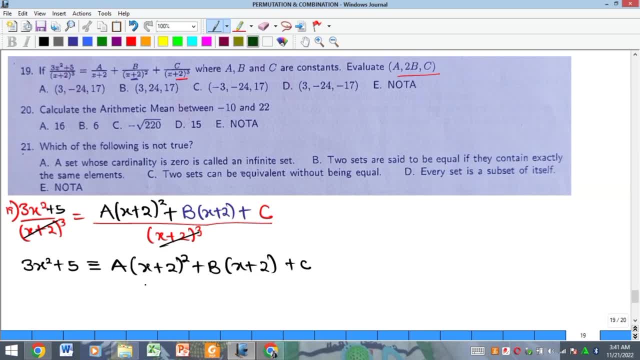 my c. there are two methods. i can use my c. there are two methods i can use here or abc- sorry, i can actually expand here. or abc- sorry, i can actually expand here or abc. sorry, i can actually expand and compare and compare and compare both sides. or i can use 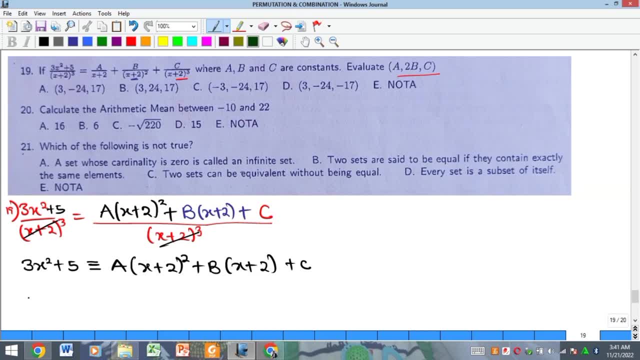 both sides, or i can use both sides or i can use the first. at least there is something i the first, at least there is something i the first, at least there is something i can do to get my c can do to get my c can do, to get my c very fast, and that is to let that's to. 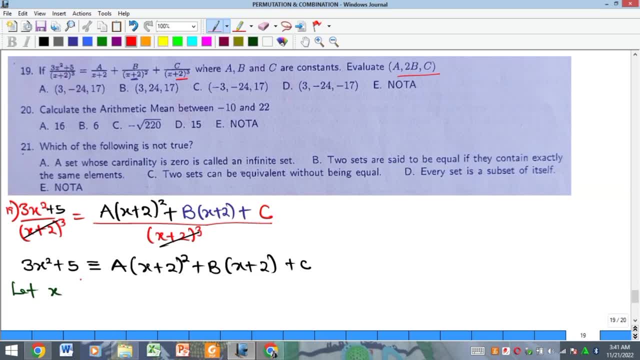 very fast, and that is to let that's to very fast, and that is to let that's to eliminate a and b. eliminate a and b, eliminate a and b. and if i want to eliminate a and b, i will, and if i want to eliminate a and b, i will. 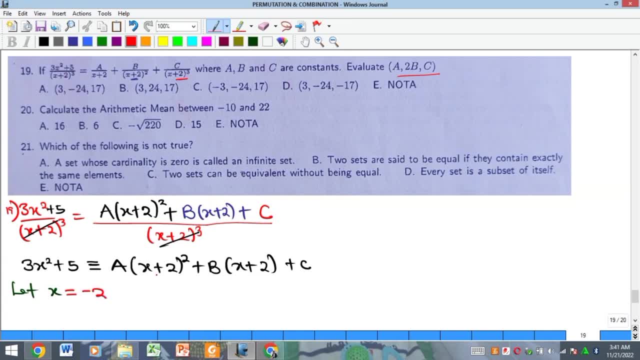 and if i want to eliminate a and b, i will make x, make x, make x minus 2, because if you put it here, you minus 2. because if you put it here, you minus 2. because if you put it here, you get zero, if you put it here, you get zero. 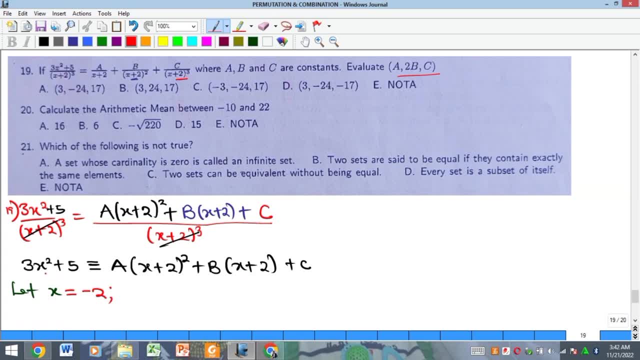 get zero. if you put it here, you get zero. get zero. if you put it here, you get zero. so let's do that substitute to the. so let's do that substitute to the. so let's do that substitute to the left hand side: x minus 2 squared. 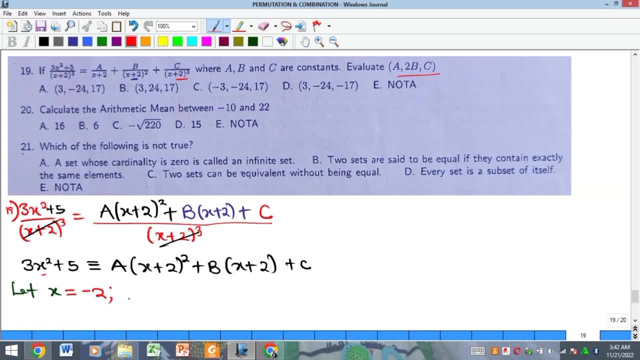 left hand side x minus 2 squared. left hand side x minus 2 squared will give us 4 4 times 3 is 12. 12 plus will give us 4. 4 times 3 is 12. 12 plus will give us 4. 4 times 3 is 12. 12 plus 5 is 17 and that is equal to now, if i 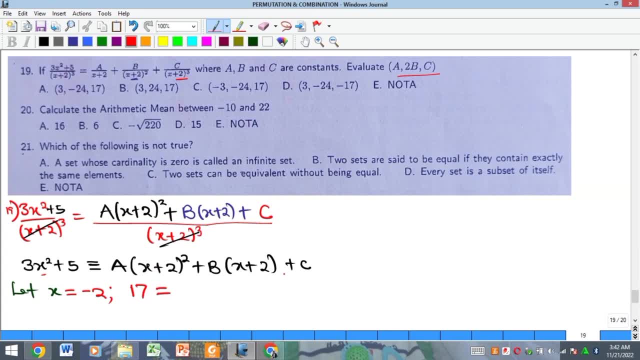 5 is 17, and that is equal to now. if i 5 is 17, and that is equal to now. if i put x minus 2 here, zero, zero, and then i put x minus 2 here, zero, zero, and then i put x minus 2 here, zero, zero, and then i just have that. my c is: 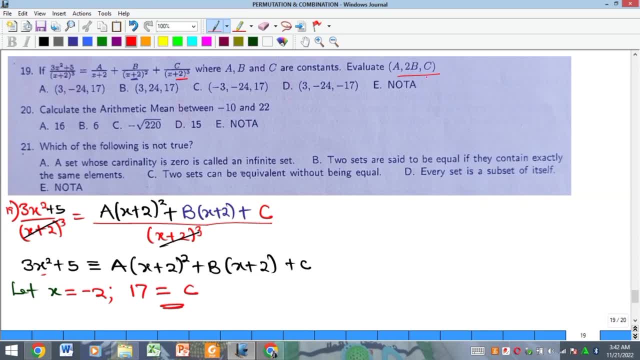 just have that. my c is: just have that. my c is that my c is 17, and so just a quick check that my c is 17, and so just a quick check that my c is 17, and so just a quick check. if you put 17 here, that means this guy. 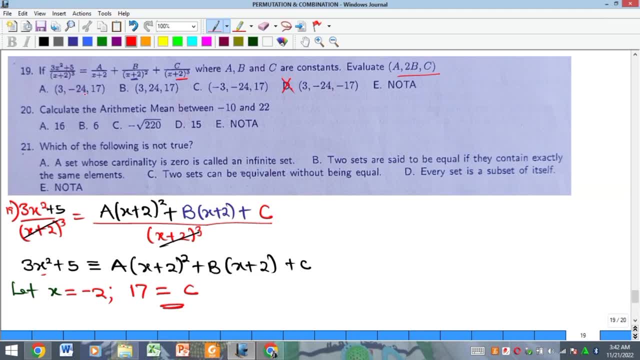 if you put 17 here, that means this guy. if you put 17 here, that means this guy is not going to be part of it. so i have is not going to be part of it. so i have is not going to be part of it. so i have 1770, so i would have to get. 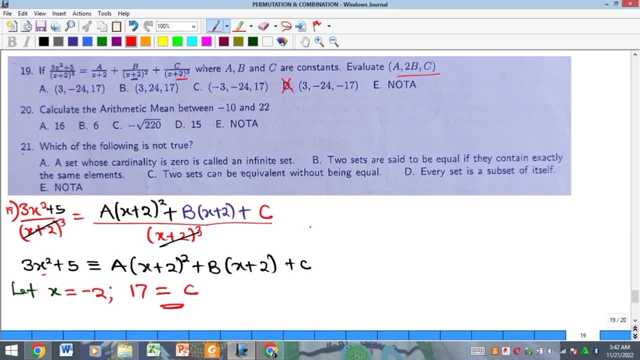 1770, so i would have to get 1770, so i would have to get from a b c. so let's go now. so at this from a b c. so let's go now. so at this from a b c, so let's go now. so at this point there is nothing else we can. 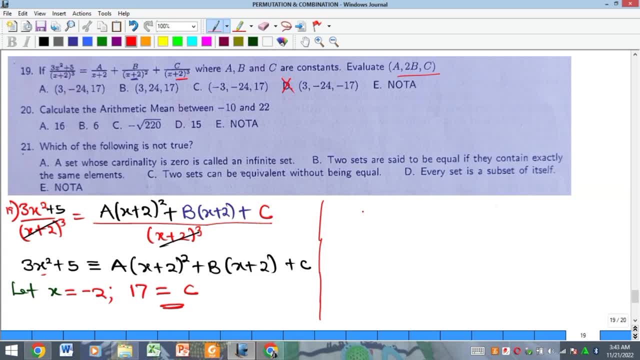 point, there is nothing else we can point, there is nothing else we can substitute, substitute, substitute. so okay, so one of the things we can, so okay, so one of the things we can, so okay, so one of the things we can also do here is just to expand now and 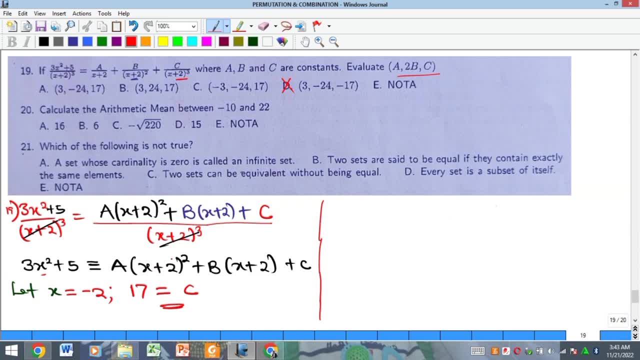 also do here is just to expand now, and also do here is just to expand now, and then substitute c, then substitute c, then substitute c. so if we expand this now, we're going to. so if we expand this now, we're going to. so if we expand this now, we're going to have 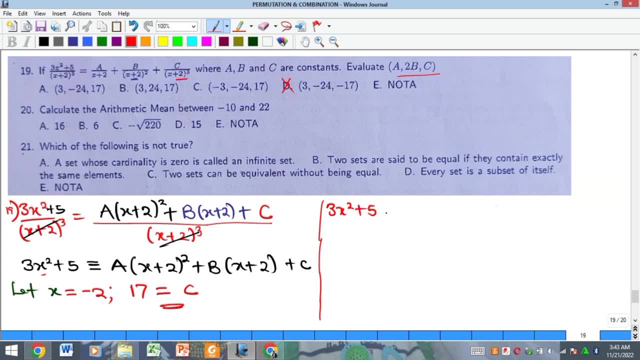 have have 3x squared plus 5. 3x squared plus 5. 3x squared plus 5 is equivalent to, is equivalent to, is equivalent to: and so i'm going to have a into the and so i'm going to have a into the. 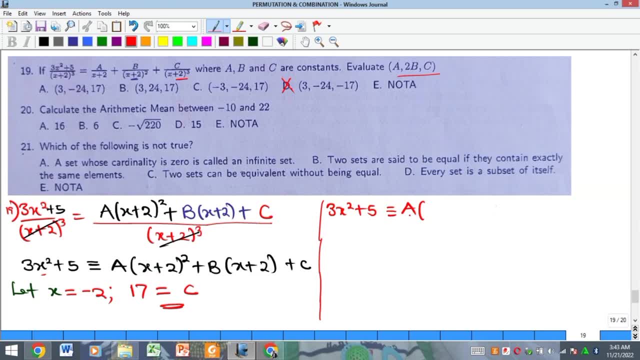 and so i'm going to have a into the bracket. if you expand bracket, if you expand bracket, if you expand x plus 2 squared, you will have x squared. x plus 2 squared, you will have x squared. x plus 2 squared, you will have x squared plus. 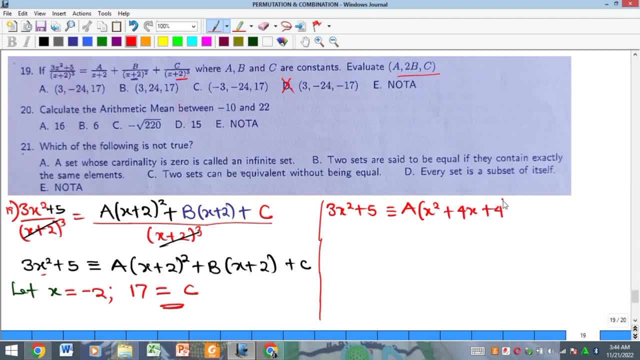 plus plus four x four x, four x plus four plus four plus four, and, and, and that is for the first one. then you now that is for the first one, then you- now that is for the first one. then you now have b, have b, have b x. that's opening the bracket plus 2b. 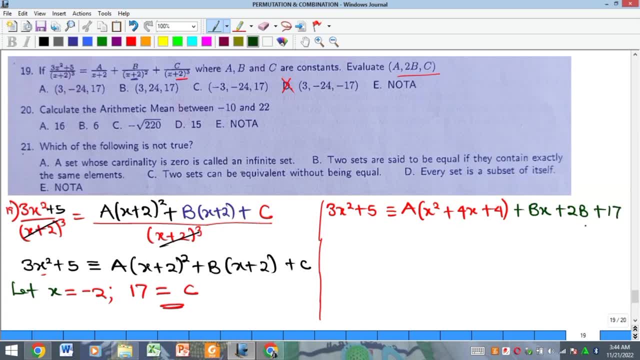 x, that's opening the bracket plus 2b. x, that's opening the bracket plus 2b plus c, which you have gotten now to be plus c, which you have gotten now to be plus c, which you have gotten now to be 17, 17. 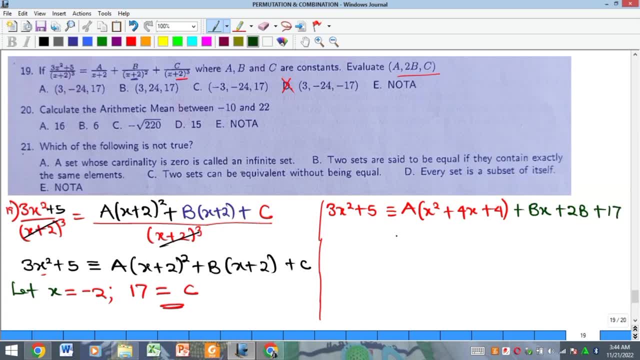 17, and so open this other side also, and so open this other side also, and so open this other side also. or let's leave that our c as what it is, or let's leave that our c as what it is, or let's leave that our c as what it is. let's leave it as c. 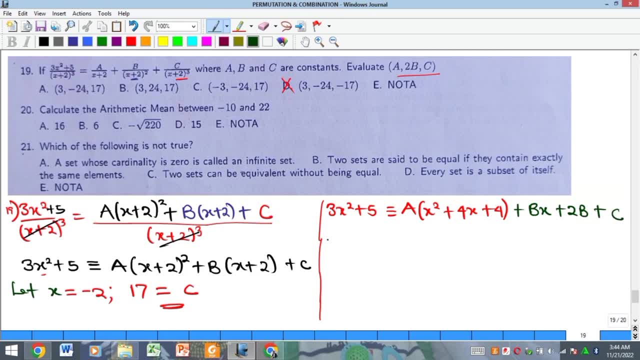 let's leave it as c, let's leave it as c, and so what we now have here now is going, and so what we now have here now is going, and so what we now have here now is going to be that this is equivalent to open, to be that this is equivalent to open. 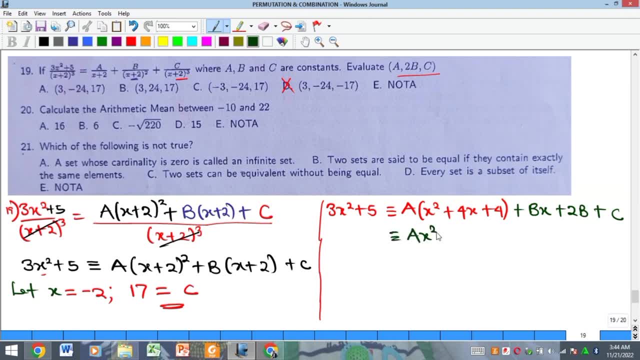 to be that this is equivalent to open this bracket. we'll have a x squared this bracket. we'll have a x squared this bracket. we'll have a x squared. then we now have four a x. then we now have four a x. then we now have four a x, then we'll have four a. 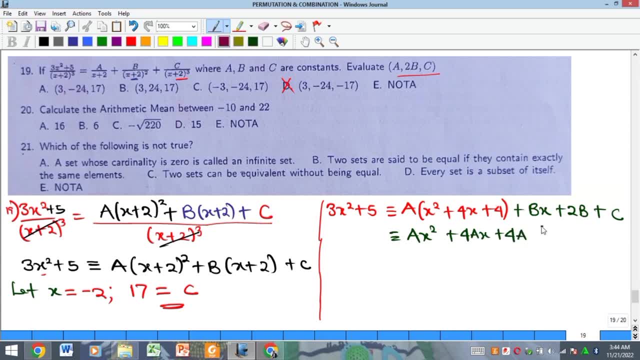 then we'll have four a, and that is plus, and that is plus, and that is plus our bx, our bx, our bx, then plus 2b, then plus 2b, then plus 2b, then plus c, then plus c, then plus c. okay, so if you compare both sides now, 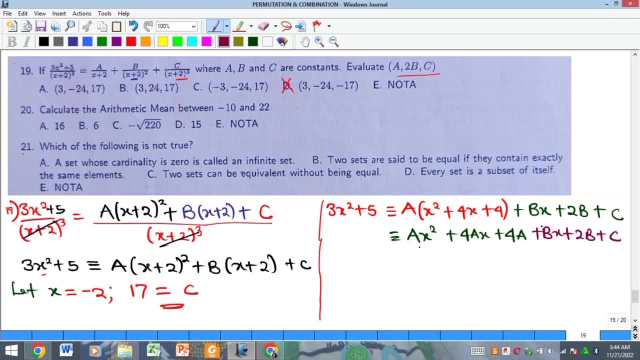 okay. so if you compare both sides now, okay. so if you compare both sides now, the only coefficient of x squared on the, the only coefficient of x squared on the, the only coefficient of x squared on the right hand side is a, and on the left right hand side is a and on the left. 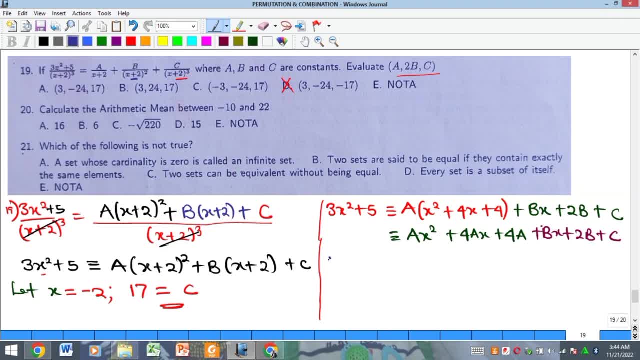 right hand side is a and on the left hand side is hand side is hand side is three. therefore, our a is equal to three. three therefore, our a is equal to three. three, therefore, our a is equal to three. so we have gotten a. we are now left with 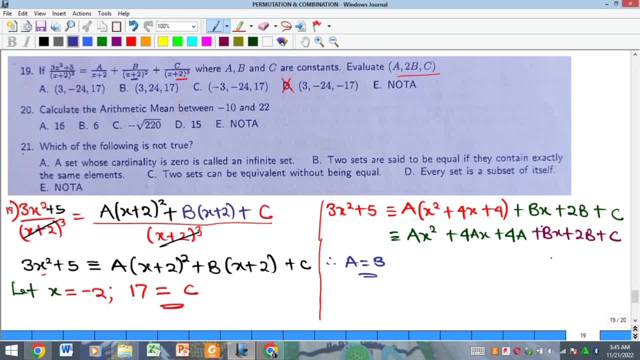 so we have gotten a we are now left with. so we have gotten a, we are now left with b. so for b, we can make use of either the b, so for b, we can make use of either the b, so for b, we can make use of either the constants or the coefficient of x. 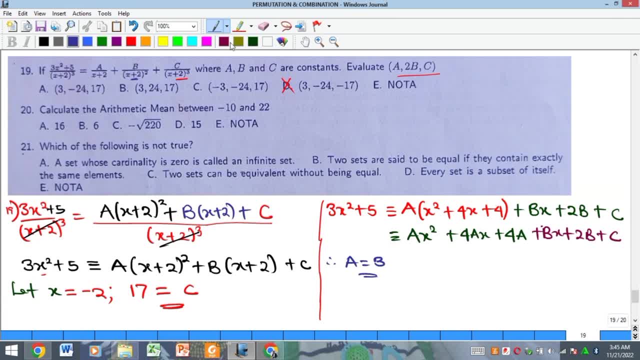 constants or the coefficient of x. constants or the coefficient of x? the coefficient of x on the right hand side, the coefficient of x on the right hand side, the coefficient of x on the right hand side, is: is is equal to look at it. join these two. equal to look at it. join these two. 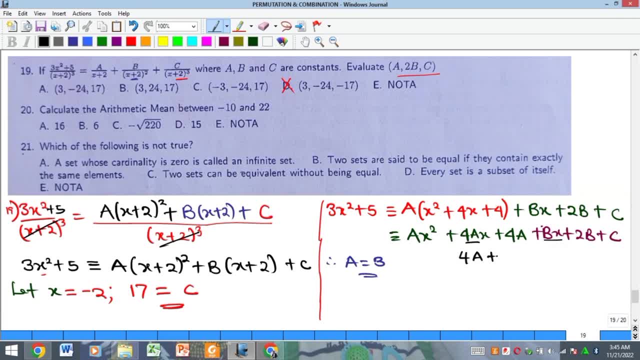 equal. to look at it, join these two. so you are going to have 4 a. so you are going to have 4 a. so you are going to have 4 a plus b, all into x plus b, all into x plus b, all into x. so the coefficient of b is 4 a plus b. 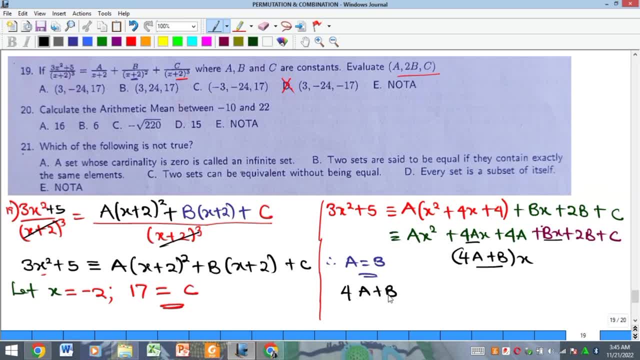 so the coefficient of b is 4 a plus b. so the coefficient of b is 4 a plus b. so 4 a plus b, so 4 a plus b. so 4 a plus b must be equal to the coefficient of x on must be equal to the coefficient of x on. 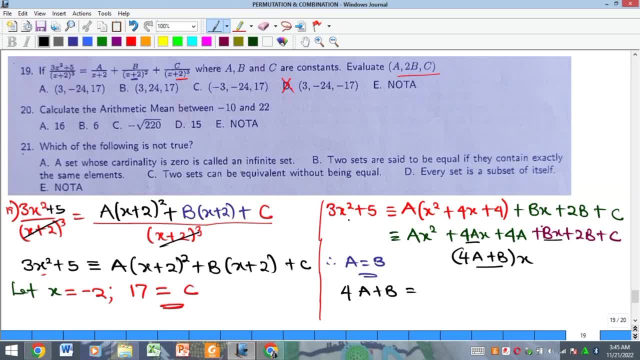 must be equal to the coefficient of x on the left hand side, the left hand side, the left hand side, and there's no x here. what it means is: and there's no x here. what it means is: and there's no x here. what it means is that the coefficient is what 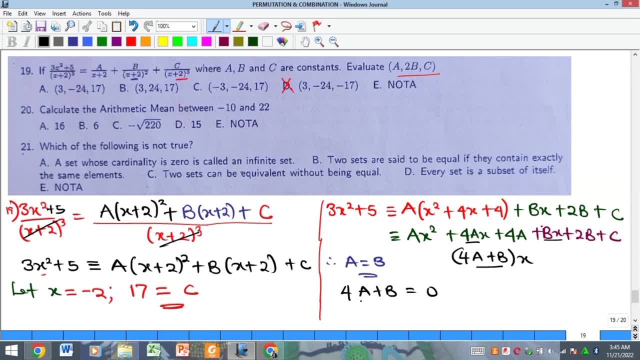 that the coefficient is what? that the coefficient is what? zero. and we already have our a as zero, and we already have our a as zero and we already have our a as three. that means three times four is three. that means three times four is three. that means three times four is twelve plus b. 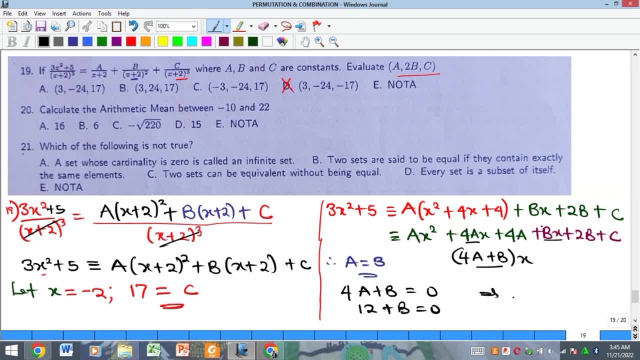 twelve plus b. twelve plus b is equal to zero. so the implication is is equal to zero. so the implication is is equal to zero. so the implication is that our b, that our b, that our b is negative 12.. okay, so now put is negative 12.. okay, so now put. 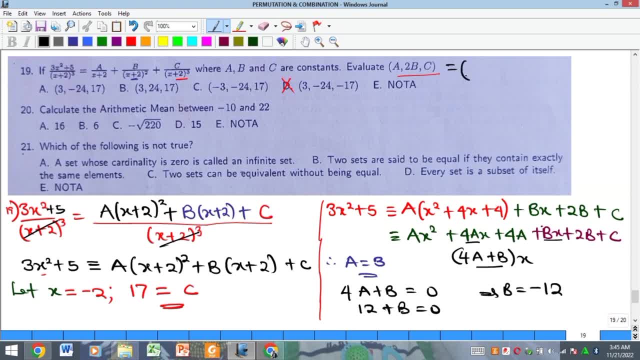 is negative 12.. okay, so now put everything here now. everything here now. everything here now. so it means that our a- let me use this. so it means that our a- let me use this. so it means that our a- let me use this, our a, our a. 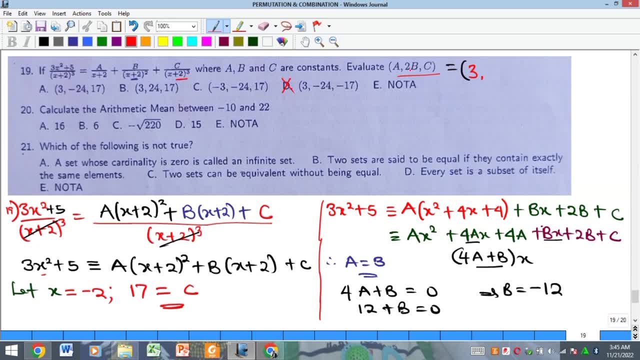 our a is three. our b is sorry. the next thing is three, our b is sorry, the next thing is three, our b is sorry. the next thing is: two times b, which is minus 24, is two times b, which is minus 24, is two times b, which is minus 24, and then you now have 17.. so let's come. 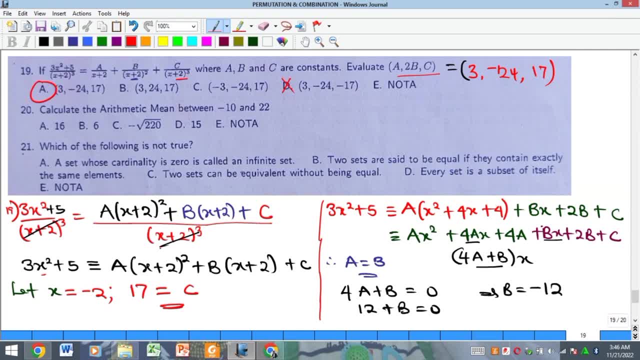 and then you now have 17.. so let's come, and then you now have 17.. so let's come here to check which one satisfies that, here, to check which one satisfies that, here to check which one satisfies that, and that is our option. a, okay, and then 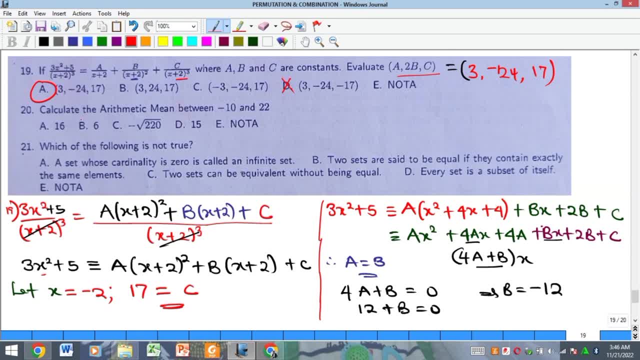 and that is our option- a okay, and then, and that is our option- a okay, and then. what about the next one? what about the next one? what about the next one? here, they said we should calculate the. here they said we should calculate the. here they said we should calculate the arithmetic mean. 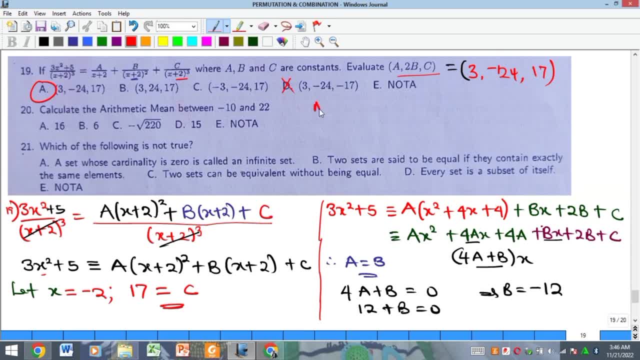 arithmetic mean, arithmetic mean of this arithmetic mean is simply of this: arithmetic mean is simply of this: arithmetic mean is simply equal to the sum of the two divided by, equal to the sum of the two divided by, equal to the sum of the two divided by two. so you have minus 10 plus 22. 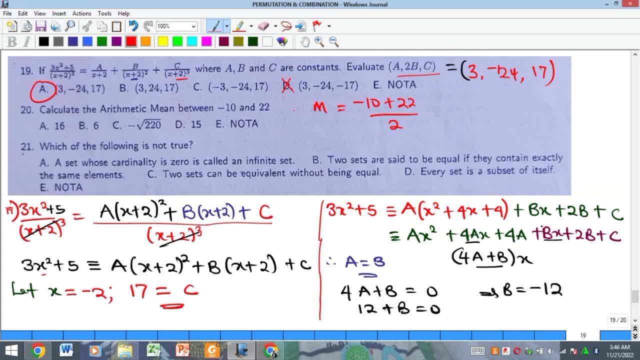 two. so you have minus 10 plus 22 two. so you have minus 10 plus 22 all over two. so you sum and divide by all over two. so you sum and divide by all over two. so you sum and divide by their number, their number. 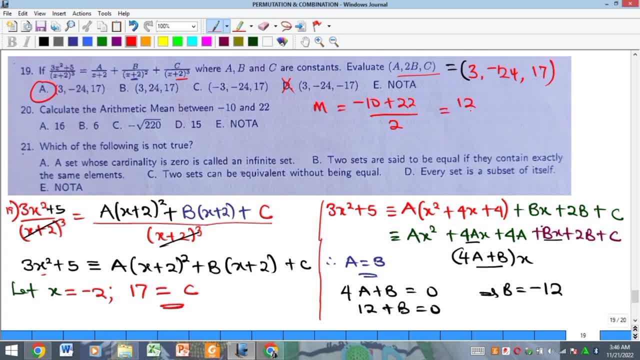 their number, and this is going to give us uh 12 all, and this is going to give us uh 12 all, and this is going to give us uh 12 all over two, which is equal to six over two, which is equal to six over two, which is equal to six. and that is option b, and so we go to. 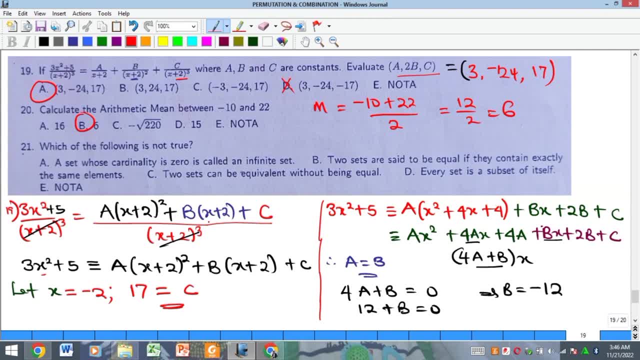 and that is option b, and so we go to, and that is option b, and so we go to. this is just a, this is just a, this is just a. a knowledge question: asking you to a knowledge question, asking you to a knowledge question, asking you to, uh, state which one is not true. 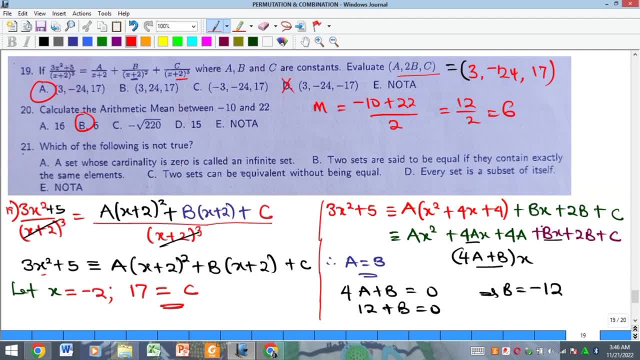 uh state which one is not true. uh, state which one is not true. unless read a set whose cardinality is, unless read a set whose cardinality is, unless read a set whose cardinality is zero is called an infinite set. this is zero is called an infinite set. this is. 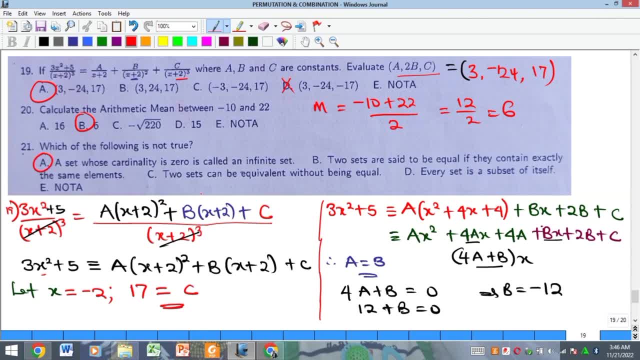 zero is called an infinite set. this is, of course, not true. of course not true. of course not true. and that is your answer. because if the? and that is your answer, because if the? and that is your answer. because if the cardinality of a set is zero, it means 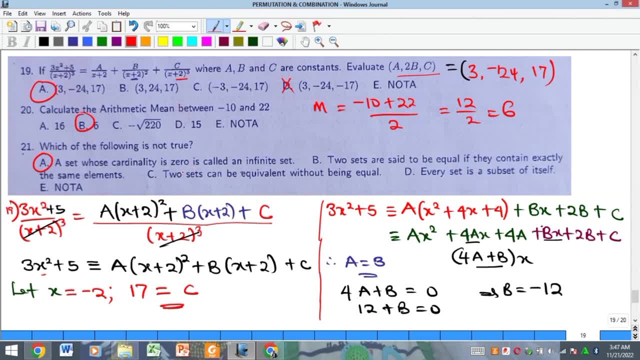 cardinality of a set is zero. it means cardinality of a set is zero. it means it's not set. so you can actually determine it's not set. so you can actually determine it's not set, so you can actually determine the cardinality is part of the definition. 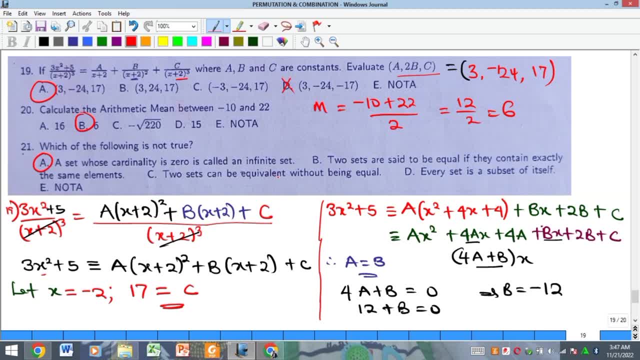 the cardinality is part of the definition. the cardinality is part of the definition. an infinite set is a set that you cannot. an infinite set is a set that you cannot. an infinite set is a set that you cannot. determine the number of elements so that. determine the number of elements, so that. 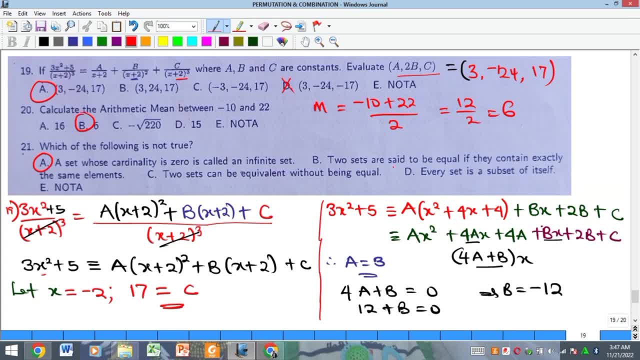 determine the number of elements. so that means, means, means. this is not true. you can check the next. this is not true. you can check the next. this is not true. you can check the next. one. two sets are said to be equal. one. two sets are said to be equal. 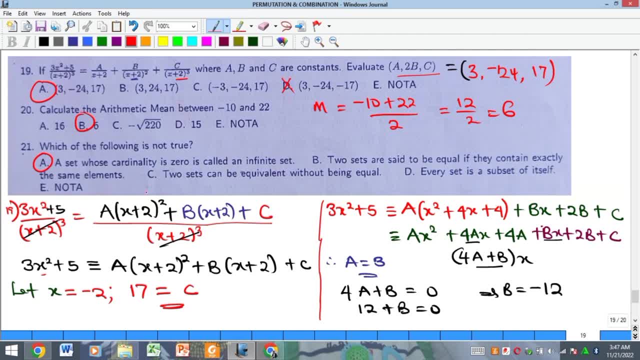 one. two sets are said to be equal if they contain exactly the same elements, if they contain exactly the same elements, if they contain exactly the same elements. that is true, that is true. that is true. two sets can be equivalent without being. two sets can be equivalent without being. 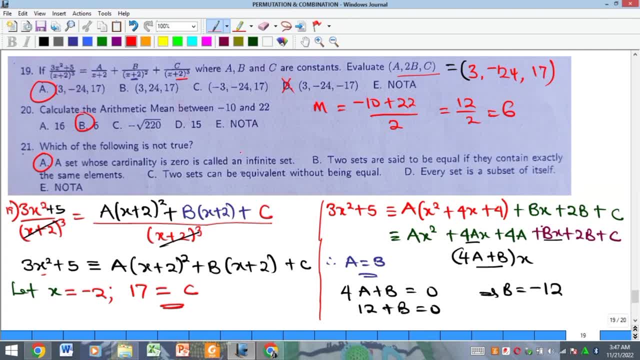 two sets can be equivalent without being equal. that is true. equal, that is true. equal, that is true. you can have two cells that have the same. you can have two cells that have the same. you can have two cells that have the same number of element. that's equivalent. 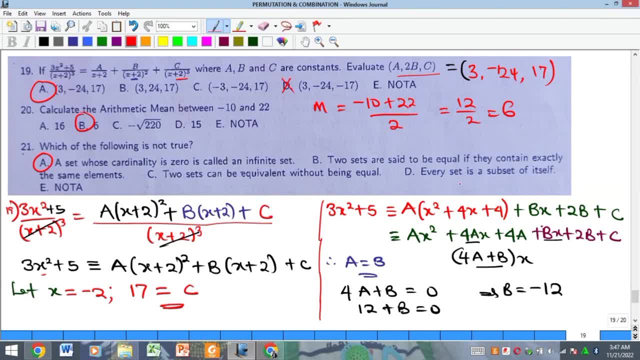 number of element that's equivalent. number of element that's equivalent and yet not equal. yes, so every set is a, and yet not equal. yes, so every set is a, and yet not equal. yes, so every set is a subset of itself. that's also true, so, subset of itself, that's also true, so. 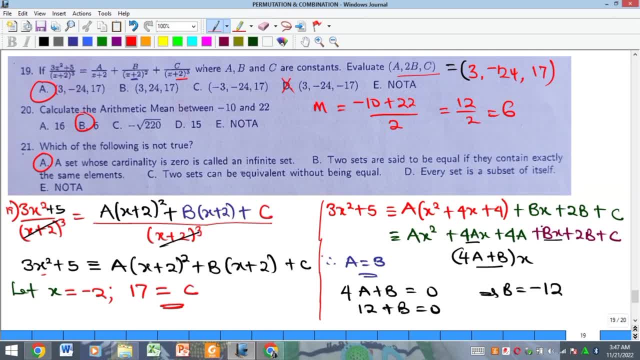 subset of itself. that's also true. so only a, only a, only a is the option that is not true for number. is the option that is not true for number. is the option that is not true for number: 21, 21, 21, okay and um, okay, so we quickly go to the. 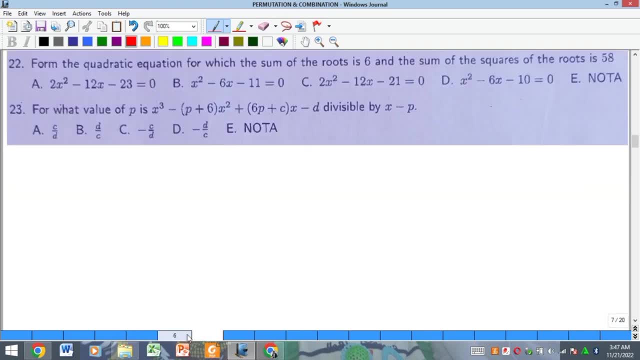 okay and um okay, so we quickly go to the okay and um okay, so we quickly go to the next one, which is next one, which is next one, which is number 22, and here it says number 22, and here it says number 22, and here it says solution. so for 22, we are asked to form. 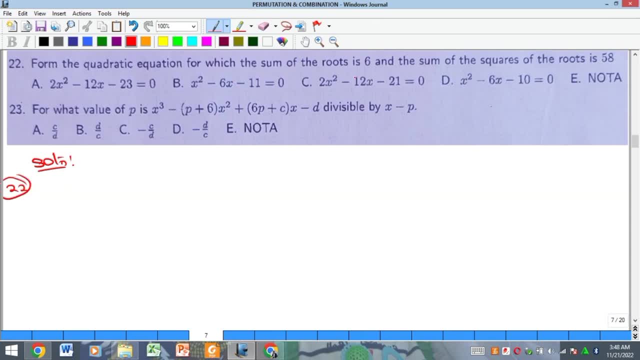 solution. so for 22, we are asked to form solution. so for 22, we are asked to form a quadratic equation for which the sum: a quadratic equation for which the sum: a quadratic equation for which the sum of uh, of uh, of uh, the sum of the roots, is six. so let the 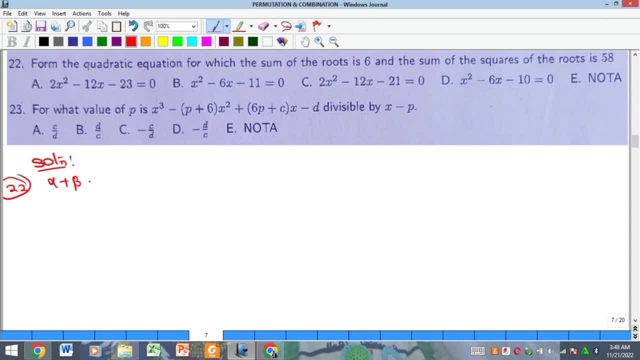 the sum of the roots is six, so let the. the sum of the roots is six, so let the roots be alpha, roots be alpha, roots be alpha and beta, so the sum is equal to six and beta. so the sum is equal to six and beta. so the sum is equal to six. and then the sum of their squares, that's. 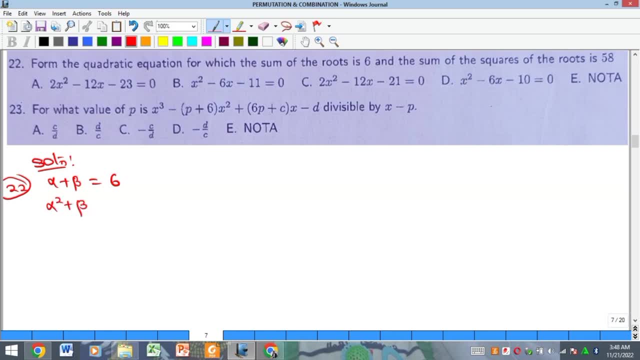 and then the sum of their squares, that's: and then the sum of their squares, that's alpha squared. alpha squared. alpha squared, the squares of the roots plus beta, the squares of the roots plus beta, the squares of the roots plus beta squared, is equal to 58. 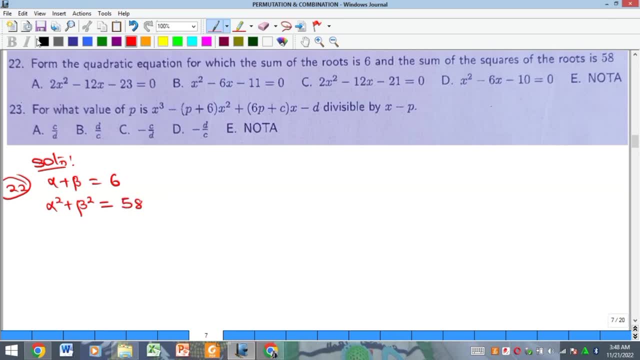 squared is equal to 58. squared is equal to 58. okay, now remember that. okay, now remember that. okay, now remember that. we are told that every, we are told that every, we are told that every quadratic equation is of this form x. quadratic equation is of this form x. 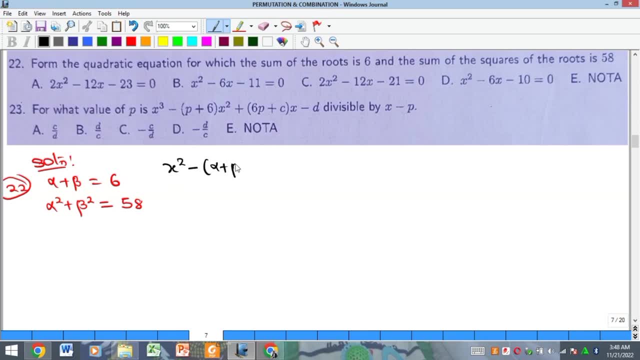 quadratic equation is of this form: x squared minus alpha plus beta, squared minus alpha plus beta. squared minus alpha plus beta, that's the two roots assuming the roots. that's the two roots assuming the roots. that's the two roots assuming the roots are alpha and beta. are alpha and beta. 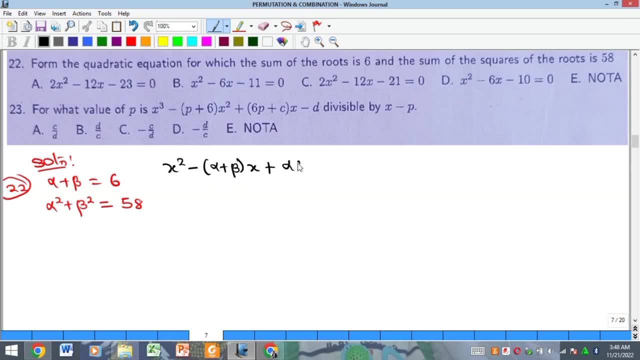 are alpha and beta times x, then plus alpha beta times x, then plus alpha beta times x, then plus alpha beta, and that is equal to zero. there's a and that is equal to zero. there's a and that is equal to zero. there's a general formula for quadratic equations. 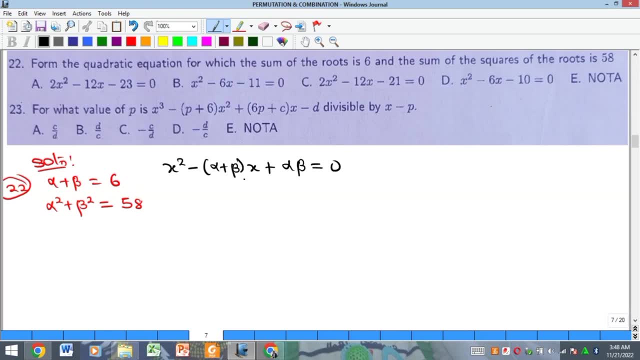 general formula for quadratic equations: general formula for quadratic equations. that is of this form. so all we need to do that is of this form. so all we need to do, that is of this form. so all we need to do now we already have this. that's the. 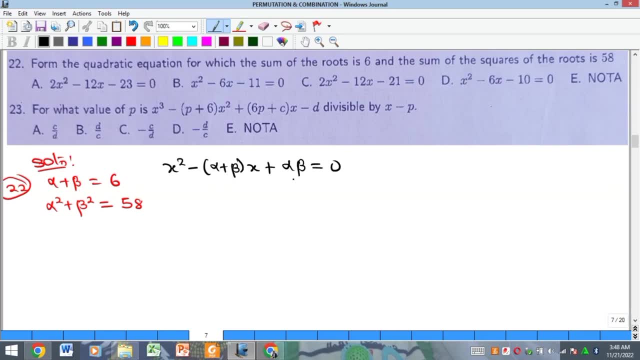 now we already have this. that's the. now we already have this. that's the coefficient of bx, coefficient of bx, coefficient of bx, and so we need to get alpha beta number and so we need to get alpha beta number, and so we need to get alpha beta number. recall that. 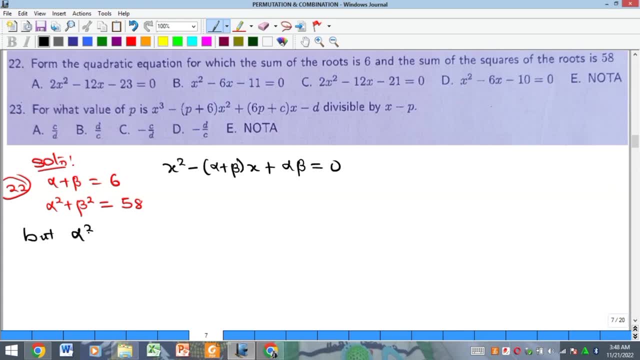 recall that, recall that we have that, our alpha squared plus. we have that, our alpha squared plus. we have that our alpha squared plus beta, squared by symmetric properties of beta, squared by symmetric properties of beta, squared by symmetric properties of roots, roots, roots, is actually equal to alpha plus beta. 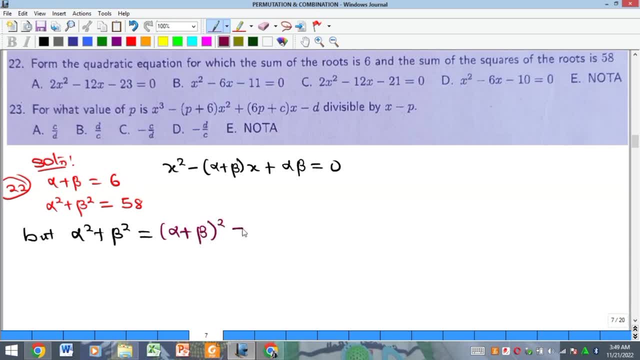 is actually equal to alpha plus beta, is actually equal to alpha plus beta. r squared r squared r squared minus minus minus. so all you need to do now is to substitute. so all you need to do now is to substitute. so all you need to do now is to substitute our values. 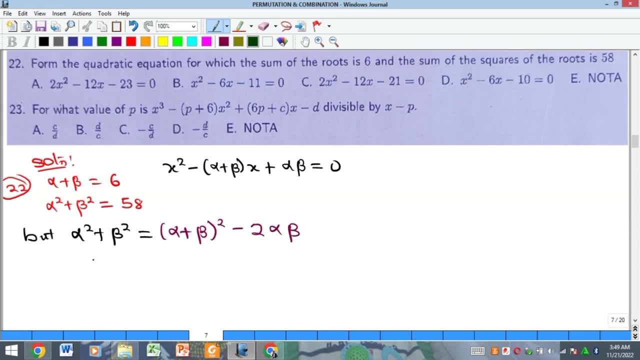 our values, our values. so i have got. i was given that alpha, so i have got. i was given that alpha, so i have got. i was given that alpha squared plus beta squared is 58 squared plus beta squared is 58 squared plus beta squared is 58, and so that is equal to alpha plus beta. 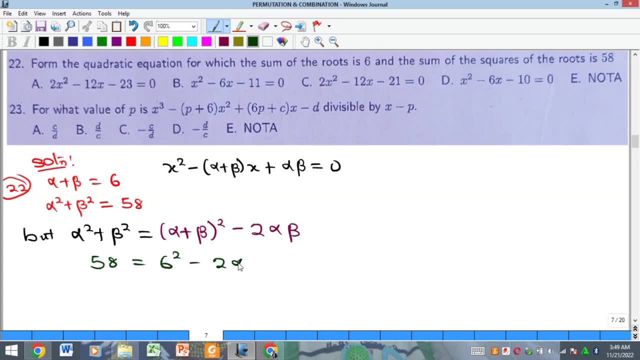 and so that is equal to alpha plus beta, and so that is equal to alpha plus beta is six squared is six squared is six squared minus two alpha beta. and so this is uh minus two alpha beta. and so this is uh minus two alpha beta. and so this is uh. so take this to this side and bring this. 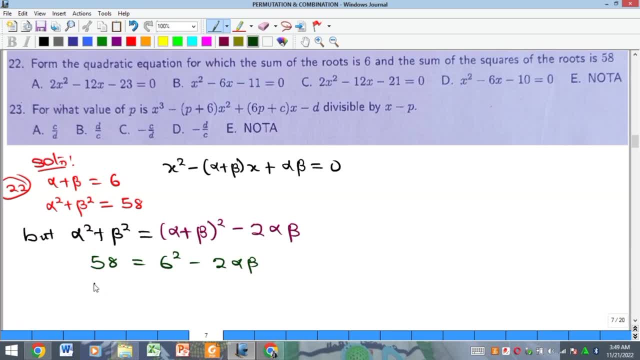 so take this to this side and bring this. so take this to this side and bring this to this side. so if this one comes here to this side and bring this to this side, it becomes positive two alpha beta. it becomes positive two alpha beta. it becomes positive two alpha beta, and that is equal to 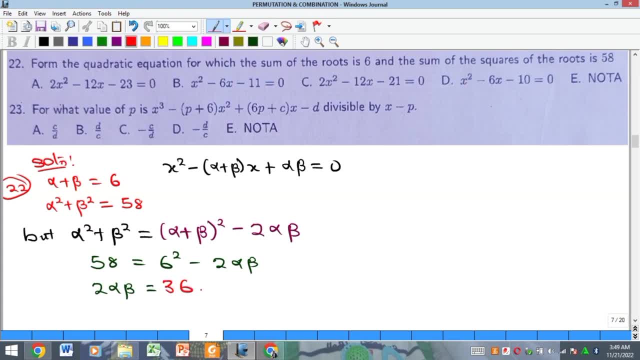 and that is equal to, and that is equal to: six squared is 36. six squared is 36, six squared is 36: 58 coming here will become minus 58. 58 coming here will become minus 58. 58 coming here will become minus 58, and so that is going to give me that my 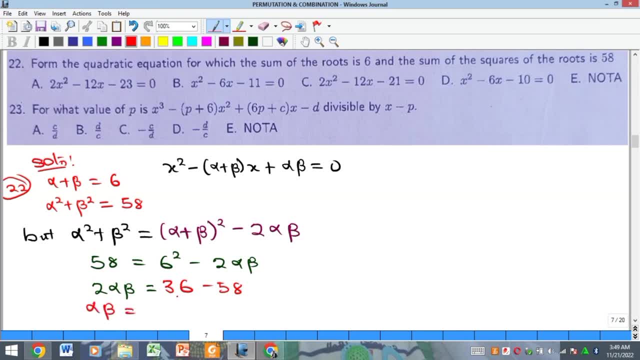 and so that is going to give me that my and so that is going to give me that my alpha beta, alpha beta, alpha beta is equal to this minus. this is going to is equal to this minus. this is going to is equal to this minus. this is going to be equal to negative 22. 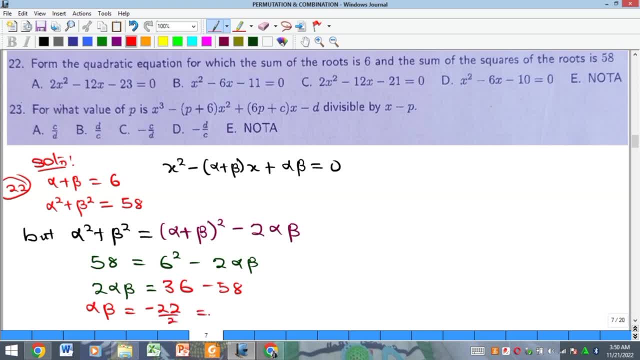 be equal to negative 22, be equal to negative 22, and so when you divide by 2, you have, and so when you divide by 2, you have, and so when you divide by 2, you have minus 11. therefore, the equation we are minus 11. therefore, the equation we are: 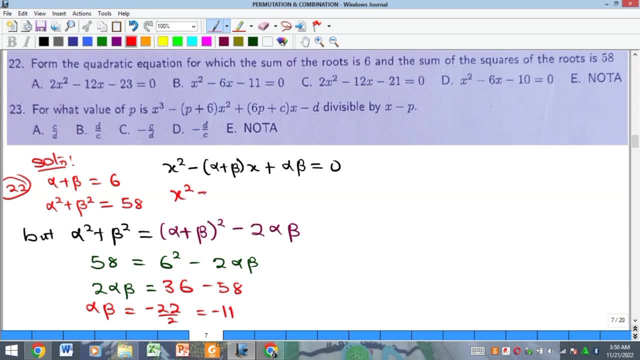 minus 11. therefore, the equation we are looking for is simply x squared minus. looking for is simply x squared minus. looking for is simply x squared minus. the whole of this is 6, which is given. the whole of this is 6, which is given. the whole of this is 6, which is given here. 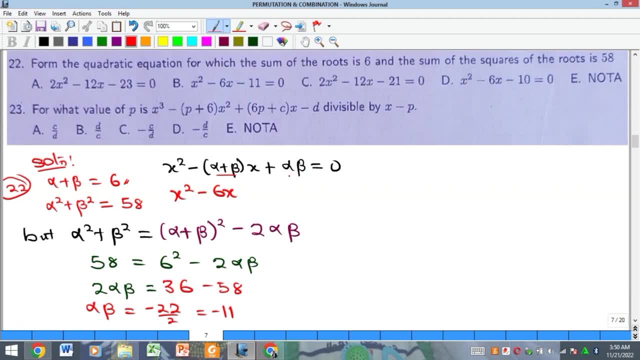 here, here, and then attach your x then the whole of, and then attach your x then the whole of, and then attach your x then the whole of this, which is this, which is this: which is: alpha beta is minus 11 from what we have. alpha beta is minus 11 from what we have. 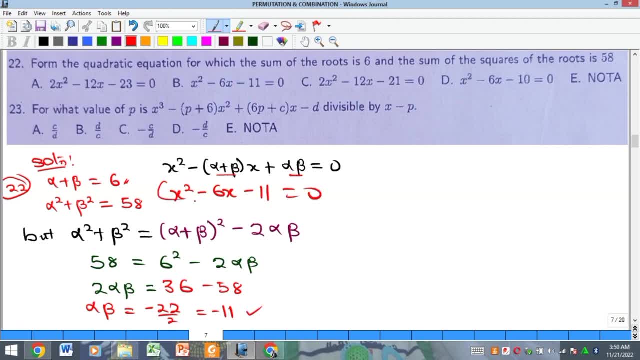 alpha beta is minus 11 from what we have here here, here, and everything is equal to zero, and so, and everything is equal to zero, and so, and everything is equal to zero, and so that is what we have as option b. that is what we have as option b. 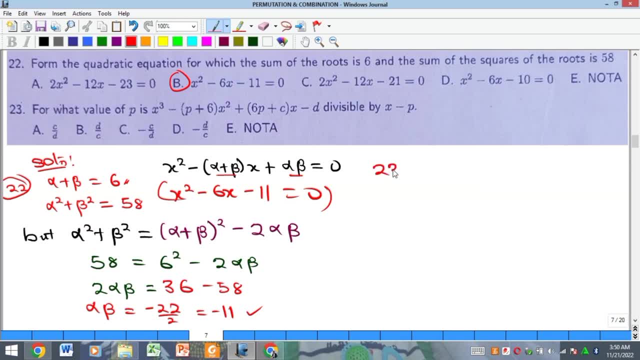 that is what we have as option b, and that's the solution. so we go to the and that's the solution. so we go to the and that's the solution. so we go to the next one, number 23, next one number 23, next one, number 23, which is also from polynomials, and. 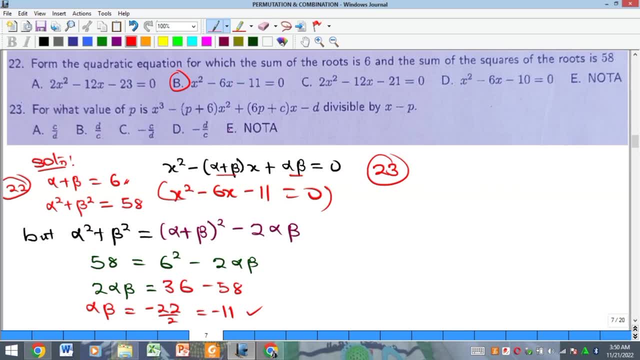 which is also from polynomials and which is also from polynomials and particularly from, particularly from, particularly from factor theorem and it says for what value factor theorem and it says for what value factor theorem and it says for what value of p, of p, of p, will this particular polynomial be. 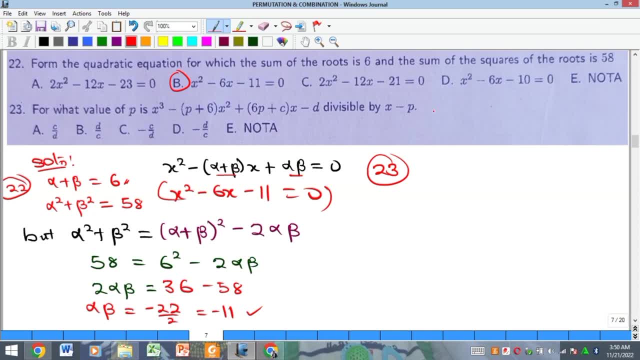 will this particular polynomial be? will this particular polynomial be divisible by divisible by divisible by x minus p? for this, just equate this to x minus p. for this, just equate this to x minus p. for this, just equate this to zero and get your x. 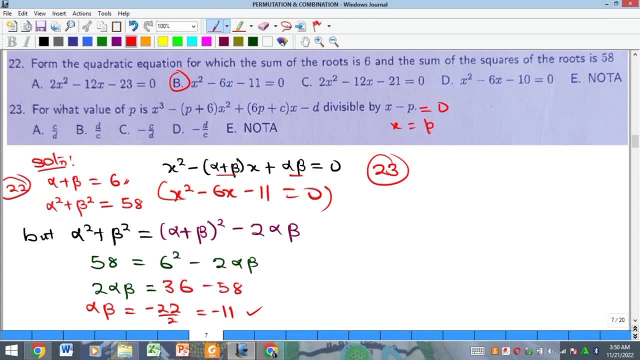 zero and get your x zero and get your x. therefore, our x is equal to p. so therefore, our x is equal to p. so therefore, our x is equal to p. so substitute this x into this, substitute this x into this, substitute this x into this, and by factor theorem, if you do this, 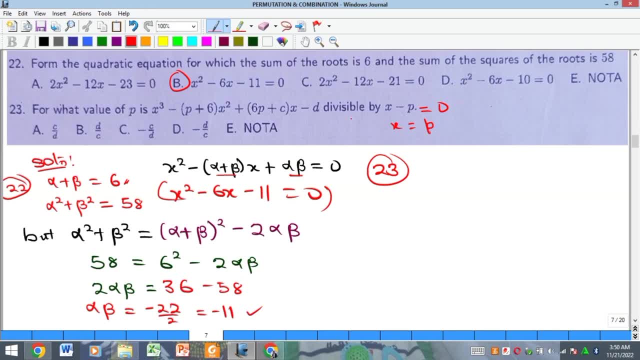 and by factor theorem. if you do this, and by factor theorem, if you do this, substitution, substitution, substitution- your value must be equal to zero. so when your value must be equal to zero, so when your value must be equal to zero, so when we get zero, we then solve for our p. 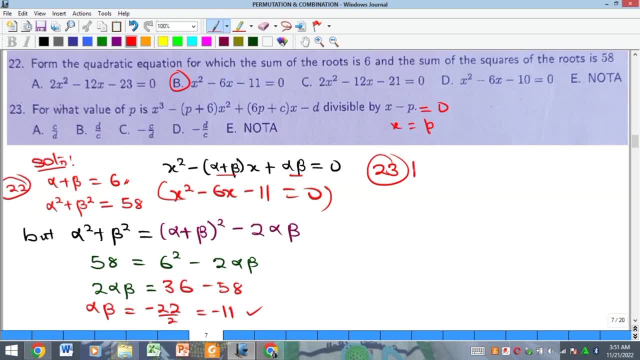 we get zero, we then solve for our p. we get zero, we then solve for our p. so let's do that. so i'm going to put. so let's do that. so i'm going to put. so let's do that. so i'm going to put: anywhere i see x, i'll put it as p, so i'll. 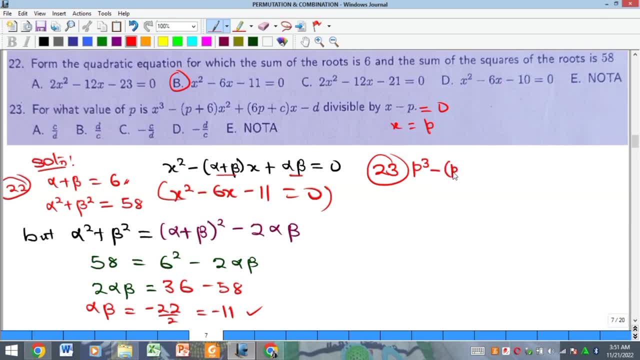 anywhere i see x, i'll put it as p. so i'll. anywhere i see x, i'll put it as p. so i'll have p cube minus p plus six. have p cube minus p plus six. have p cube minus p plus six, then x now is also p plus p squared. 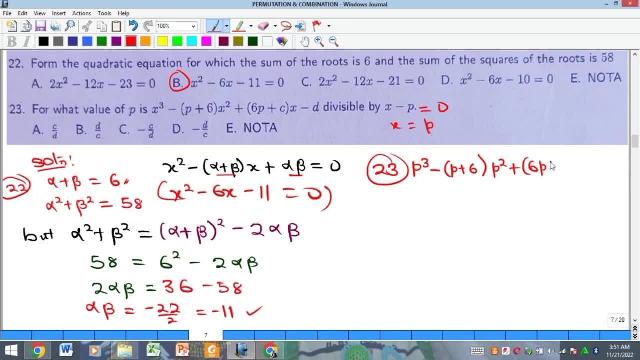 then x now is also p plus p squared, then x now is also p plus p squared into 6 p plus c, into 6 p plus c, into 6 p plus c. my x, there is p, then minus d. my x, there is p, then minus d. 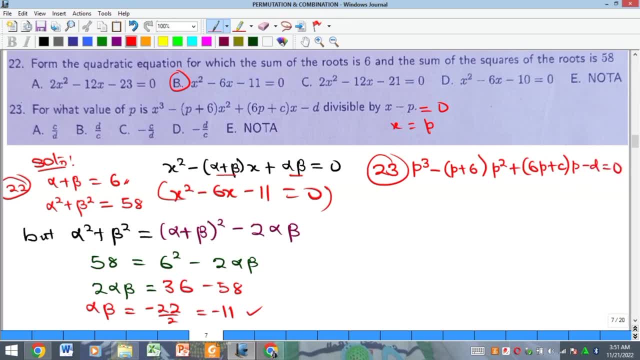 my x, there is p, then minus d, all equal to zero by factor theory. so all equal to zero by factor theory. so all equal to zero by factor theory. so what this means is that i am going to. what this means is that i am going to. what this means is that i am going to have 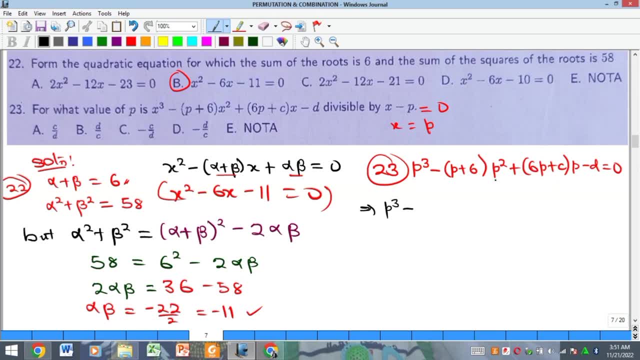 have have: just expand all the brackets. then p just expand all the brackets, then p just expand all the brackets, then p times. this is going to times. this is going to times. this is going to give me p cubed. then i'm opening from: give me p cubed, then i'm opening from: 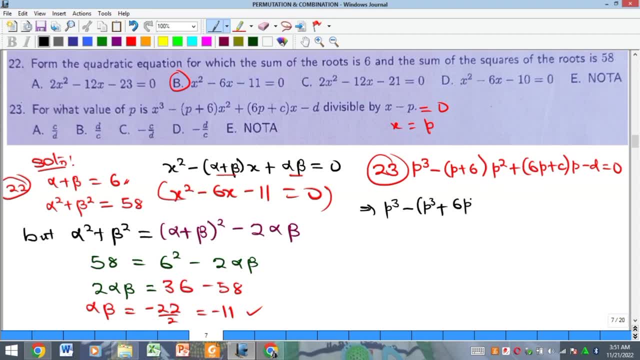 give me p cubed, then i'm opening from the right first, the right first, the right first. then 6 times p squared is also p squared. then 6 times p squared is also p squared, then 6 times p squared is also p squared. then i can open this one straight ahead. 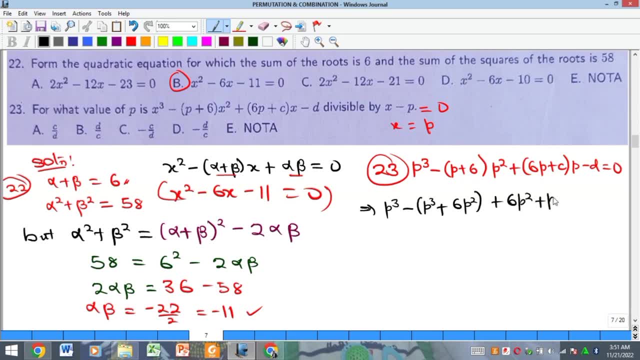 then i can open this one straight ahead, then i can open this one straight ahead. so i have 6 p squared. so i have 6 p squared. so i have 6 p squared plus pc. i did this because there is minus plus pc. i did this because there is minus. 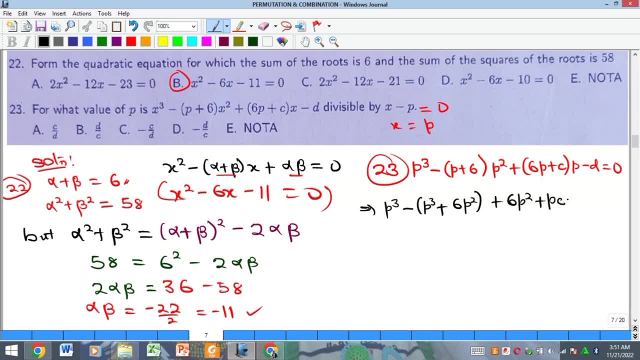 plus pc. i did this because there is minus here. so you open from the right and from here. so you open from the right and from here. so you open from the right and from the left, the left, the left. but in this case it's just positive. but in this case it's just positive. 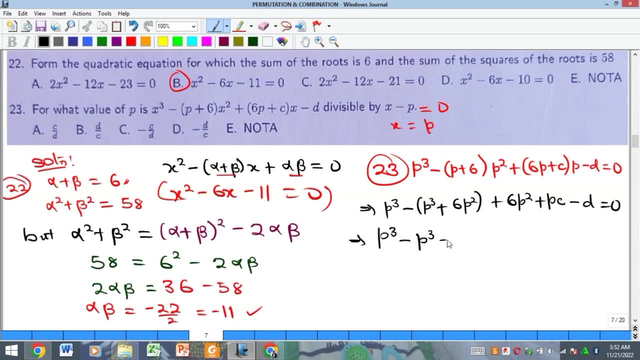 but in this case it's just positive. minus p cube, then minus times. this is minus p cube, then minus times. this is minus p cube, then minus times. this is also minus 6p squared, and that is plus. also minus 6p squared, and that is plus. 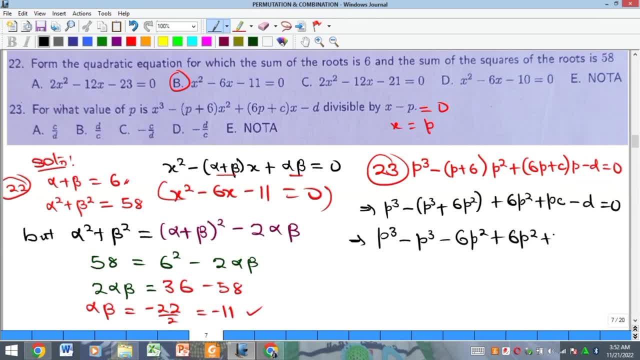 also minus 6p squared, and that is plus 6p squared, and that is plus pc 6p squared, and that is plus pc 6p squared, and that is plus pc minus d equal to zero. okay, so finally. minus d equal to zero. okay, so finally. 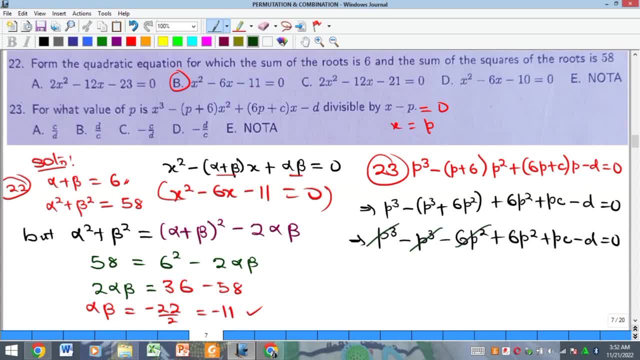 minus d equal to zero. okay, so, finally, you can see that this will take away, you can see that this will take away. you can see that this will take away this. this will take away this. so we only this. this will take away this. so we only this. this will take away this. so we only have. 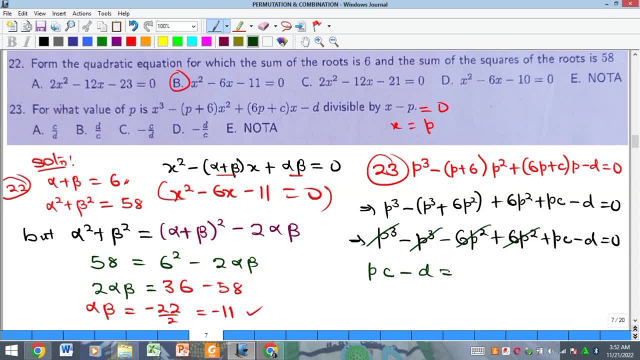 have. have pc minus d to be equal to zero, pc minus d to be equal to zero, pc minus d to be equal to zero. take that to the other side, so pc is. take that to the other side, so pc is. take that to the other side, so pc is equal to d. 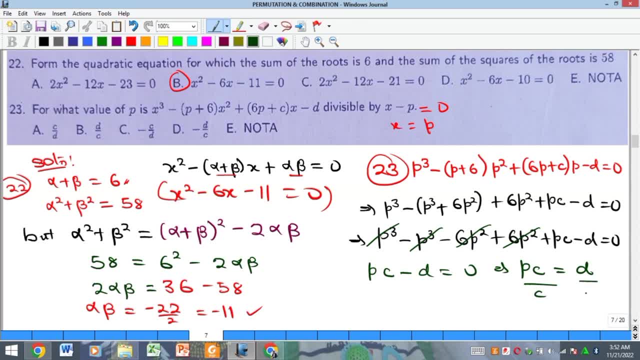 equal to d. equal to d. so divide both sides by c to get your p. so divide both sides by c to get your p. so divide both sides by c to get your p. that's what they asked you for. that's what they asked you for. that's what they asked you for. therefore, our p is equal to d, all over. 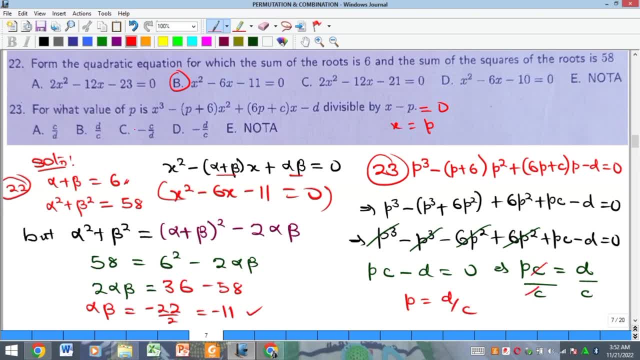 therefore, our p is equal to d all over. therefore, our p is equal to d all over c. of course this will take away this c. of course, this will take away this c. of course, this will take away this. and that is somewhere here. option, and that is somewhere here. option. 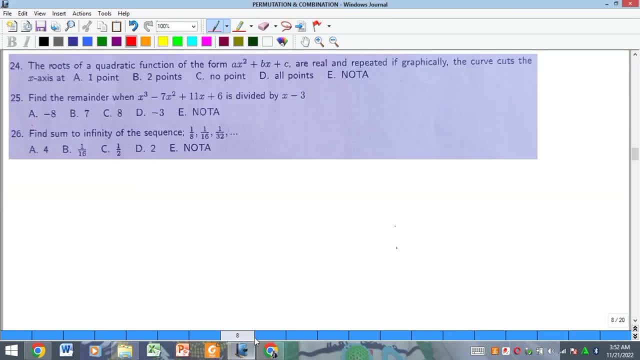 and that is somewhere here, option b. so we go to the next one, number 24 b. so we go to the next one, number 24 b. so we go to the next one, number 24, which is asking us: uh 24 says: which is asking us, uh 24 says: 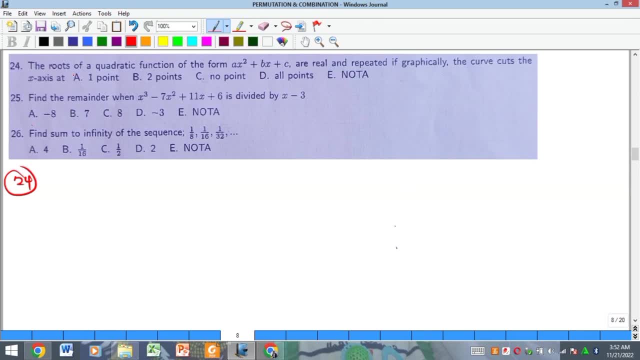 which is asking us: uh. 24 says that we should uh that the roots of a, that we should uh that the roots of a, that we should uh that the roots of a quadratic function, quadratic function, quadratic function of the form. this are real and repeated of the form. this are real and repeated. 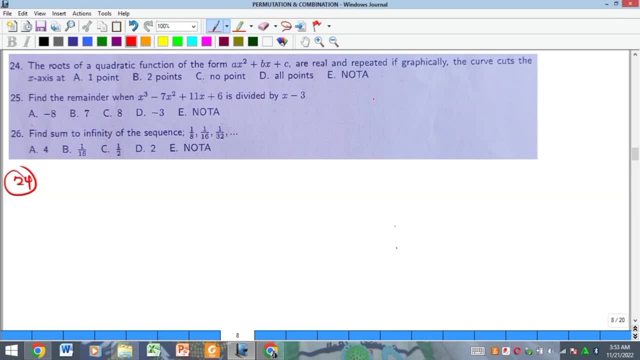 of the form, this are real and repeated. if graphically the curve cuts, okay. so if graphically the curve cuts, okay. so if graphically the curve cuts, okay. so you recall that, you recall that, you recall that we, we have also seen this, even on this, we, we have also seen this, even on this. 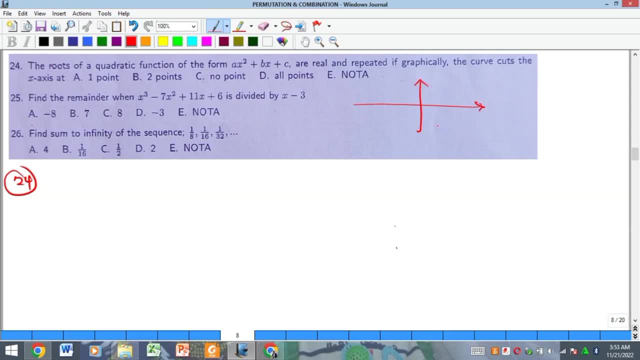 we. we have also seen this even on this channel. you can also watch channel. you can also watch channel. you can also watch that is under types of roots or forms of. that is under types of roots or forms of. that is under types of roots or forms of roots. i've explained that. so this is our. 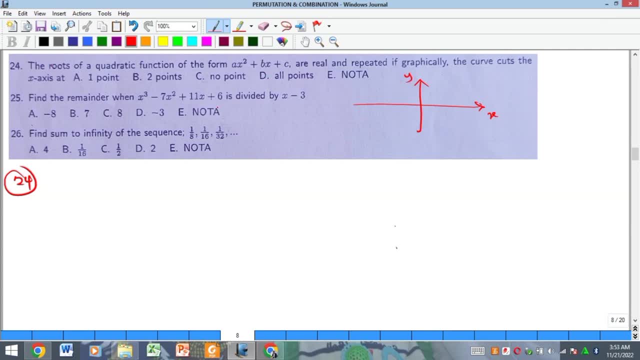 roots. i've explained that. so this is our roots. i've explained that. so this is our y axis. this is our x axis for you to y axis. this is our x axis for you to y axis. this is our x axis for you to have a. have a. 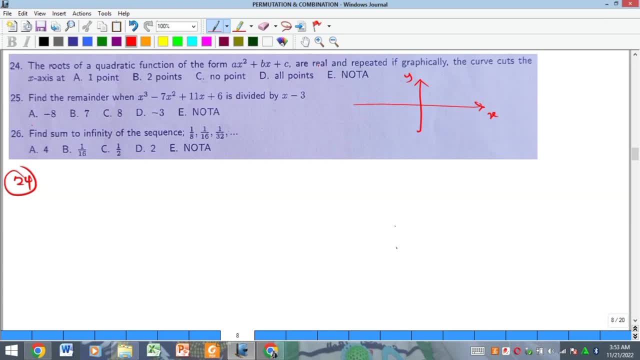 have a real and repeated roots. real roots means real and repeated roots. real roots means real and repeated roots. real roots means that it will touch the x as is repeated, that it will touch the x as is repeated. that it will touch the x as is repeated means it will touch it. 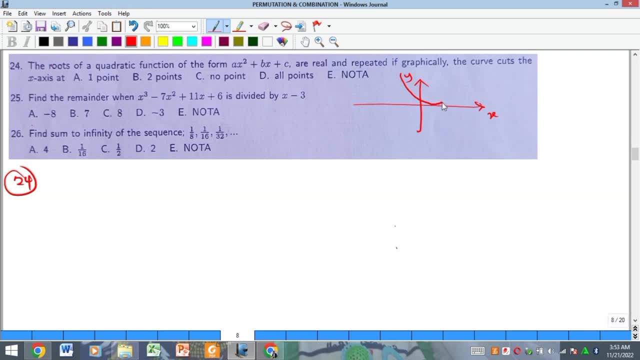 means it will touch it means it will touch it just at a point, something like this, just at a point, something like this, just at a point, something like this: okay, so just at one point. so this is the okay, so just at one point. so this is the. 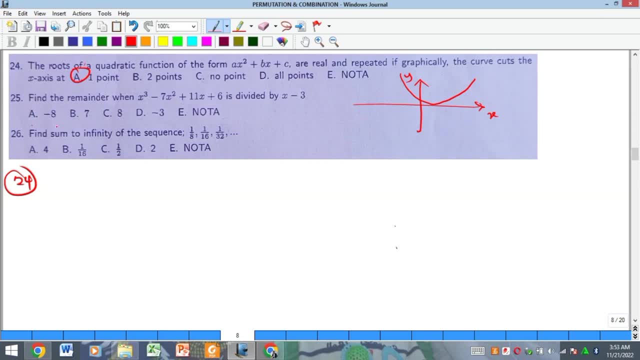 okay, so just at one point. so this is the solution. okay, so just at one point. so this is the solution. a now the second one, that's number 25. a now the second one, that's number 25. a now the second one, that's number 25 here says that we should find. 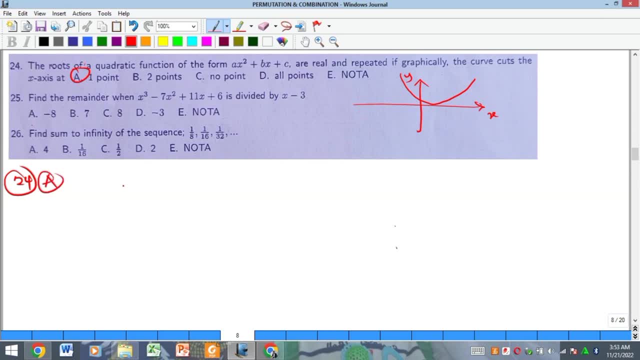 here says that we should find. here says that we should find. so this is option a, so i'll go to. so this is option a, so i'll go to. so this is option a, so i'll go to. number 25, which says that we should. number 25 which says that we should. 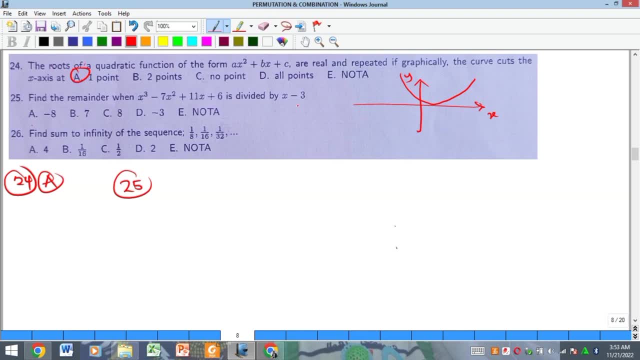 number 25, which says that we should find a remainder when this polynomial is. find a remainder when this polynomial is, find a remainder when this polynomial is divided by this, divided by this, divided by this, this one: now we also use remainder theorem. this one: now we also use remainder theorem. 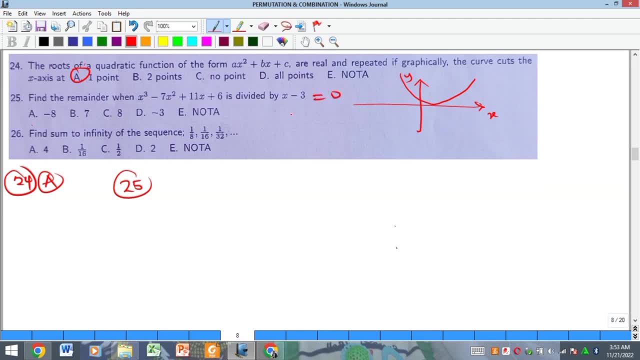 this one. now we also use remainder theorem, which says that if i equate this to zero. which says that, if i equate this to zero, which says that if i equate this to zero, that's the divisor and solve for x. that's the divisor and solve for x. 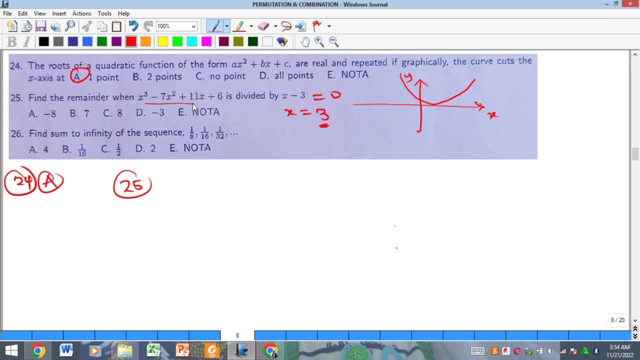 that's the divisor, and solve for x that if i substitute this value of x into that, if i substitute this value of x into that, if i substitute this value of x into the polynomial, whatever i get the polynomial, whatever i get, the polynomial, whatever i get is the remainder. so the remainder i'm. 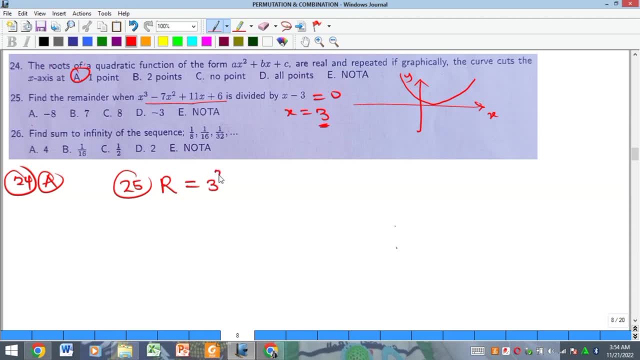 is the remainder, so the remainder i'm is the remainder, so the remainder i'm looking for, looking for, looking for is equal to 3 raised to the power of 3 is equal to 3 raised to the power of 3 is equal to 3 raised to the power of 3 minus 7 into 3 squared. 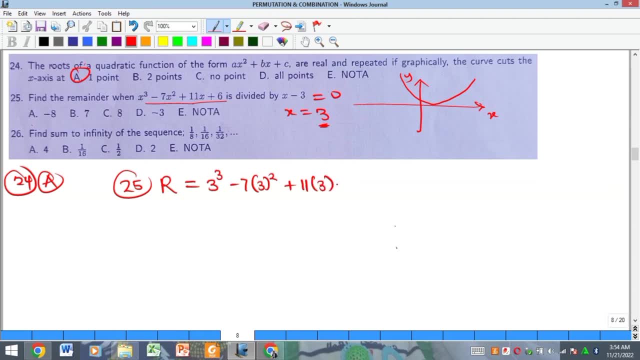 minus 7 into 3, squared minus 7 into 3, squared plus 11 times 3, then plus 6, plus 11 times 3, then plus 6, plus 11 times 3, then plus 6, and that's going to give me this is: 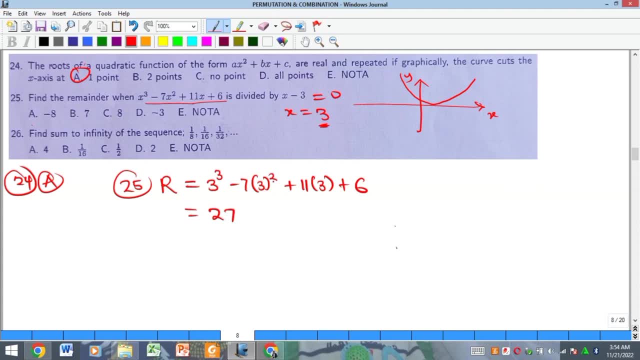 and that's going to give me this is: and that's going to give me this is 27. the 3 squared is 9 times 7. 27 the 3 squared is 9 times 7. 27 the 3 squared is 9 times 7. 3, 9 times 7 is also equal to. 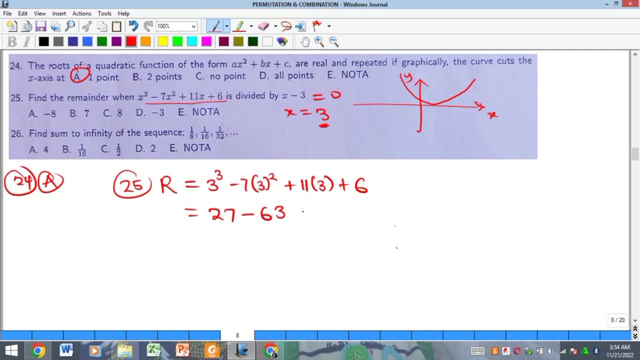 3, 9 times 7 is also equal to 3, 9 times 7 is also equal to 63, then this is going to give us 33- 63. then this is going to give us 33- 63. then this is going to give us 33, and then plus 6. so if we subtract this, 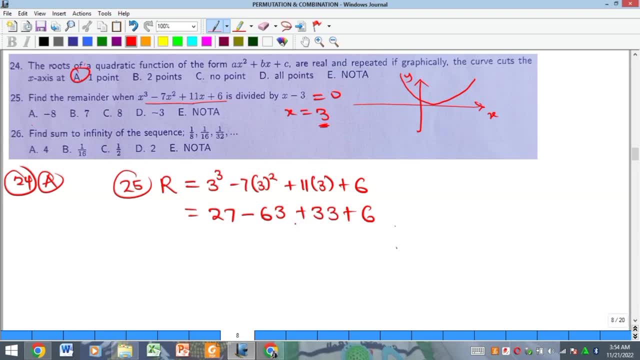 and then plus 6. so if we subtract this and then plus 6, so if we subtract this, if we add everything here, this is going. if we add everything here, this is going. if we add everything here, this is going to give us to give us, to give us minus 30 plus this is minus 3 plus 6. 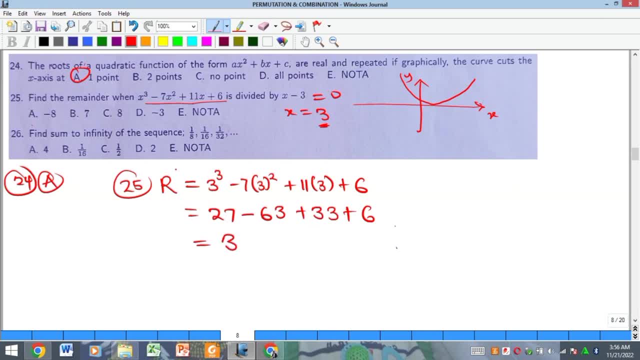 minus 30 plus this is minus 3 plus 6. minus 30 plus this is minus 3 plus 6, is equal to 3, is equal to 3, is equal to 3. that and so this is option e. that and so this is option e. 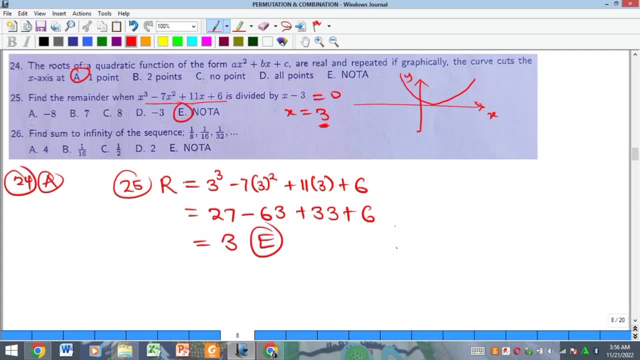 that, and so this is option e, that's none of the above. okay, so finally, for this page, we go for. okay, so finally for this page, we go for. okay, so finally for this page, we go for number 26 and number 26. number 26 and number 26. 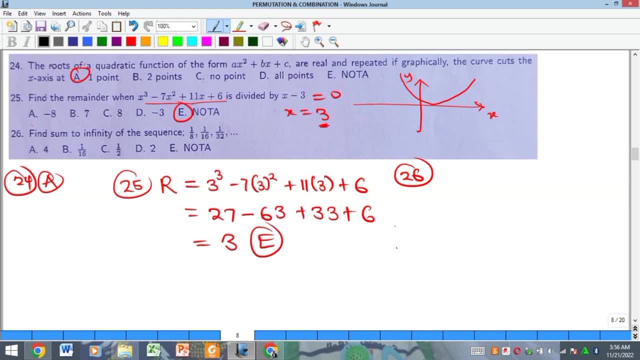 number 26, and number 26 says that we should find the sum to. says that we should find the sum to. says that we should find the sum to infinity. this is coming from a infinity, this is coming from a infinity, this is coming from a geometric progression: sum to infinity. 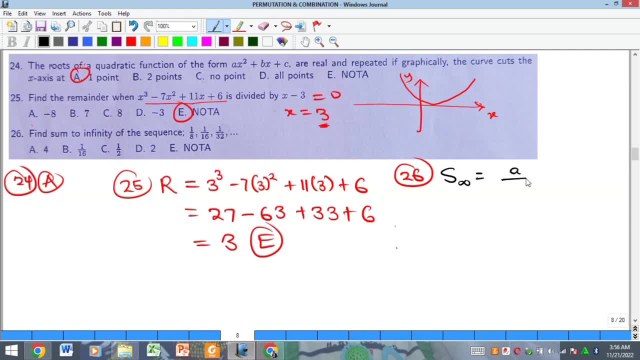 geometric progression: sum to infinity. geometric progression: sum to infinity. written this way is actually equal to written. this way is actually equal to written. this way is actually equal to: a, which is the first term. a, which is the first term, a, which is the first term. all over 1 minus r, if your. 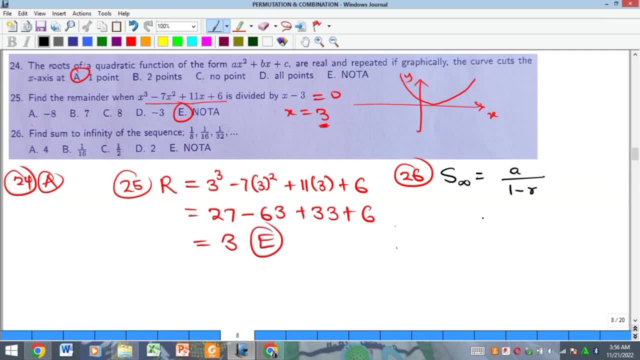 all over 1 minus r, if your all over 1 minus r, if your r is less than 1 and r is less than 1 and r is less than 1, and of course we can see it here. how do we? of course, we can see it here. how do we? 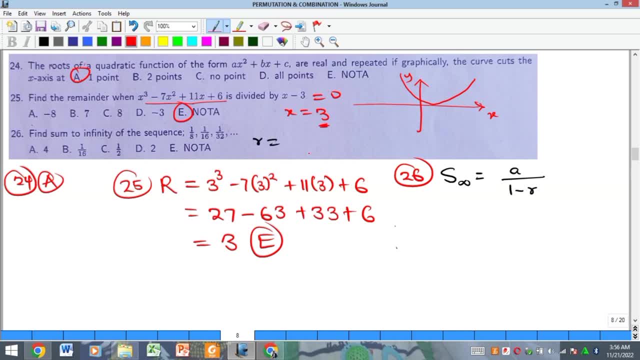 of course we can see it here. how do we get our r? get our r, get our r. our r is always equal to a term. our r is always equal to a term. our r is always equal to a term divided by the previous term. so we can. 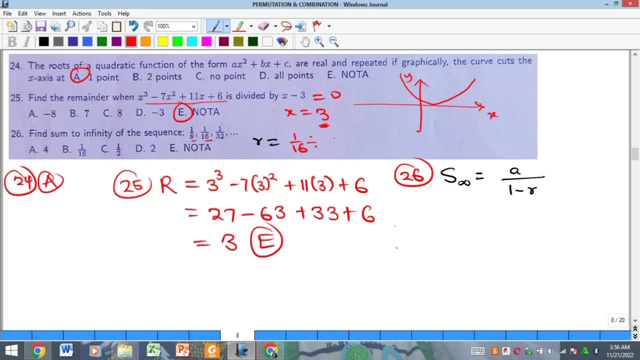 divided by the previous term. so we can divided by the previous term. so we can use 1 over 16 divided by 1 over 8. use 1 over 16 divided by 1 over 8. use 1 over 16 divided by 1 over 8 and of course, i can have this as 1 over. 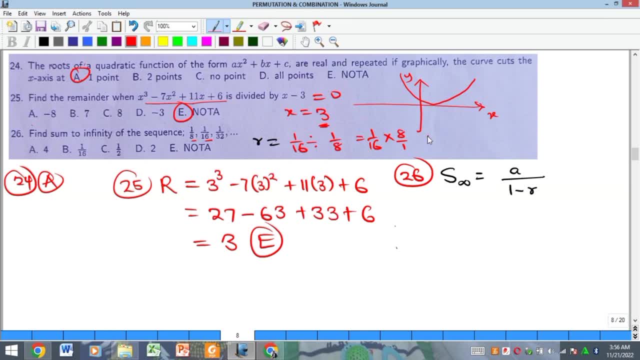 and of course, i can have this as 1 over, and of course i can have this as 1 over. 16 times 16 times 16 times 8 over 1, which will give me 1 over 2. 8 over 1, which will give me 1 over 2. 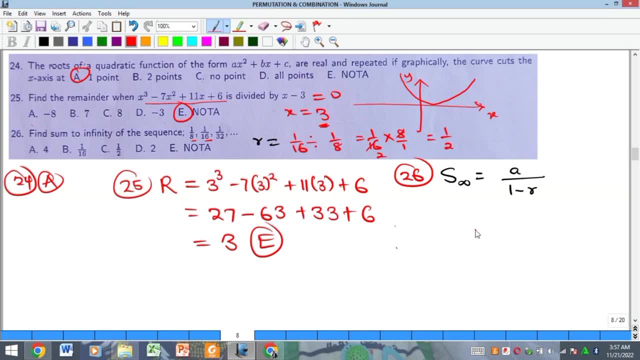 8 over 1, which will give me 1 over 2. if this cancels this, okay, so we put: if this cancels this, okay, so we put: if this cancels this, okay, so we put that here we are going to have a which, that here we are going to have a which. 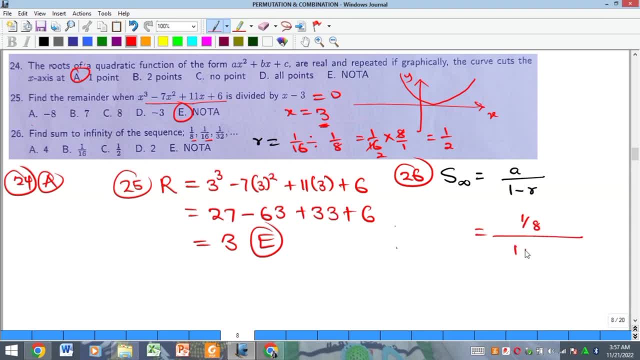 that here we are going to have a which is 1 over 8 all over. 1 minus 1 over 2 is 1 over 8 all over. 1 minus 1 over 2 is 1 over 8 all over 1 minus 1 over 2, and that is going to give us 1 over 8. 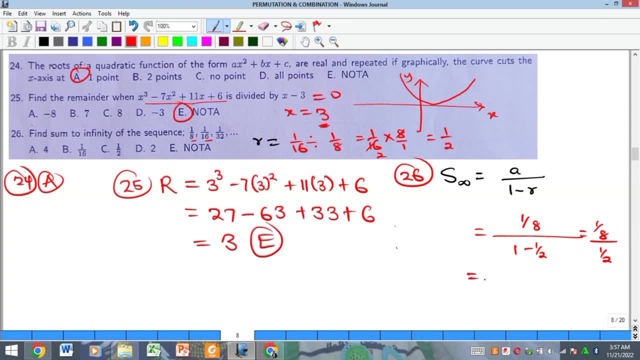 and that is going to give us 1 over 8, and that is going to give us 1 over 8 divided by 1 over 2, and this is equal to divided by 1 over 2, and this is equal to divided by 1 over 2, and this is equal to 1 over 8. if you change division to: 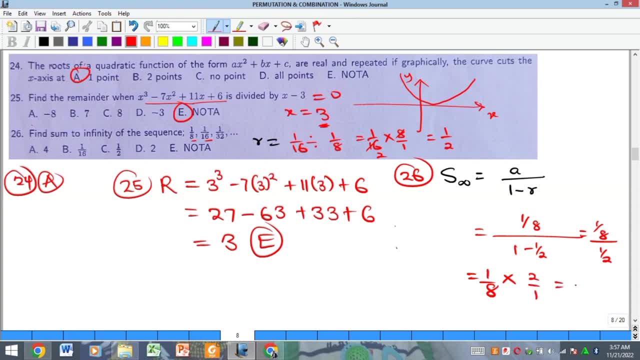 1 over 8 if you change division to 1 over 8. if you change division to multiplication, you have 2 over 1 and multiplication you have 2 over 1 and multiplication you have 2 over 1 and this will give us 1 over 4 as the. 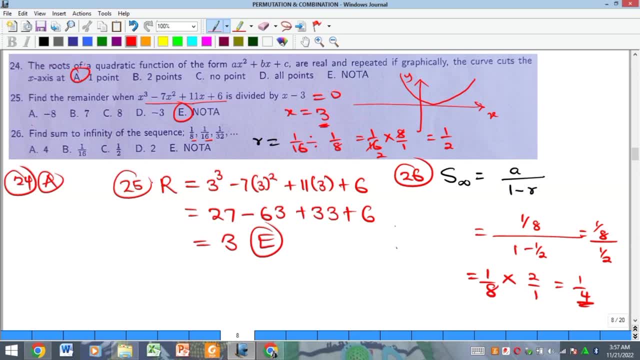 this will give us 1 over 4 as the. this will give us 1 over 4 as the solution, and here again we can see that solution, and here again we can see that solution, and here again we can see that the solution is also not there, and so we 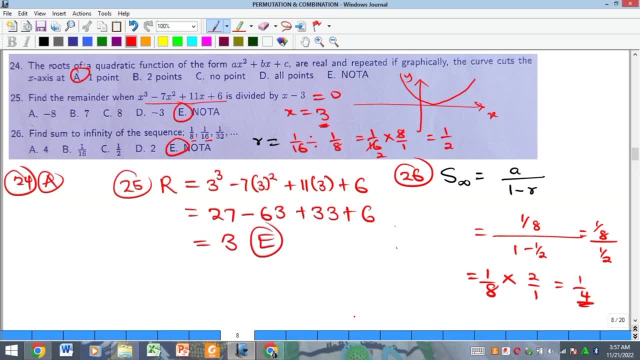 the solution is also not there, and so we the solution is also not there, and so we also choose none of the above as our also choose none of the above as our also choose none of the above as our solution. so to the number 27 solution. so to the number 27. 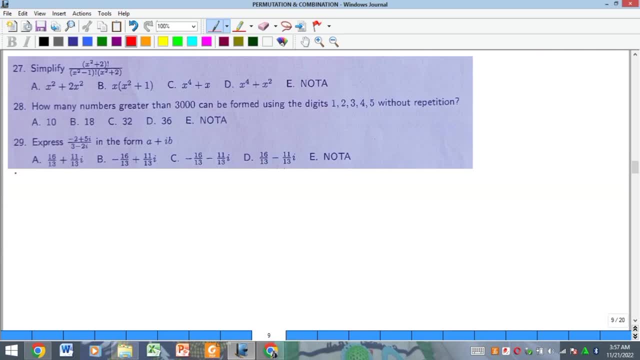 solution. so to the number 27. they asked us to simplify this. this is: they asked us to simplify this. this is: they asked us to simplify this. this is from factorials and of course you can from factorials and of course you can from factorials and of course you can find factorial, the video to factorial in. 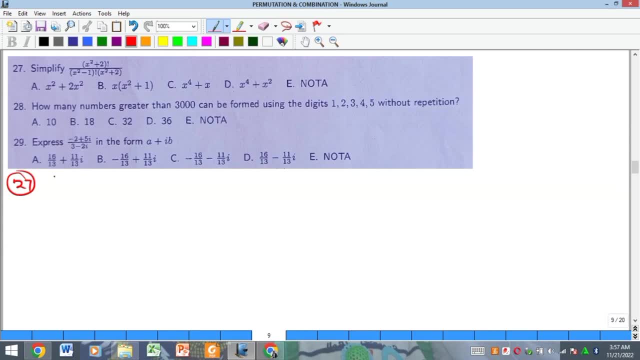 find factorial. the video to factorial in find factorial. the video to factorial in our channel here. so this is going to be our channel here. so this is going to be our channel here. so this is going to be. we have x squared plus two. we have x squared plus two. 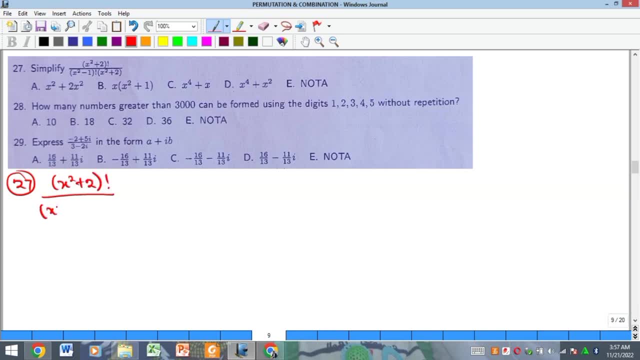 we have x squared plus two, factorial all over, x squared minus one. factorial all over x squared minus one. factorial all over, x squared minus one factorial factorial factorial. x squared plus two. so what are we going? x squared plus two. so what are we going? x squared plus two. so what are we going to do? 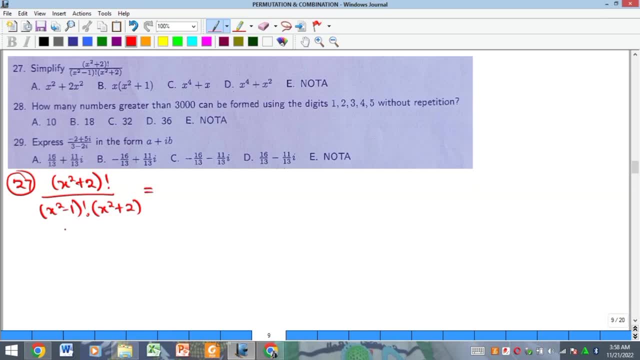 to do, to do now. look at the denominator- the denominator. now look at the denominator- the denominator. now look at the denominator. the denominator has x squared minus one. has x squared minus one. has x squared minus one. so remember the formula for factorial. if so, remember the formula for factorial if. 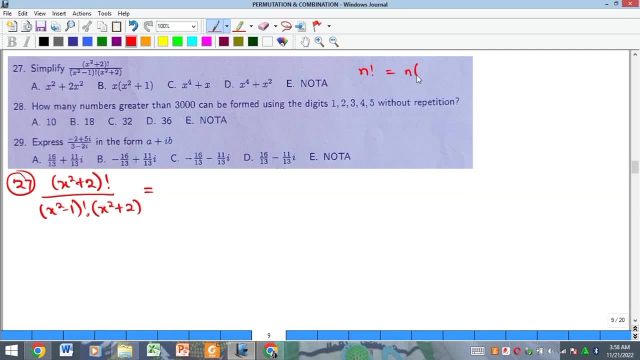 so remember the formula for factorial: if you have this, this is the same thing. you have this, this is the same thing. you have this, this is the same thing as n times. you keep subtracting one as n times. you keep subtracting one as n times. you keep subtracting one. you keep subtracting one, just like that. 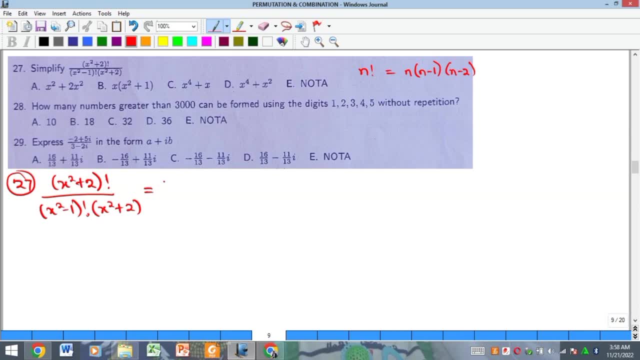 you keep subtracting one just like that. you keep subtracting one just like that. so if i subtract, if i just bring it the, so if i subtract, if i just bring it the, so if i subtract, if i just bring it the way it is, way it is. 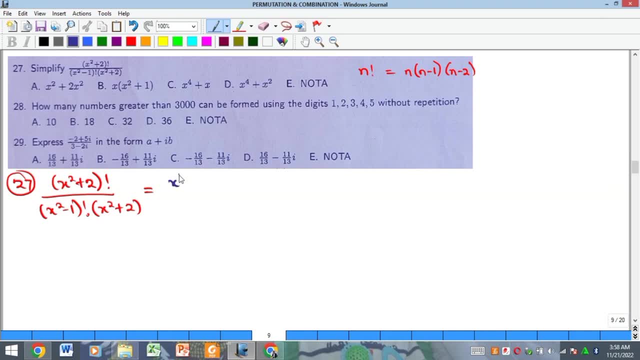 way it is. i am going to have my x squared. i am going to have my x squared. i am going to have my x squared plus two times. i will remove one plus two times. i will remove one plus two times. i will remove one. that's x squared plus one. i will remove. 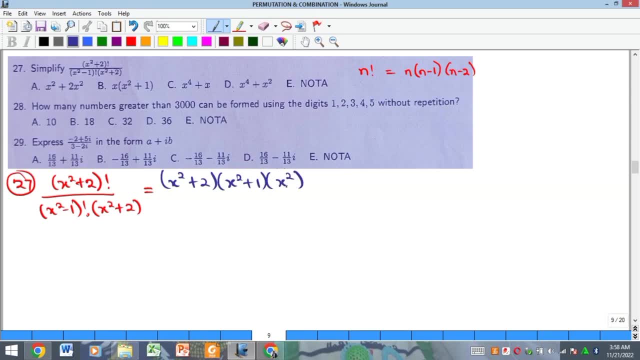 that's x squared plus one. i will remove that's x squared plus one. i will remove one. again: that's x squared minus one. one again: that's x squared minus one. one. again, that's x squared minus one. why am i going that way? i want to get. why am i going that way? i want to get. why am i going that way? i want to get to what is in the denominator, so i can to what is in the denominator, so i can to what is in the denominator, so i can stop here, stop here. 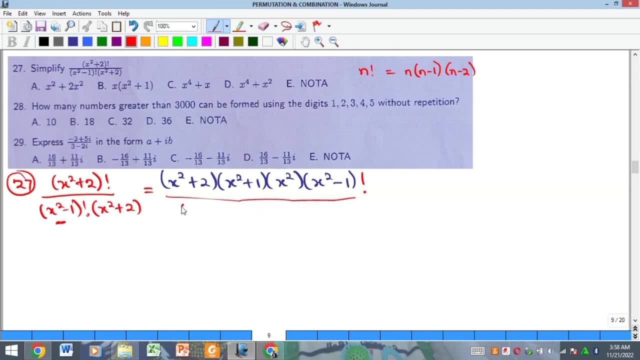 stop here, then this is all over. and then in my, then this is all over. and then in my, then this is all over. and then in my denominator i just write what i have. denominator, i just write what i have. denominator, i just write what i have there. and then here i also bring it down. 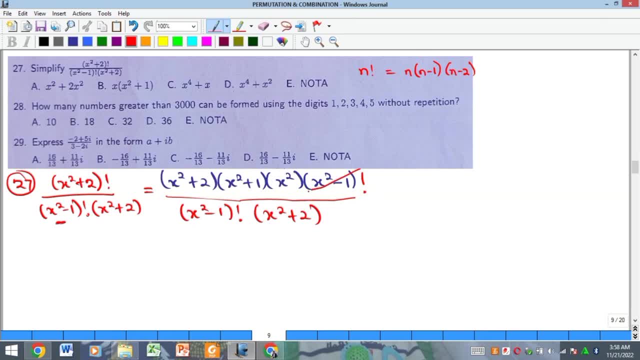 there and then here. i also bring it down there and then here. i also bring it down now, at this point. you can see, now, at this point, you can see now, at this point, you can see this: x squared minus one factorial will this x squared minus one factorial will. 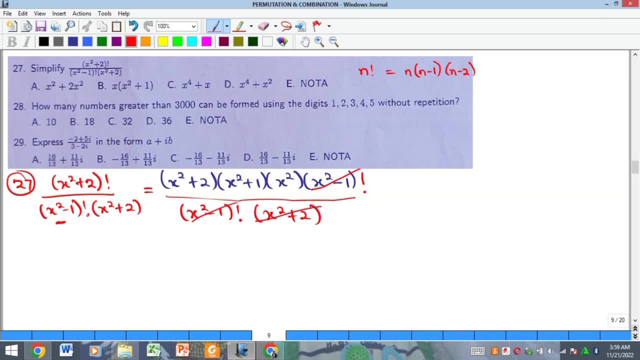 this: x squared minus one. factorial will remove this. remove this, remove this. and already you can see x squared plus, and already you can see x squared plus, and already you can see x squared plus two there. so this is going to give us two there. so this is going to give us. 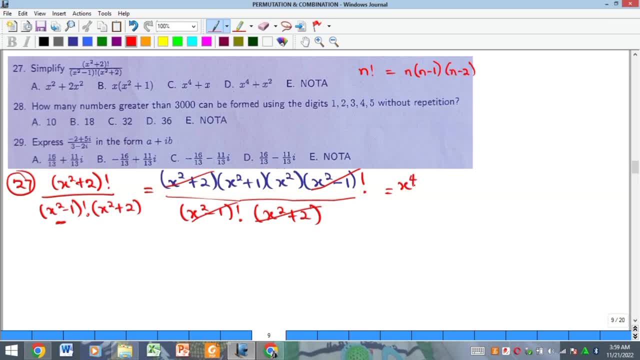 two there. so this is going to give us: if this multiplies, you have x raised to. if this multiplies, you have x raised to. if this multiplies, you have x raised to power four, power four. power four plus x squared as our solution, and that plus x squared as our solution, and that. 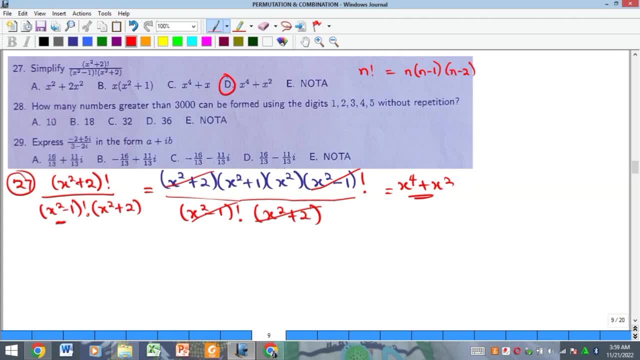 plus x squared as our solution, and that is the, is the is the option d. now this one says how many option d. now. this one says how many option d. now. this one says how many numbers greater than numbers greater than numbers greater than 3000 can be formed using the digits we. 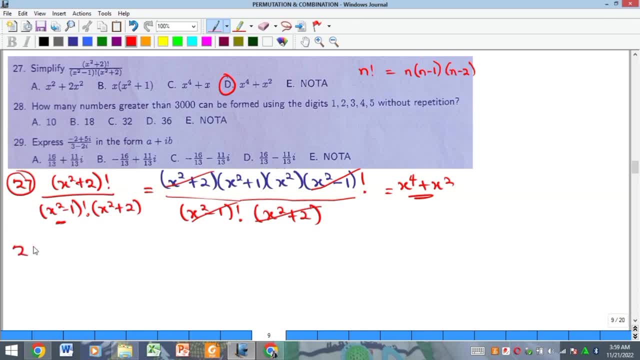 3000 can be formed using the digits we. 3000 can be formed using the digits we have here, have here, have here: this number 28 is from permutation and this number 28 is from permutation and this number 28 is from permutation and combination. 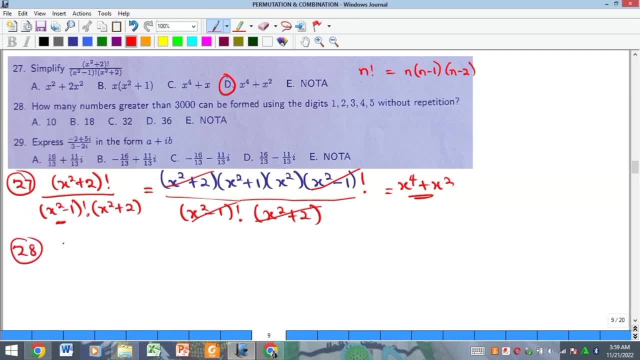 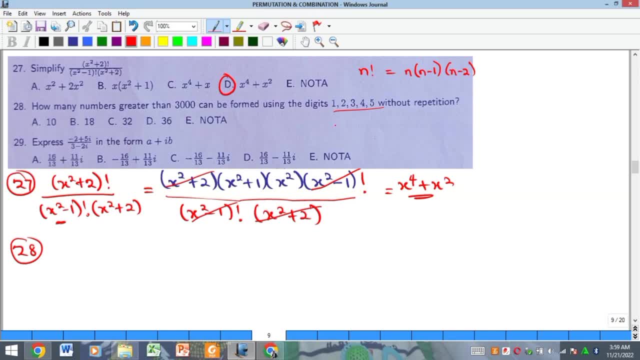 five digits to form a four digit number. so there are two ways we can form this. so there are two ways we can form this. so there are two ways we can form this. remember they say without repetition, remember they say without repetition, remember they say without repetition. so the first way is that. 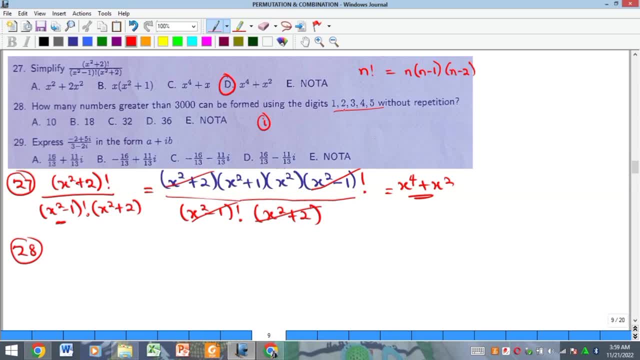 so the first way is that. so the first way is that we can use any of the numbers that so we can use any of the numbers that so we can use any of the numbers that so form a five digit: any five digit number. form a five digit: any five digit number. 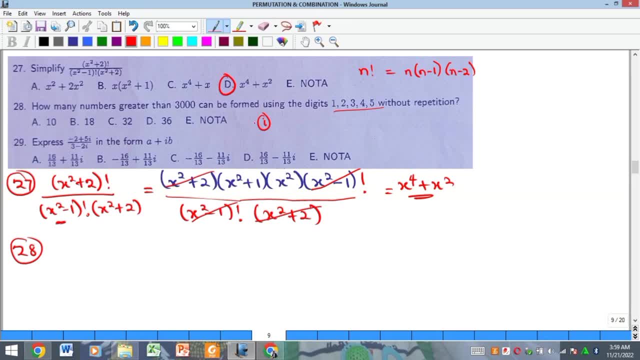 form a five digit, any five digit number you form will definitely be greater than you form, will definitely be greater than you form will definitely be greater than three thousand three thousand three thousand. so that means: so that means form uh. so that means form uh. so that means form uh. form any five digits. 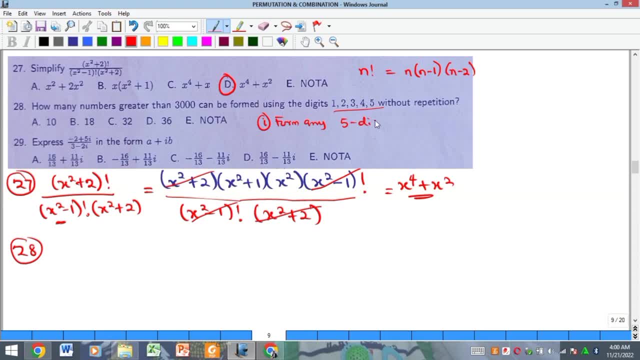 form any five digits, form any five digits, any five digits number, and if we form any any five digits, any five digits number, and if we form any any five digits, any five digits, number from here, number from here, number from here, that means we can pick anyone and 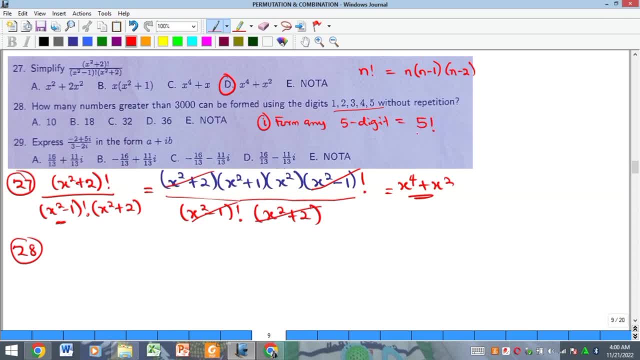 that means we can pick anyone. and that means we can pick anyone. and that's actually equal to five factorial. that's actually equal to five factorial. that's actually equal to five factorial. okay, and then the next way, let me bring. okay, and then the next way, let me bring. 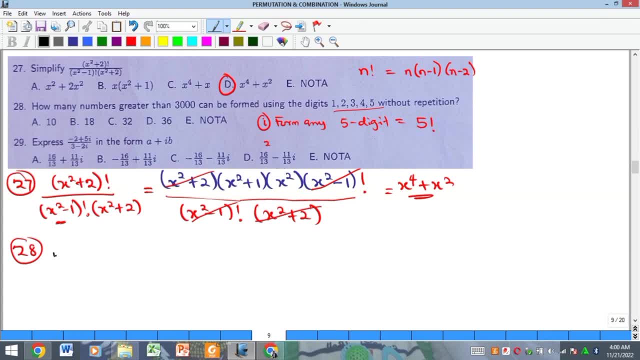 okay, and then the next way: let me bring this thing i'm doing down here, so the this thing i'm doing down here, so the this thing i'm doing down here, so the next way we can get a, a number that is. next way we can get a, a number that is. 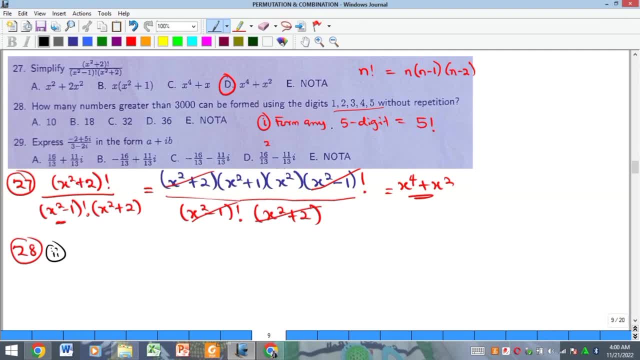 next way we can get a, a number that is greater than three thousand, greater than three thousand, greater than three thousand is to, is to is to now form four digit number. that the four now form four digit number. that the four now form four digit number. that the four digit number we are going to form. 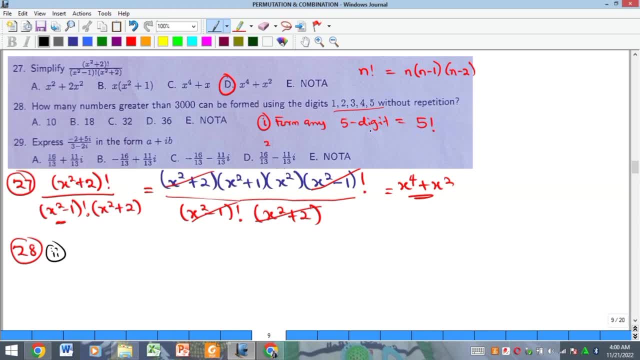 digit number we are going to form. digit number we are going to form must begin with: either sorry, we must must begin with, either sorry, we must must begin with, either sorry. we must begin with a number that is greater. begin with a number that is greater, begin with a number that is greater or equal to three. so from here, now we 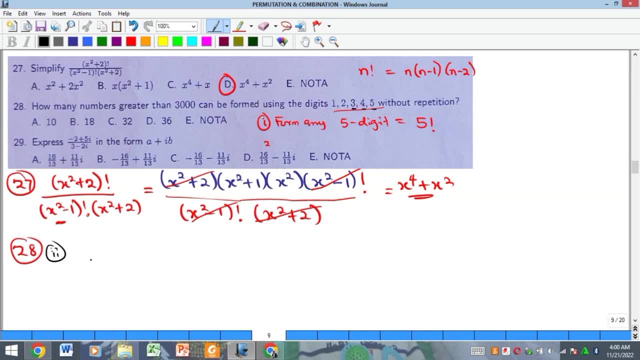 or equal to three, so from here now we or equal to three, so from here now we can pick three, four or five. so what it can pick- three, four or five, so what it can pick- three, four or five. so what it means is that look at what is going to. 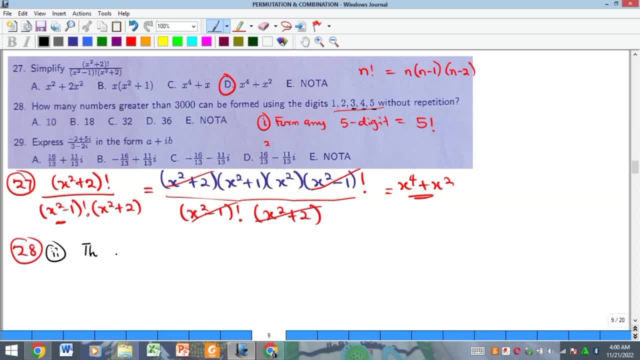 means. is that look at what is going to means? is that look at what is going to be? we're going to have the thousand be. we're going to have the thousand be. we're going to have the thousand column, then we'll have the hundred column, then we'll have the hundred. 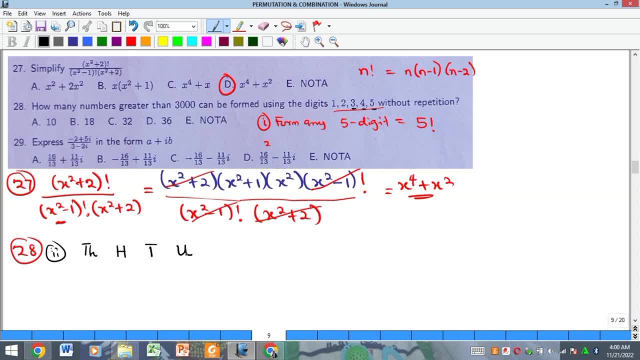 column, then we'll have the hundred column, then we have the tens column and column, then we have the tens column and column, then we have the tens column and we have the unit column. so we're going we have the unit column. so we're going we have the unit column. so we're going to be using counting system here. so for 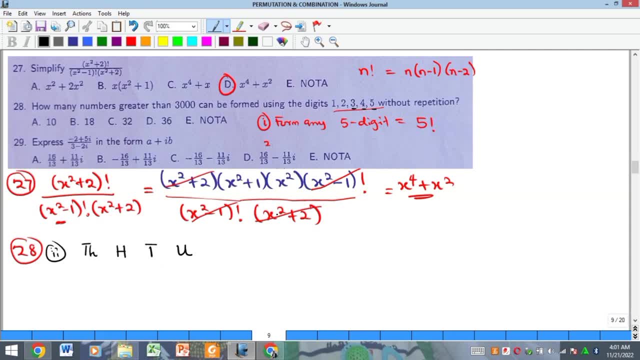 to be using counting system here, so for to be using counting system here, so for the hundred column only numbers the hundred column only numbers the hundred column only numbers three, four and five can be here. so only three, four and five can be here. so only three, four and five can be here, so only three can enter here, and that is times. 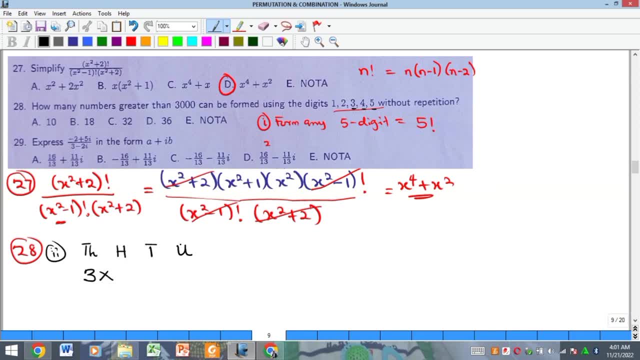 three can enter here, and that is times. three can enter here, and that is times now. what about hundred column? how many now? what about hundred column? how many now? what about hundred column? how many can enter now? all of them can actually, can enter now. all of them can actually. 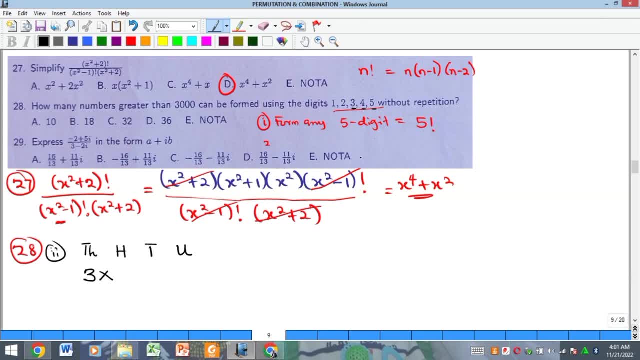 can enter now, all of them can actually enter here, and it will be greater than enter here and it will be greater than enter here and it will be greater than three thousand. however, they said without three thousand. however, they said without three thousand. however, they said without repetition. so meaning, if i pick any of 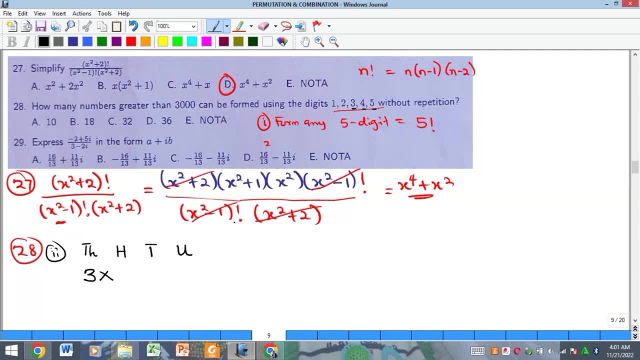 repetition. so meaning if i pick any of repetition. so meaning if i pick any of three, four and five, i will be left with three, four and five. i will be left with three, four and five. i will be left with only four digits to pick, so only four. 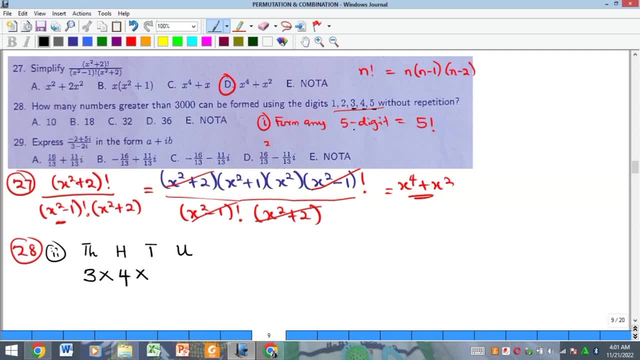 only four digits to pick, so only four. only four digits to pick, so only four can enter here. times now also if i've can enter here. times now also if i've can enter here. times now also if i've picked any of three, four and five and 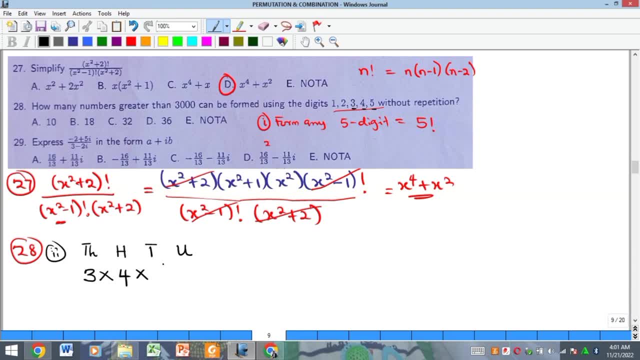 picked any of three, four and five. and picked any of three, four and five. and i've picked also 400. i've picked also 400. i've picked also 400 column. then for tens column, only three column. then for tens column, only three column. then for tens column, only three digits will be left to be picked, and in 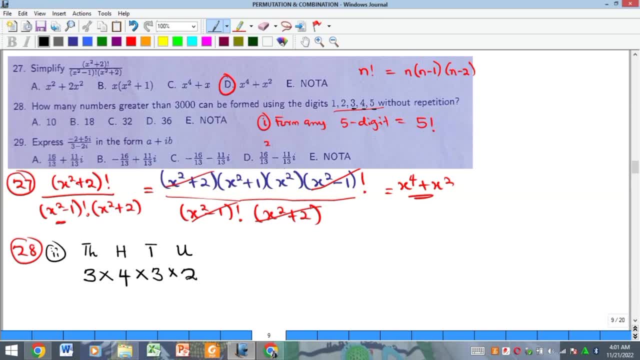 digits will be left to be picked and in digits will be left to be picked and in the same vein, only two will be left here the same vein, only two will be left here the same vein, only two will be left here to be picked. and so if we multiply this, 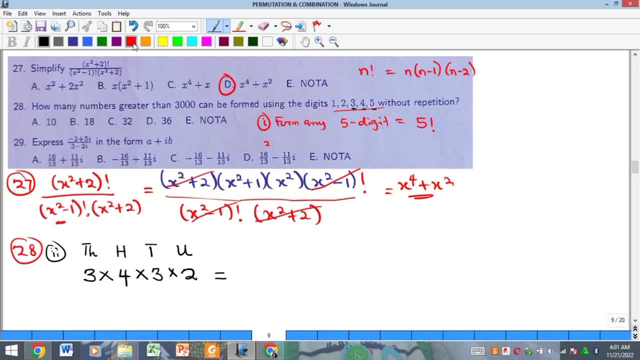 to be picked. and so if we multiply this, to be picked. and so if we multiply this, we are going to get the next, the next number of digits that can help, the next number of digits that can help, the next number of digits that can help us get. 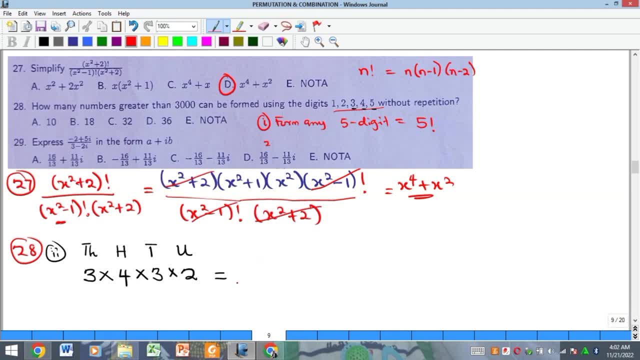 us get, us get, sorry. the next number of formations, sorry, the next number of formations, sorry, the next number of formations that will give us number greater than that, will give us number greater than that, will give us number greater than three thousand. and this is going to be. 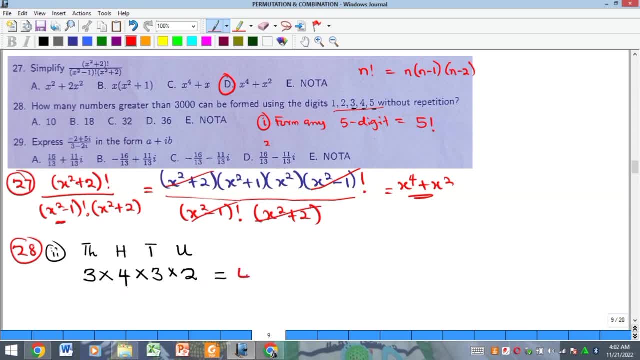 three thousand, and this is going to be three thousand, and this is going to be twelve twenty four, twenty four times two. twelve twenty four, twenty four times two. twelve twenty four, twenty four times two is forty eight. and so now, whereas this, is forty eight. and so now, whereas this 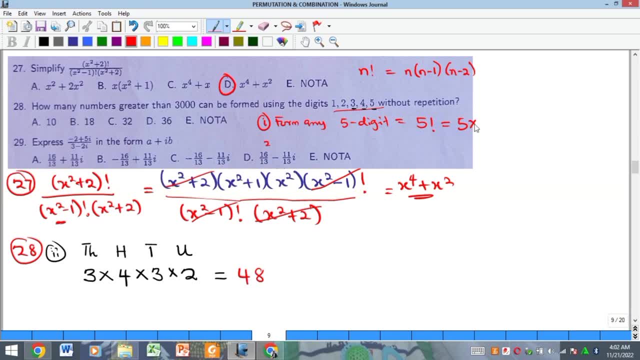 is forty eight. and so now, whereas this one is five factorial which is five, one is five factorial which is five, one is five factorial which is five times four times three times, two times times four times, three times, two times times four times three times, two times one. this is twenty, this is sixty one. 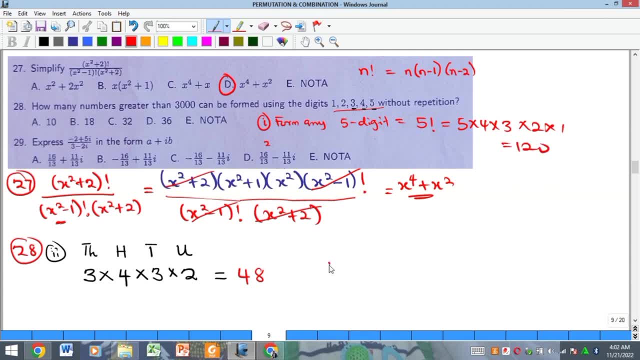 one. this is twenty. this is sixty one. one. this is twenty. this is sixty one: twenty. so the total number. total number: twenty. so the total number. total number: twenty. so the total number. total number of digits that can be formed from these, of digits that can be formed from these. 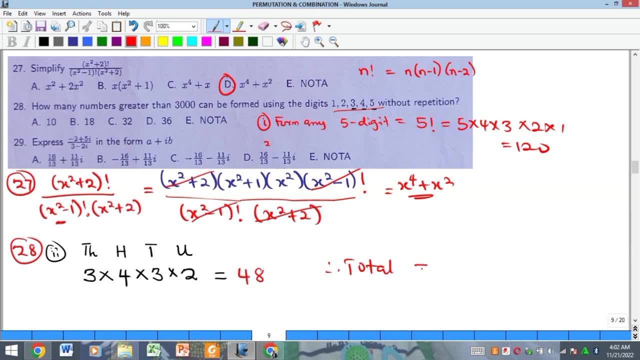 of digits that can be formed from these numbers, and without repetition, that will numbers. and without repetition, that will numbers. and without repetition, that will give us a number greater than three. give us a number greater than three. give us a number greater than three. thousand is one twenty plus forty eight. 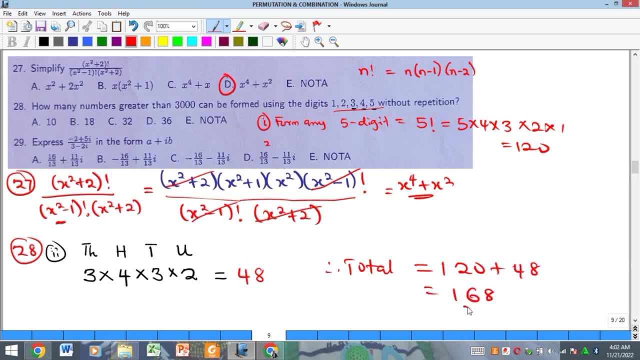 thousand is one twenty plus forty eight thousand is one twenty plus forty eight, and that is one hundred and sixty eight, and that is one hundred and sixty eight, and that is one hundred and sixty eight. and of course you can see it is not in, and of course you can see it is not in. 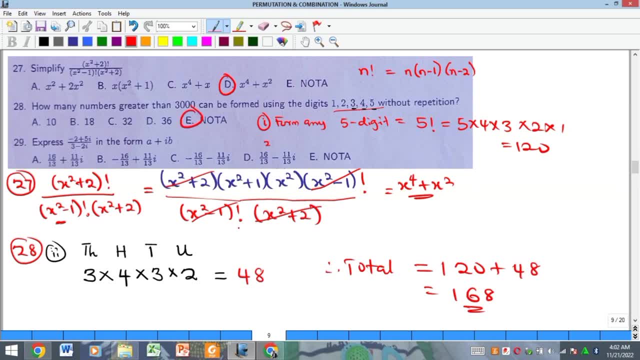 and of course you can see, it is not in the option, the option, the option, and so that is what, and so that is what, and so that is what. sorry, please, sorry, please, sorry, please. look at the mistake here. this is not. look at the mistake here. this is not. 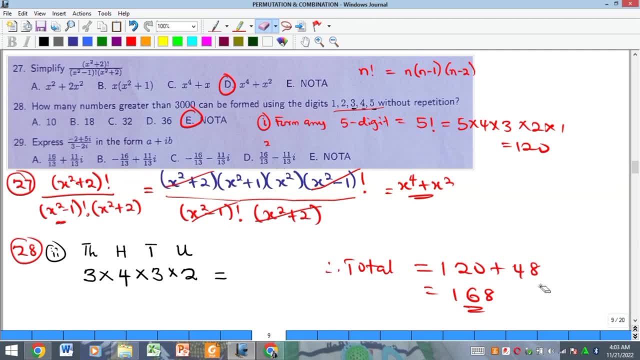 look at the mistake here. this is not forty eight. forty eight, forty eight is a mistake. i'm sorry about that is a mistake. i'm sorry about that is a mistake. i'm sorry about that, okay, look at it. our this time. this is okay. look at it: our this time. this is. 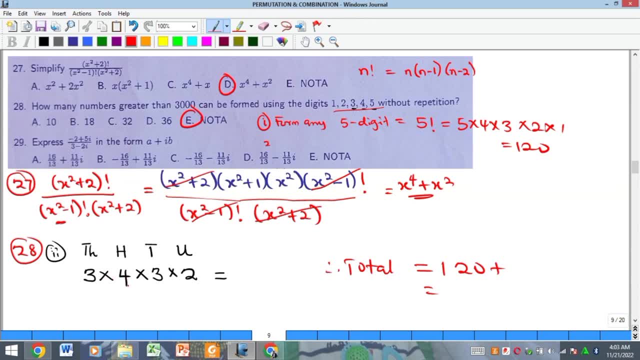 okay, look at it, our this time. this is twelve twelve times three is 36. twelve twelve times three is 36. twelve twelve times three is 36, not 24. and 36 times 2 is not 24 and 36 times 2 is not 24 and 36 times 2 is 72. so sorry, we're supposed to have 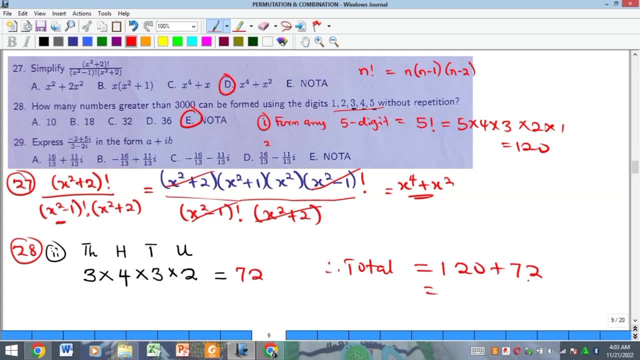 72. so sorry we're supposed to have 72, so sorry we're supposed to have plus 72 here, plus 72 here, plus 72 here, and when you add 72, and when you add 72, and when you add 72 to 120. 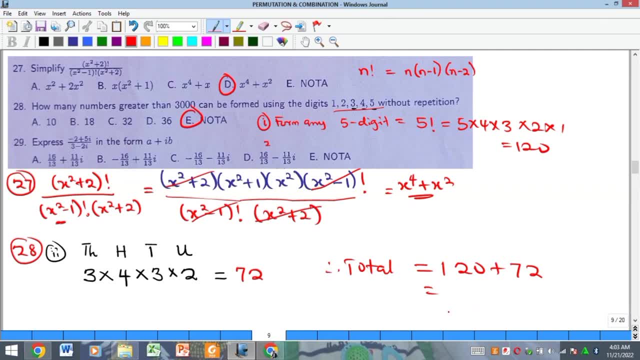 to 120. we are then going to have 192, and it is. we are then going to have 192, and it is. we are then going to have 192, and it is still, still, still none of the above. okay, so so quickly, we then go to. 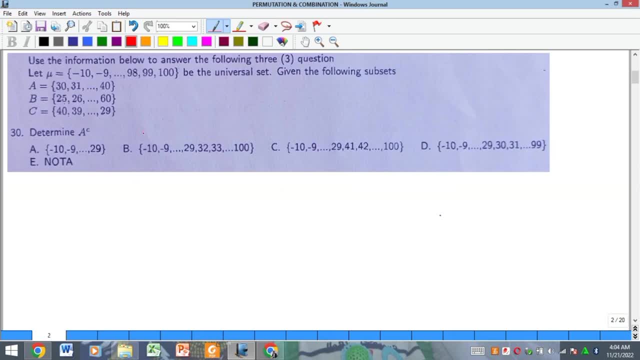 okay, so so quickly we then go to okay. so so quickly. we then go to the number 13. now look at this one. it the number 13. now look at this one. it the number 13. now look at this one. it says that we should use the information. 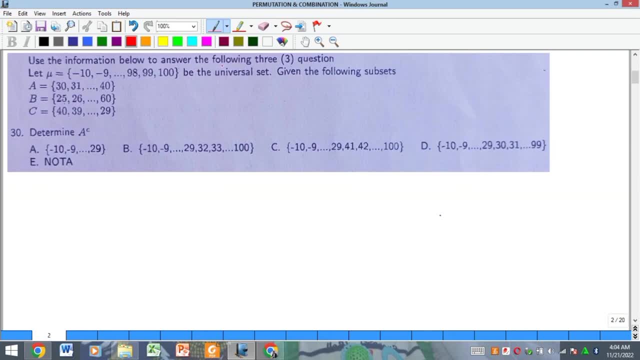 says that we should use the information. says that we should use the information below to answer below, to answer below to answer the following three questions. that's from the following three questions. that's from the following three questions. that's from 30 to 31 and 32. remember i said that? 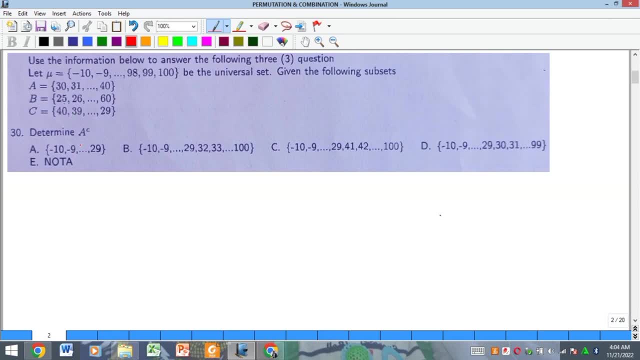 30 to 31 and 32. remember i said that 30 to 31 and 32. remember i said that there are 33 questions. there are 33 questions. there are 33 questions. so let's look at this. it says that you. so let's look at this: it says that you. 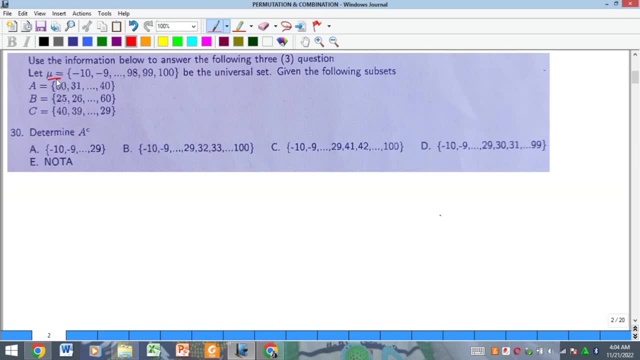 so let's look at this. it says that you are giving a universal set, are giving a universal set, are giving a universal set which is this, and then that's minus 10, which is this, and then that's minus 10, which is this, and then that's minus 10 up to 100, and then they're asking us: 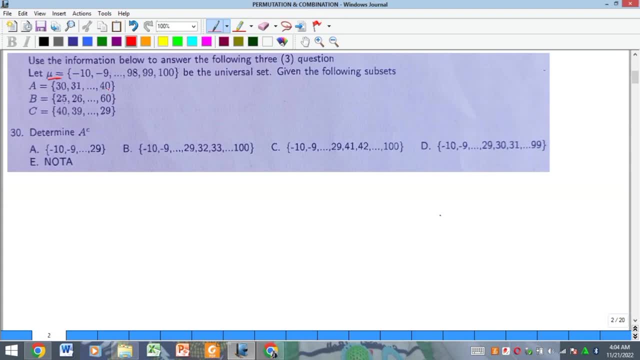 up to 100, and then they're asking us up to 100, and then they're asking us this and a is this from 30 to 40 from d? this and a is this from 30 to 40 from d. this and a is this from 30 to 40, from d is 25 to 60 and c is 40 down to 29. 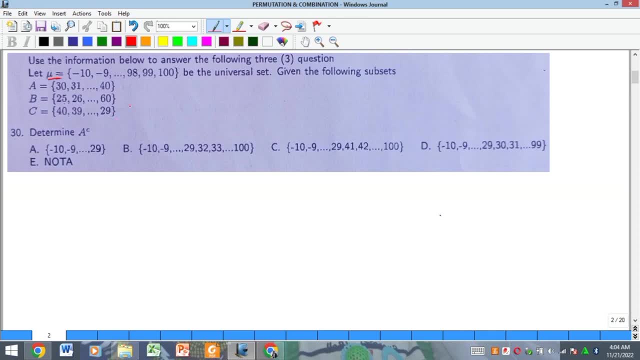 is 25 to 60 and c is 40 down to 29, is 25 to 60 and c is 40 down to 29. okay, so we can actually list these. okay, so we can actually list these. okay, so we can actually list these elements if we want. 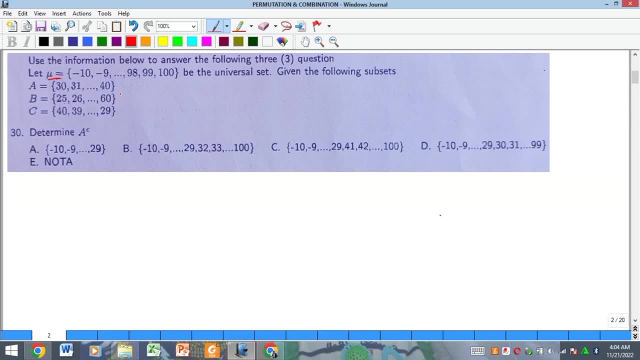 elements. if we want elements, if we want number, they say we should determine a number. they say we should determine a number. they say we should determine a complement meaning elements in the complement meaning elements in the complement meaning elements in the universal set that are not in a. so what? 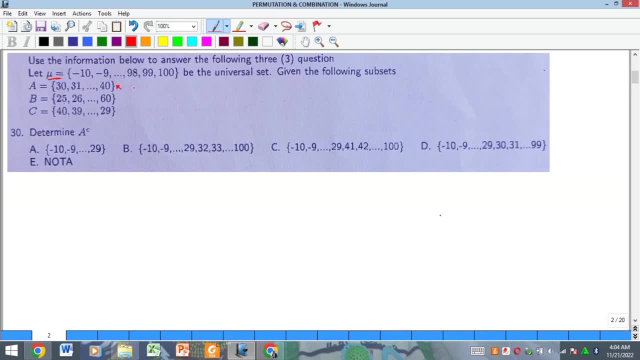 universal set that are not in a? so what universal set that are not in a? so what is that going to be? let's try to. is that going to be? let's try to. is that going to be? let's try to where we can actually, where we can actually. 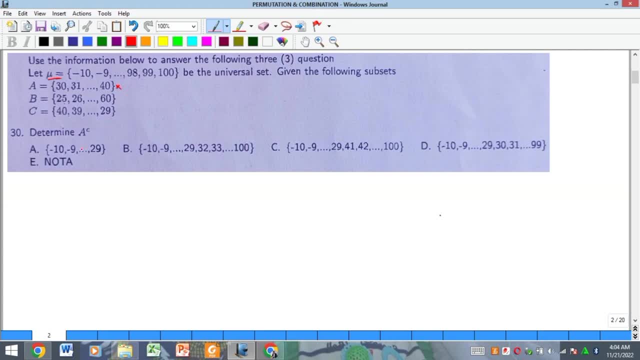 where we can actually list, like i said, but there will be no list, like i said, but there will be no list, like i said, but there will be no point, point, point to look at it. so our a compliment is to look at it. so our a compliment is: 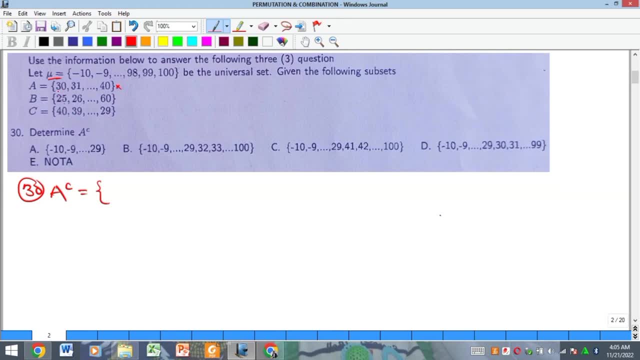 to look at it. so our a compliment is simply going to be, simply going to be simply going to be so. a started from 13, that means so. a started from 13, that means so. a started from 13, that means minus 10 is not going to be there, so 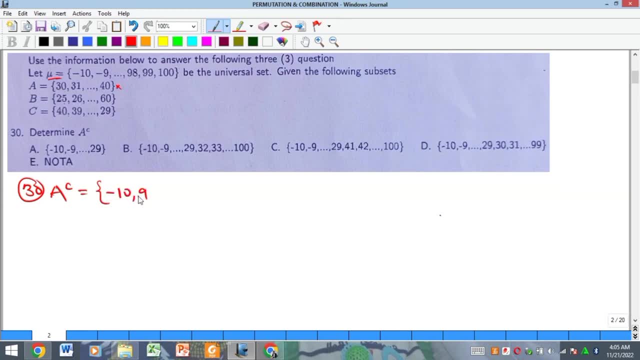 minus 10 is not going to be there. so minus 10 is not going to be there, so i'll go from minus 10. i'll go from minus 10. i'll go from minus 10, minus 9, sorry down to minus 9, sorry down to. 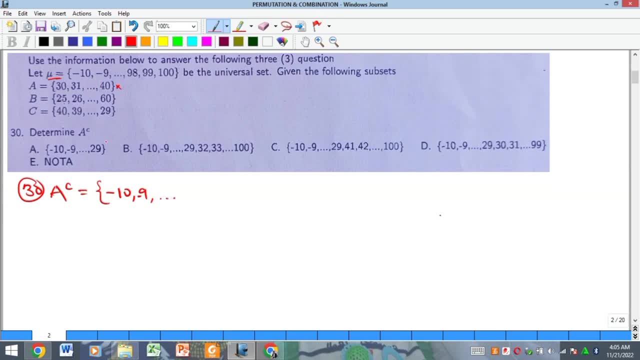 minus 9. sorry, down to remember: these elements are just whole. remember these elements are just whole. remember these elements are just whole. number, so number. so there's no point. down to 29. so 29 is not here and then i will now jump up to 40 is in a, so i. 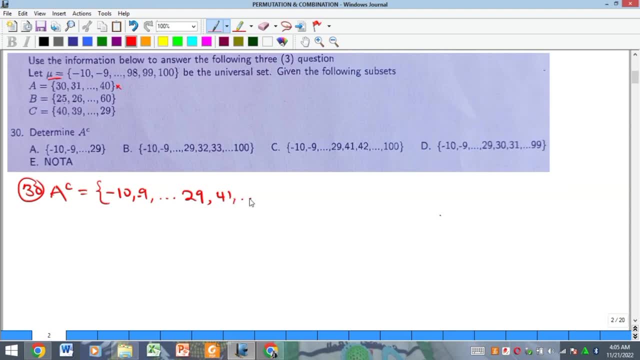 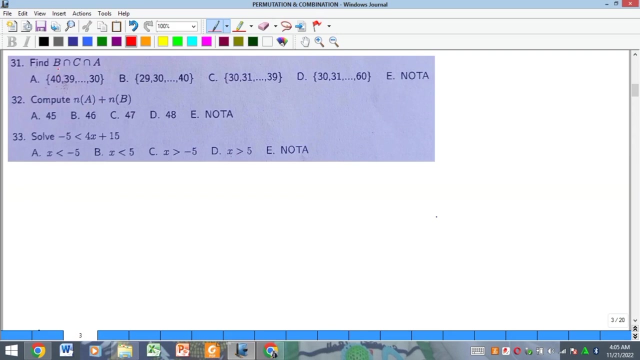 will begin from 41, 42 down to 100, which are elements in the universal set. this is the complement of a. let's look at the options and it is somewhere here. option c, that's the solution for number 30, and then we quickly go to the next one, which is 31. that one says b, intersection c. 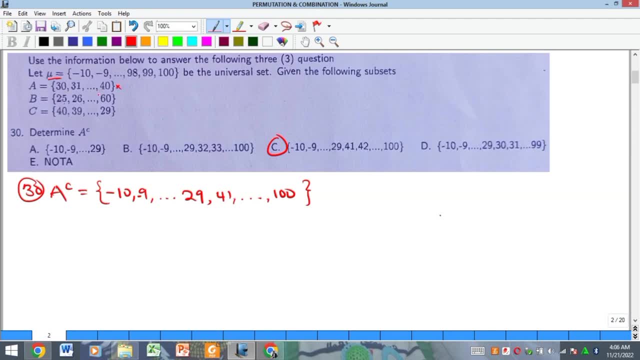 intersection a. so we'll keep referring back to this place. what is our b? this is b. it said in intersection c, intersection a. okay, so 31 is b. intersection c, intersection a, meaning elements here, here and here, elements in this three. okay, so what are the elements in the three of them? okay, let's begin from. 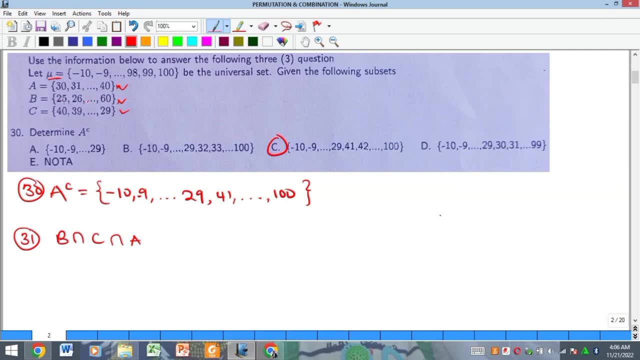 here, of course, 25 to 40. contains to 60, contains 40 in between. so 40 must be in that intersection. then what else? okay, now, remember that this one now is going down this way: this one is going down, this one is going up. okay, so the other. 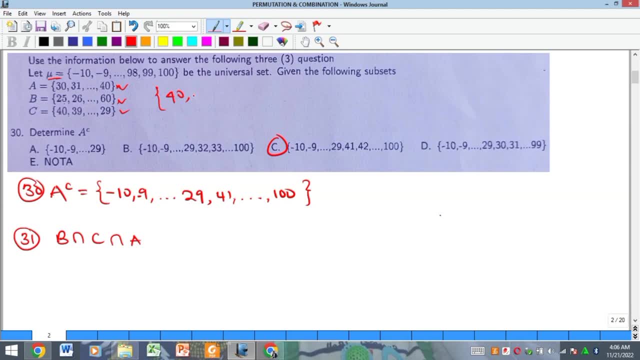 thing that will be in this would definitely be 39. 39 will be there, because 39 is here, is here, is also here, then 38 will also be there and 37 will be there, and in fact, you keep going down and the only thing is that for this one, 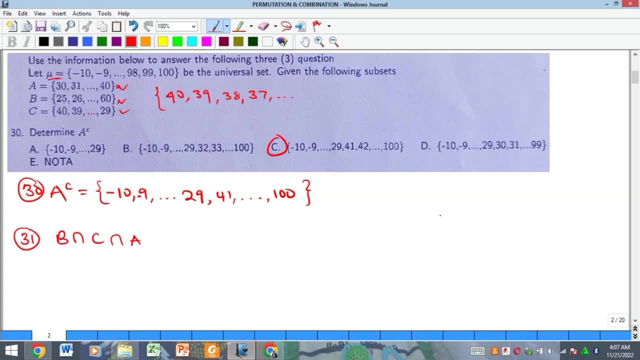 now you are going to stop at 30, because 30 is also here and 30 is here. remember this. one moves down, so it crossed 30 before getting to 29. we can pick 29 even though 29 is here is here, but it is not here. so we are going to stop at 30 and let's 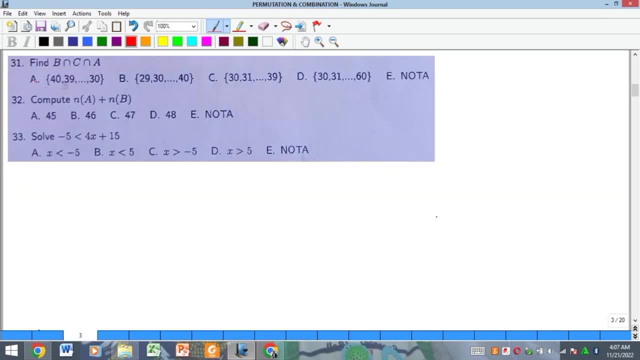 check. okay. so from 40 down to 30, that is definitely option A. and then back. they said we should find n of A plus n of B. what's n of A? cardinality of A number of elements in A and n of B? A plus n of B was n of B. cardinality of A number of elements in a number of elements in a and N of B. a plus n of B was N of A. cardinality of A number of elements in a and N of B: a. 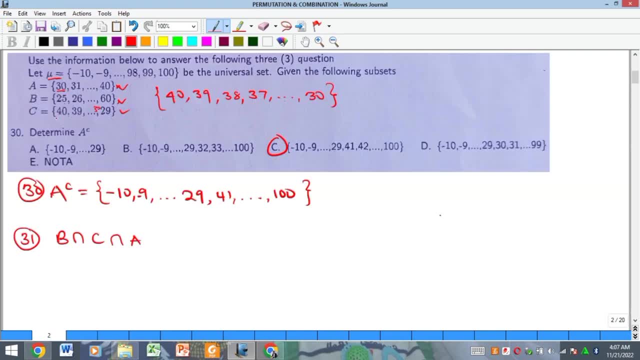 is cardinality of b. so let's go back. so can we check the cardinality from 30 to 40. of course, from 31 to 40 is 10, that's 10 elements, 10 numbers. then if you add 30, so it means that for number 32, 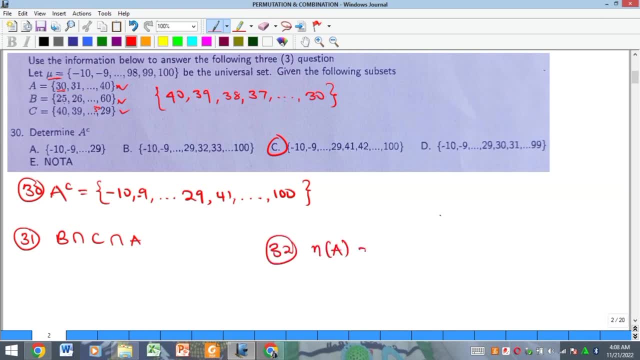 the cardinality of a is equal to 11 and then the other one is cardinality of b. let's look at it from 31 to 60 is going to be 30 number. that's, if you number from 31 to 60, you have 30 numbers. 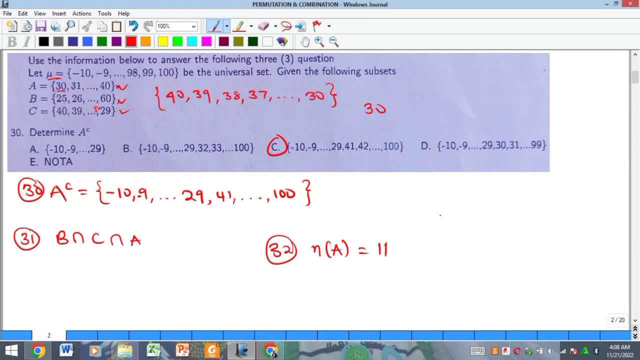 then what about from 25 to 30? sorry, if you number from 31 to 60 will be 30 numbers. then what about from 25 to 30? you can count 25, 26, 27, 28, 29, 30. these are ор. 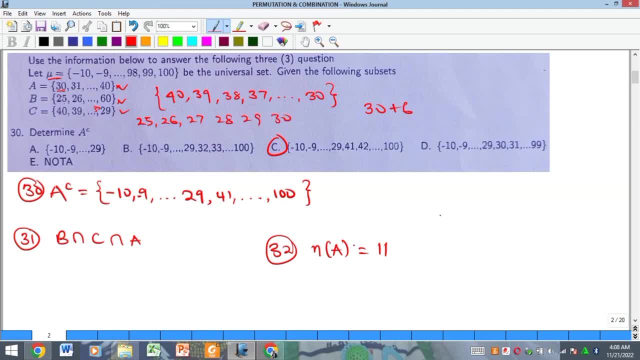 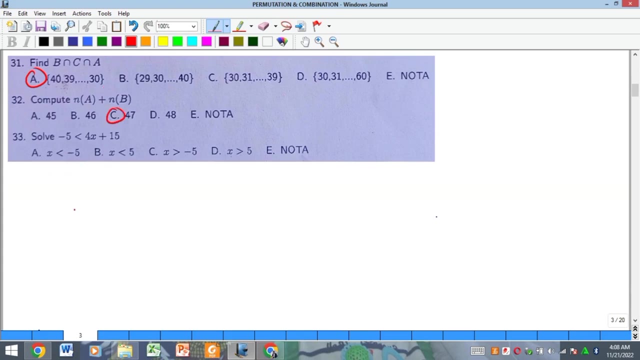 six digits. so you add it here. so you have that your n of b is equal to 36. therefore the sum of the two will give you 47 as your solution and you can see that here as option, option c, and then finally we have that we should solve this inequality. so for number 33 to solve the 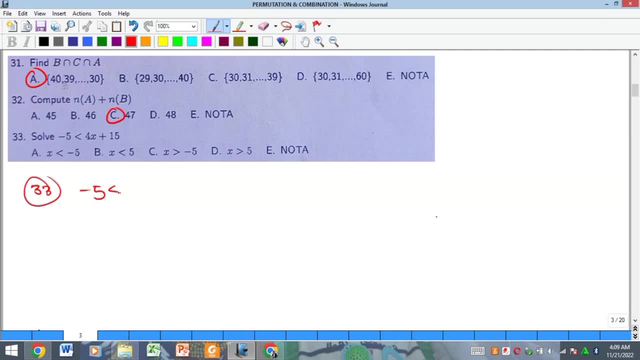 inequality here i have: minus 5 is less than 4x plus 15.. all i will need to do is collect like times. so take this 15 to this side, so i'll have minus 15. sorry, minus 5 minus 15 is less than 4x.